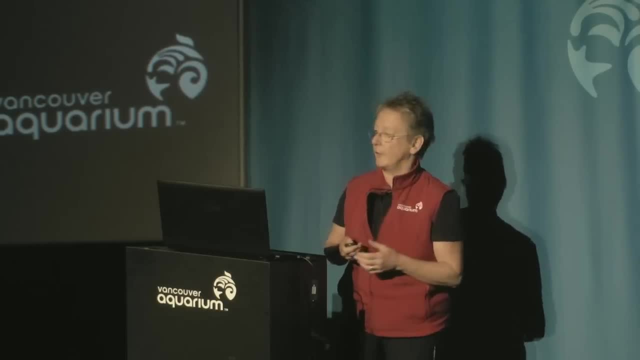 We used to take them for granted. They were everywhere all the time, But now we can go back and look at them, look at them in more detail when they were here, and now that they're gone we have to go back. Another thing is we have an algae that has been in Howe Sound before. 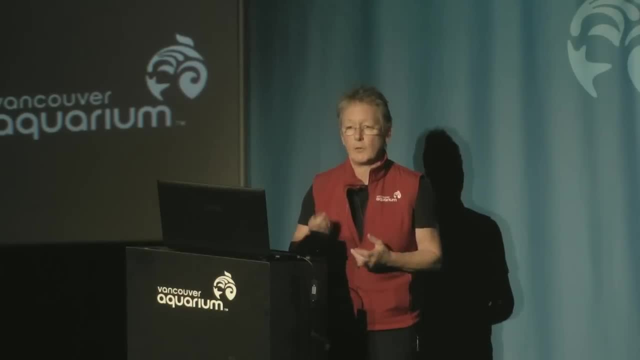 but we're seeing it in greater numbers in different places, and so that's a change, And whenever there's a change, we're really interested in that. So we go back and see what we had before and pay attention to what's happening now. 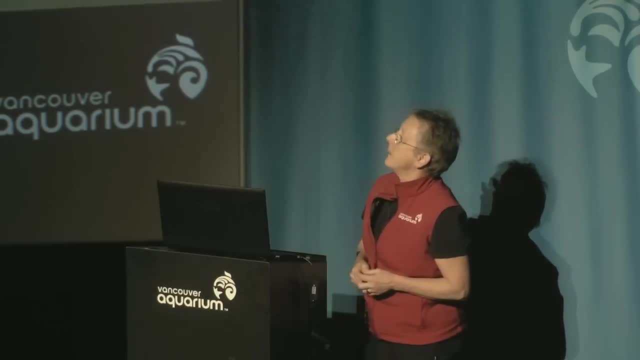 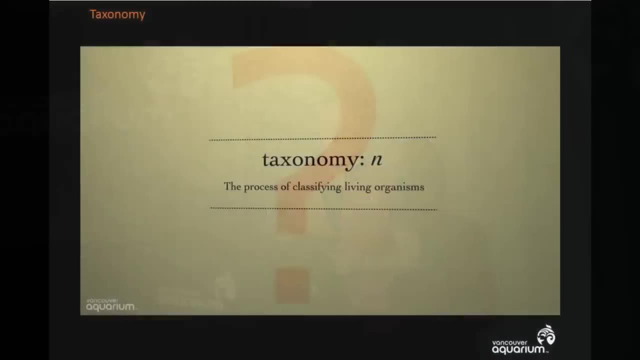 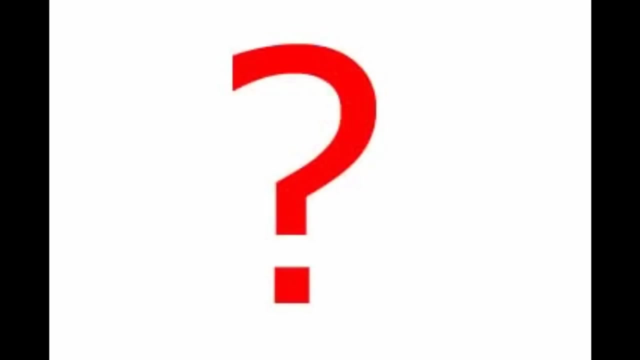 So that's what we do as taxonomists. The process of naming organisms is called taxonomy, And the important thing about taxonomy is it gives us comparison to other animals as well. So the more we know about organisms, the more we can compare them and look at them and see how they interact together. 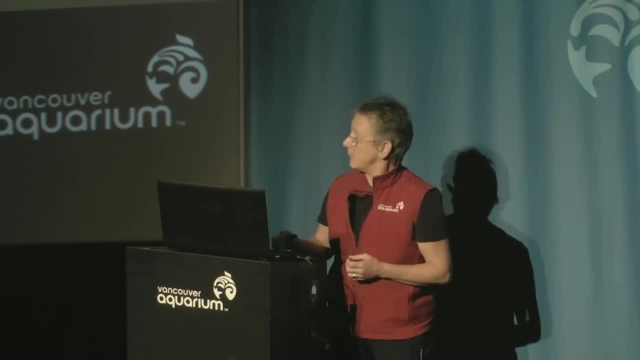 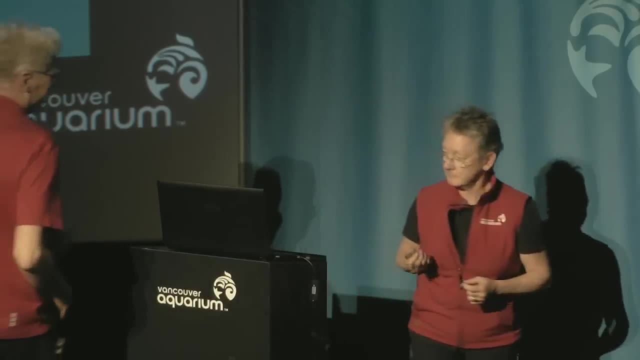 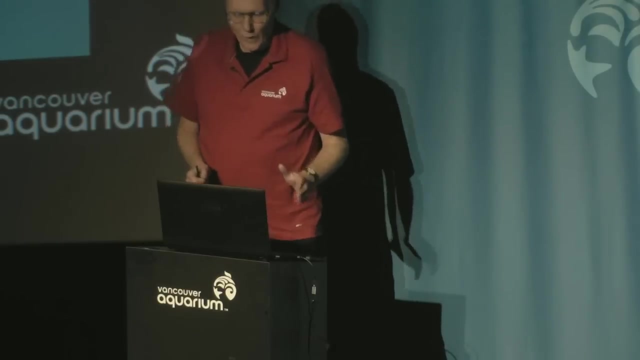 Now we We're going to talk a little bit more about taxonomy. Jeff has some ideas about this and how he wants to speak about it. So I just want to make one point, which has to do with the fact that most of you are familiar. 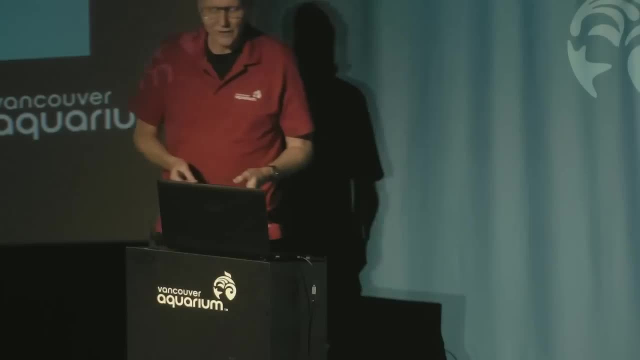 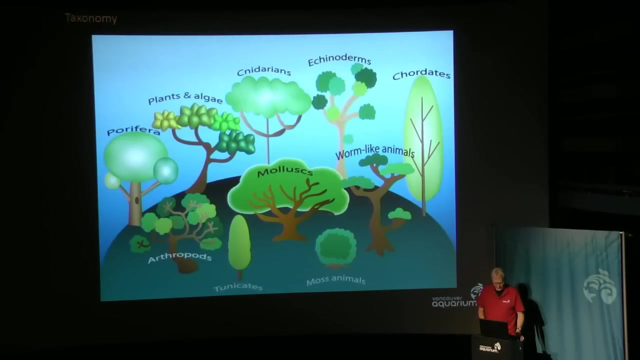 with your family tree, how you're related to your cousins, your aunts and your uncles. You've probably seen a family tree of life, the relationships of different types of plants and animals to each other. I just want to give you a little reminder that all the ideas that get presented to you 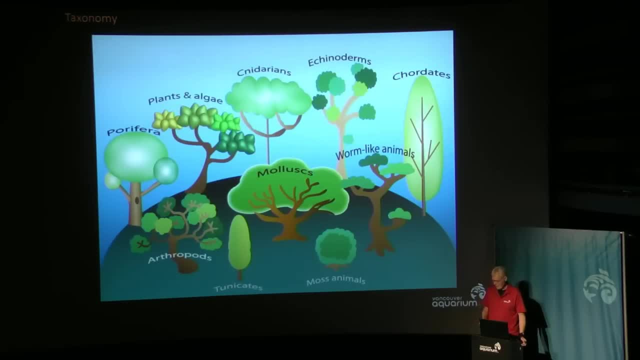 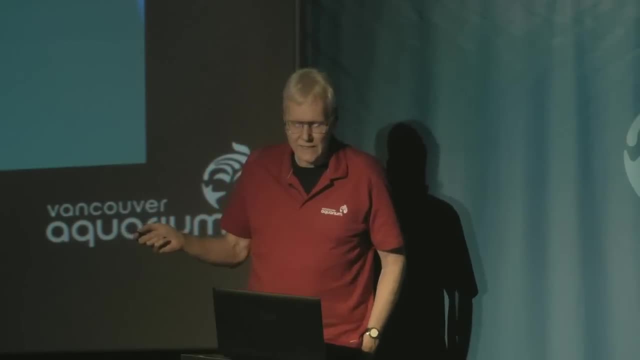 come from human minds, They don't necessarily represent reality. We're showing you a whole grove of family trees because, for example, the arthropods, which include the insects and the crustaceans, are considered on the part of all the scientists. 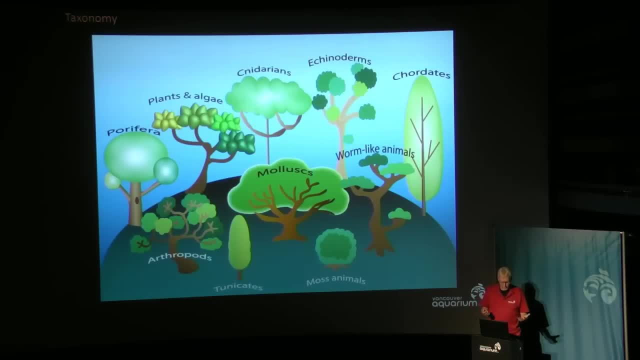 at the British Museum to not be from the same origins. They say that crustaceans are polyphaletic, meaning it's a grove of family trees. They arose separately different points in time and came to the same evolutionary solution to problems in living. 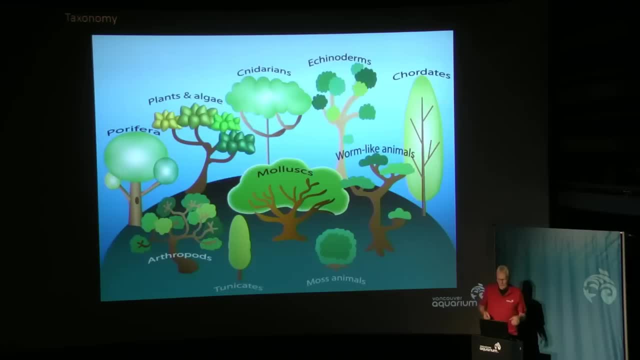 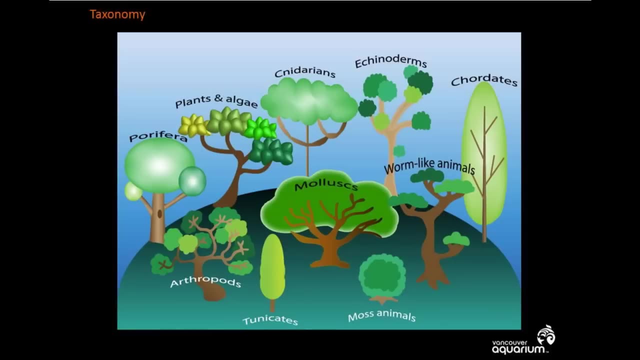 They got to have exoskeletons, similar compound eyes, that sort of thing, And I'm a fish scientist and that nice landscape tree way over on the right Chordates represents animals' backbones. That's the fish. 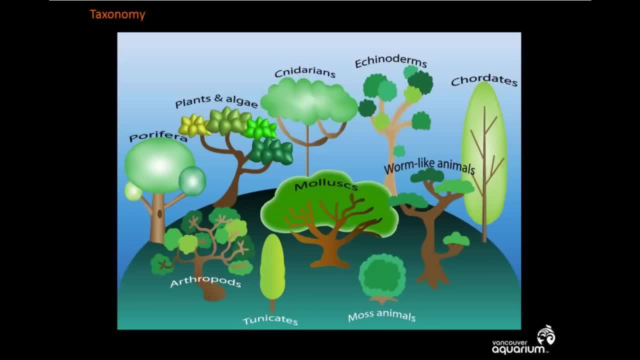 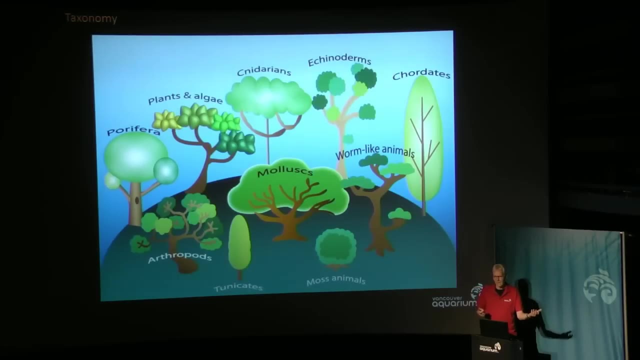 And in fact, my understanding is that, in fact, eels were never related to other types of fish and the lungfishes are not related to our persiform fishes. The perch-like fishes didn't really arise from the soft-raid herrings and salmon. 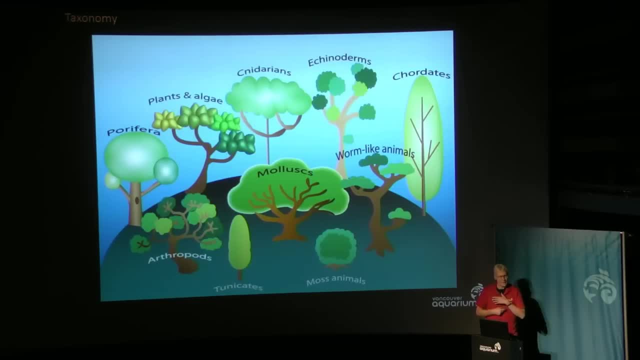 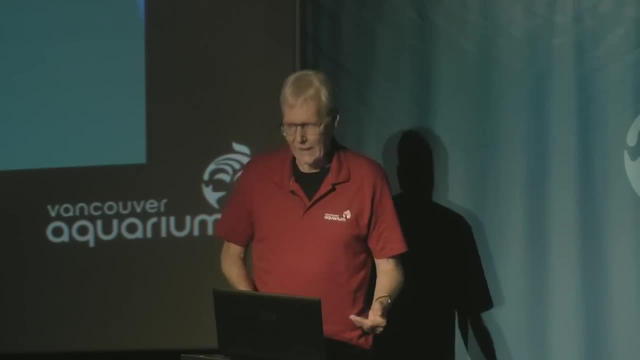 They're unrelated And codfishes are unrelated. Codfishes are an excellent example, because their anatomy is very, very different. Their circulatory anatomy, their skeletal anatomy, they're just very different. They arose from separate ancestors. So fishes are polyphaletic as opposed to monophyletic, which means one family tree. 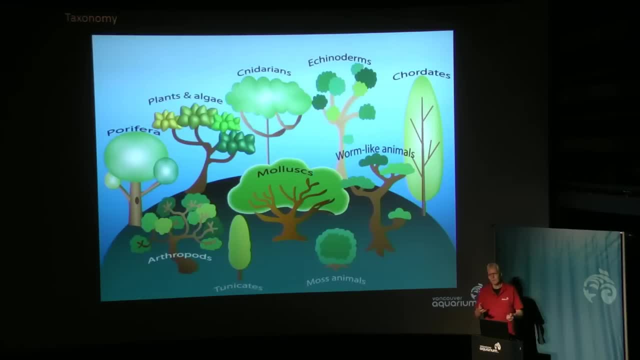 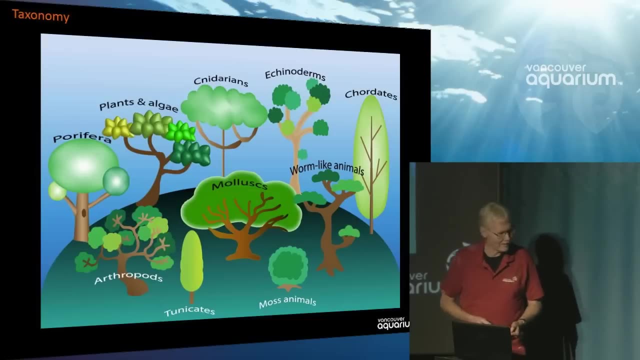 It's just a different point of view and there have been very forceful presentations of arguments that we all arose from the same cell. Got that? It's just difference of opinion, so keep your minds open. okay, Here you are. Thanks, Jeff. 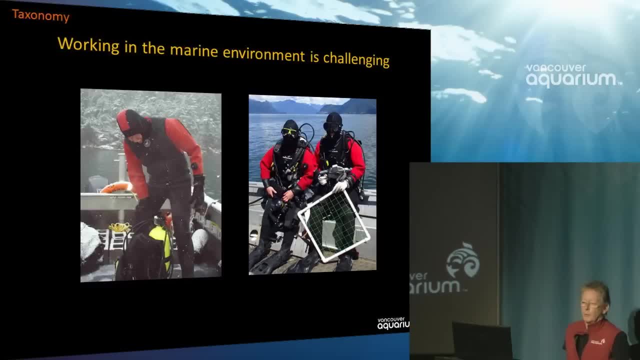 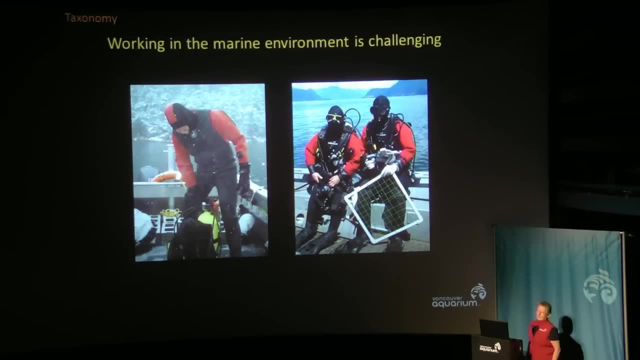 It's not always easy out there. We can't just pick and choose when we dive or we wouldn't have any reliable data. So we're out there in the rain and the snow and we're taking quadrats and cameras and we're just doing everything we can all year round. 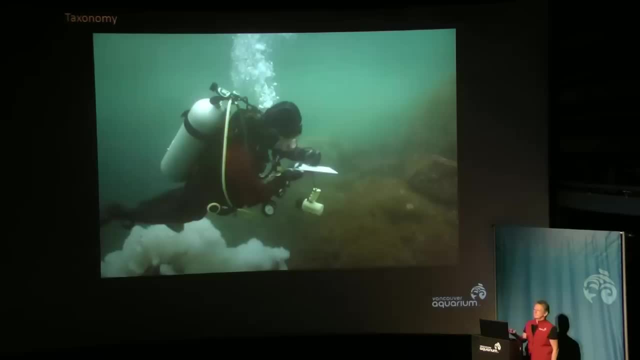 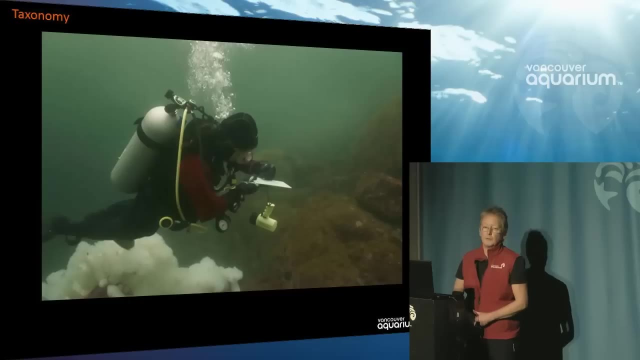 So there's always challenges to working in the marine environment And some days we're really lucky. it's crystal clear to do our work and we can see what we're doing and do multitasking, and this diver is taking taxon notes. 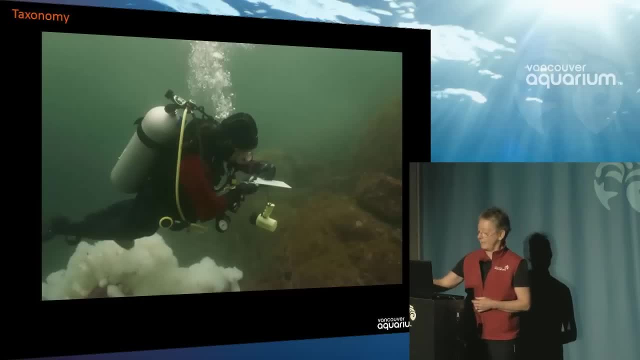 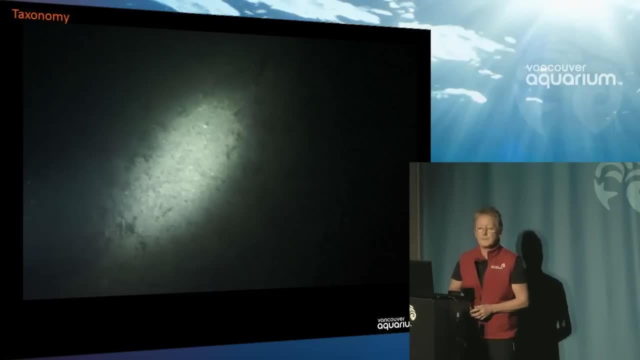 You can see the slate and they're just getting the data they need from the dive. But other days- this is what we're dealing with. On this dive we had 20 minutes to go from the surface down to the bottom, find a biohorm. 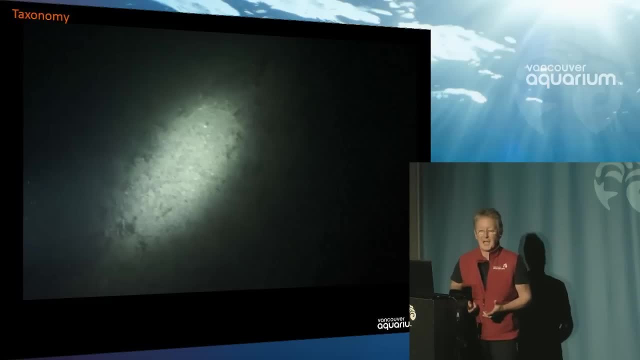 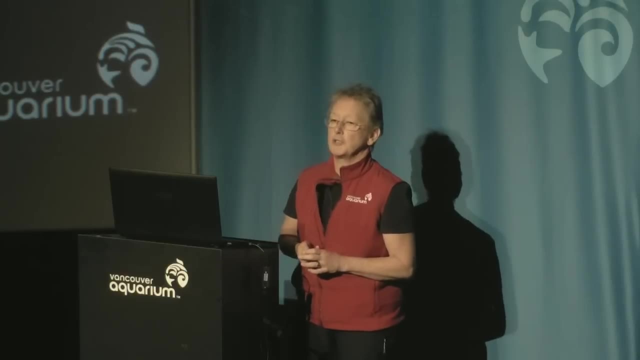 that we'd never seen before. It's a little bit of a needle in a haystack because we throw the anchor. we have a pretty good idea where we are, but until we go down that line and find the bottom and look around, we're really not sure. 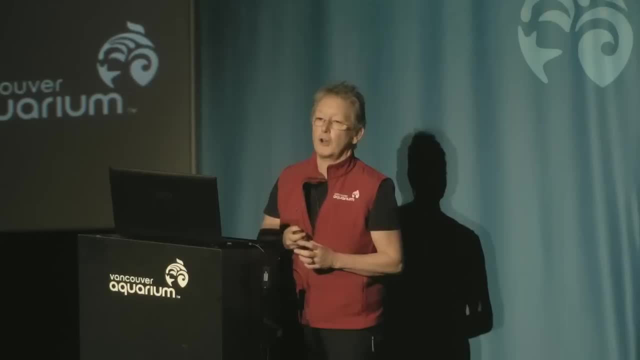 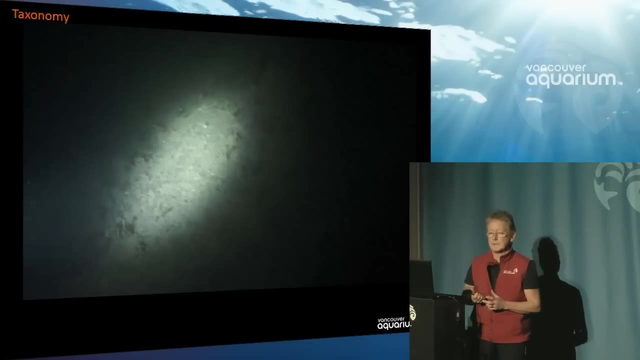 So this is what we land on. sometimes This is about 90 feet in the darkness, And but we make the best of it, because on every dive we do we try to get some kind of taxonomy, even if we're doing other purposes. 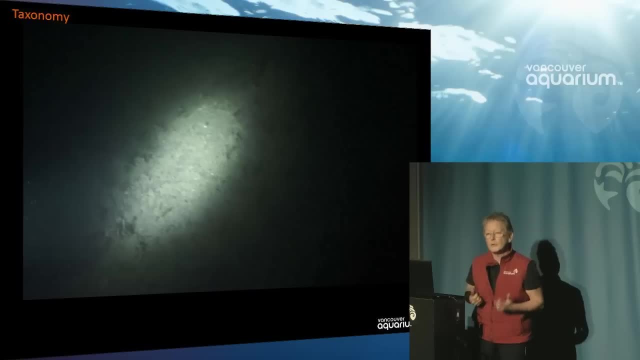 In this case it was actually looking for a biohorm, But because we may only get to this dive in our careers three or four times, we try to gather all the data we can because it may be the only data we get. 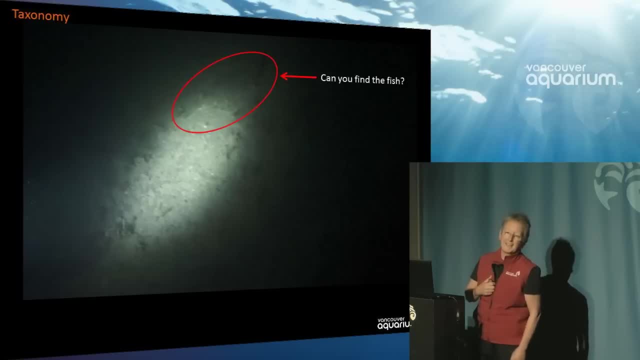 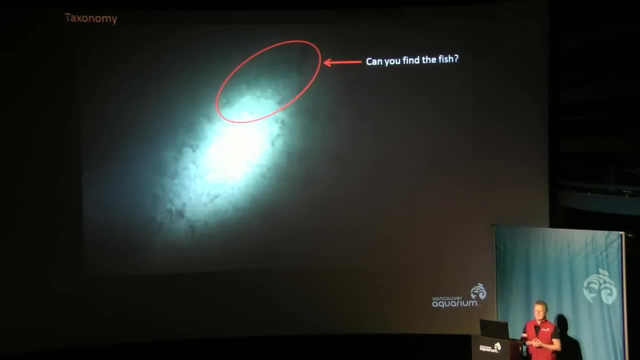 So find the fish. That's the fish that we just recorded on our way by. We saw it and so that goes in the taxonomic database, even though it's not really part of the dive. So 20 minutes surface down and back up to do this, plus Jeff will explain he's going. 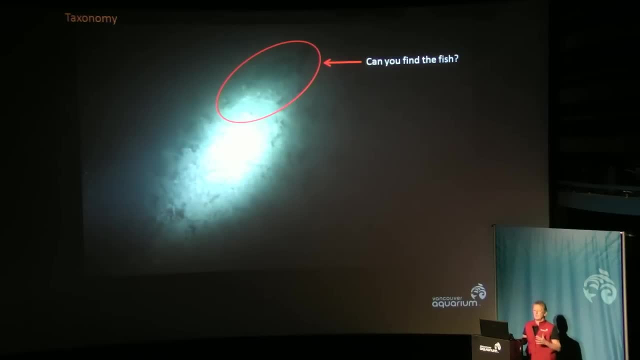 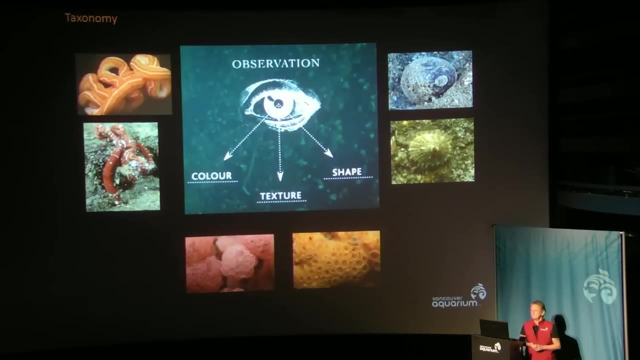 to show you a film of the biohorm that we actually found that day, and so you'll get an idea of what we're doing in 20 minutes. To be a good taxonomist, you have to look for color and texture and shape, and that'll. 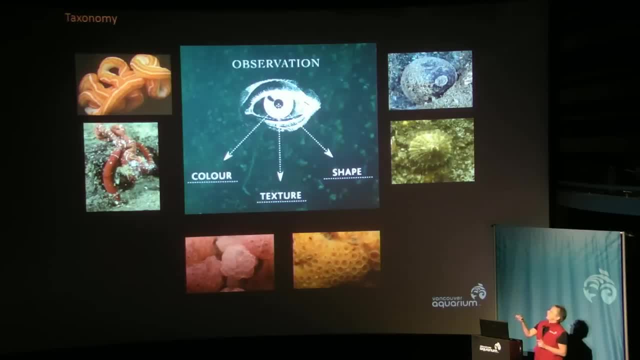 help you identify animals. So up in the top left we have a couple of worms that look a little bit similar, but there are different stripings on them And they're actually different colors, So that's what you'd have to look for in order to identify them. 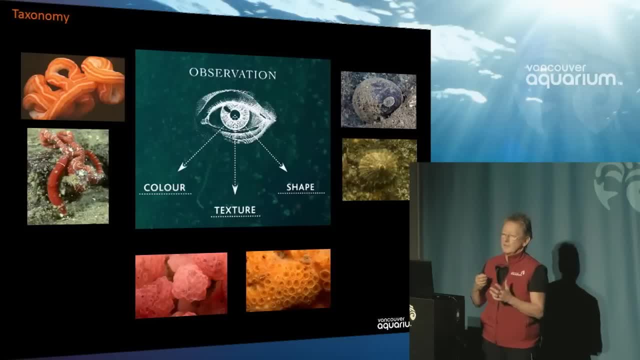 And there wouldn't be another worm that had striping like this. But there's something very similar in a couple of worms. In this case, over here we have two animals. They're limpets and they're about the same depth, but they're very different looking. 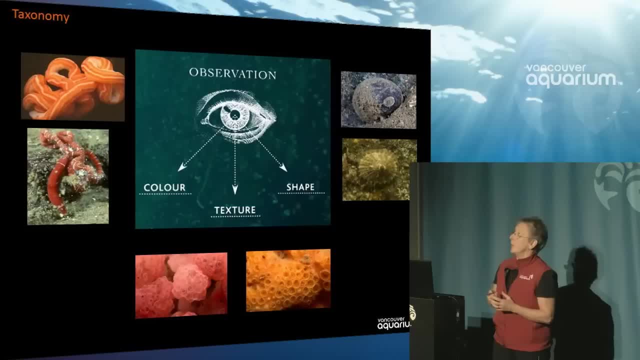 And you just develop an eye for it. So if you can pick up the color and the shape in this little mark on this guy and the ridges on this one, this one has a hole in the top, But if you're just swimming over them, 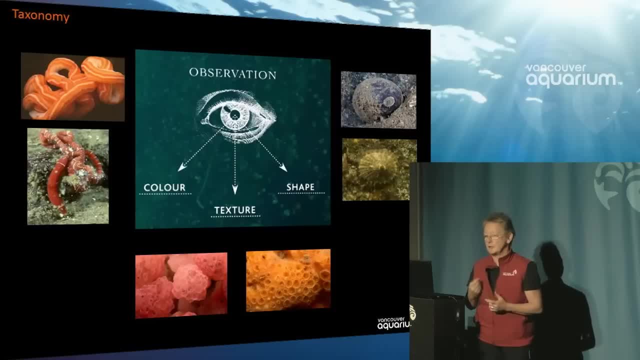 quickly you might not notice those details. So the more details you get to know in your mind, know the animals, you get very good at picking out the different species while you're under water. These animals here look very similar. 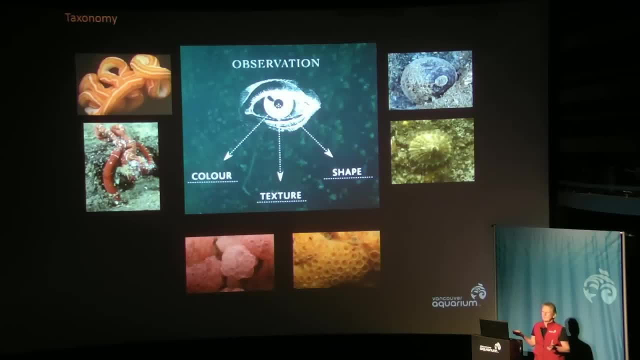 This one is a sponge. This one is a completely different animal and a different phyllo. This is a tunicate, This is a mushroom tunicate, And so the textures are very similar, but the animals are very different. So the more you learn, the more you'll do well with taxonomy. 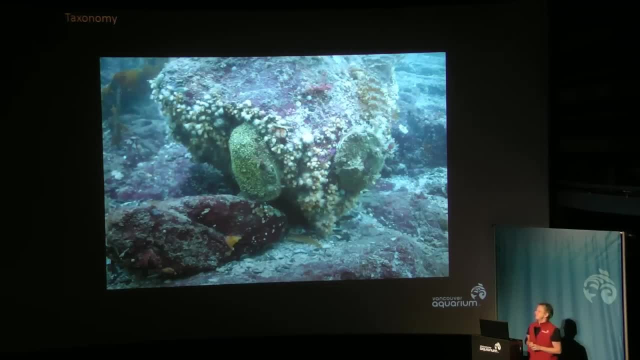 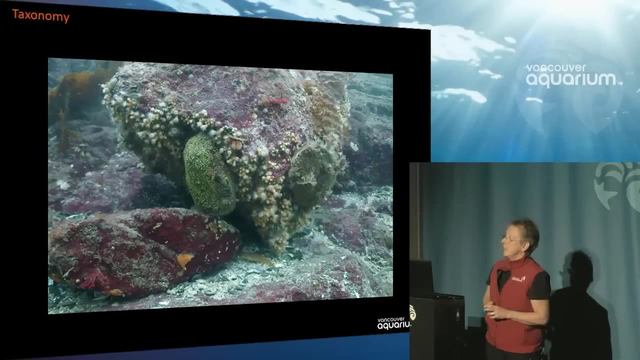 find the species. this is a rock with quite a few species on it and in a lot of different phyla, and this is what we do in a taxon dive. we don't have time. we meant this is about five minutes of a 40 minute dive because we're at shallower. 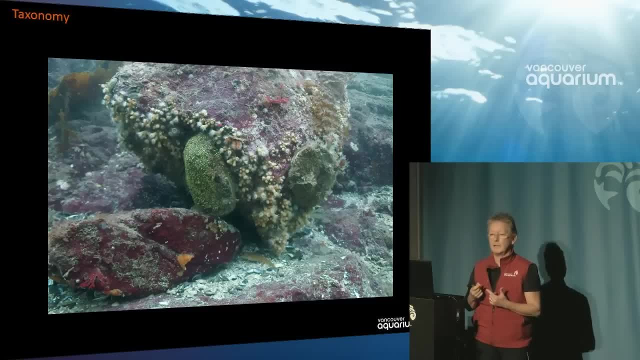 depths this time, but we have to, as we're swimming along, just calculate the abundance and the number of species in and we record it later. so in this one in particular, there are 17 species in eight different groups. so we've got cnidarians, these are zoanthids. we have not gonna go through them all, but I'll. 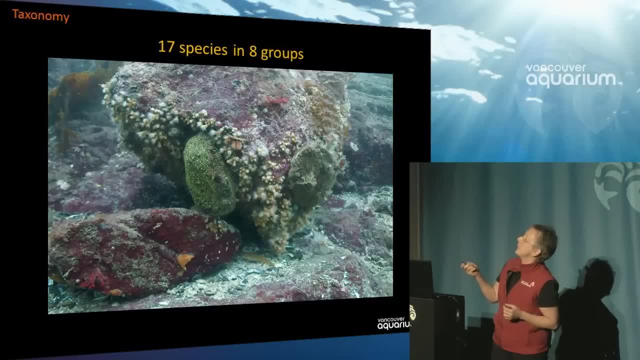 show you. these are rock scallops here, and on the rock scallops there are sponges growing in the, in the shell. we've got a fish here, a goby we've got, encrusting red, algae's we've got encrusting coral and algae's we've got. 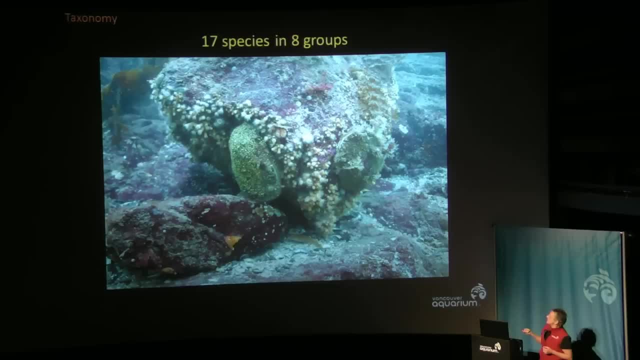 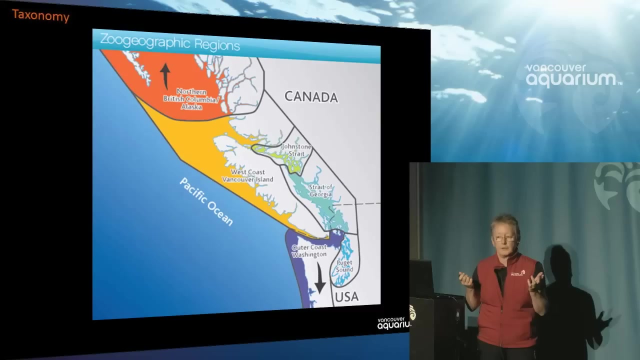 other varieties of red algae sponges. that's the sponge we just looked at and you can see the red algae. that's the red algae. that's the red algae. that's the red algae. it looks a lot different from what it was when we knew there were some sort of 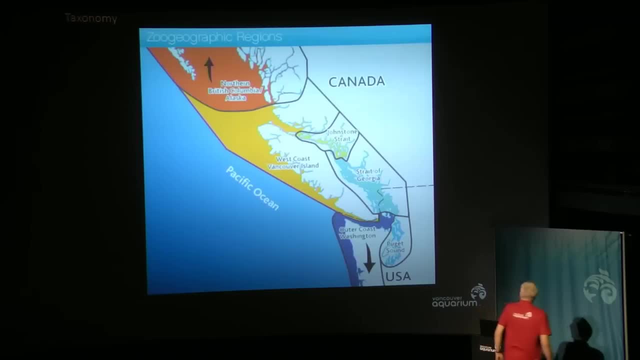 fungus growing in each of the soft expand the water. does the scion oil? heard this popular concept of the Salish Sea, Puget Sound in the Strait of Georgia. It makes good sense from a socioeconomic standpoint. There are a lot of cultural reasons to talk. 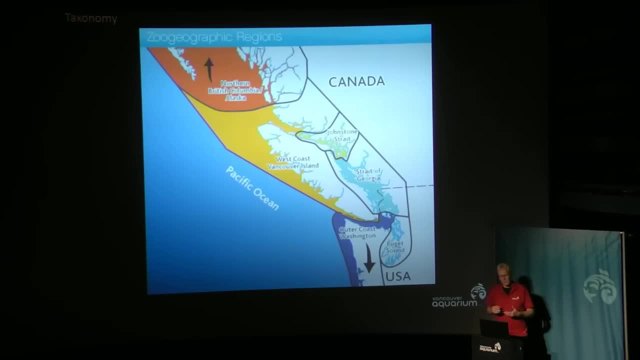 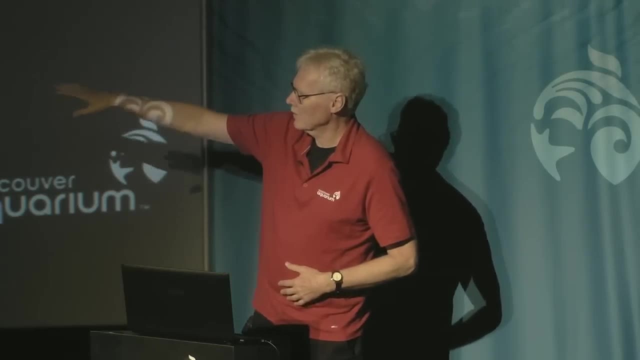 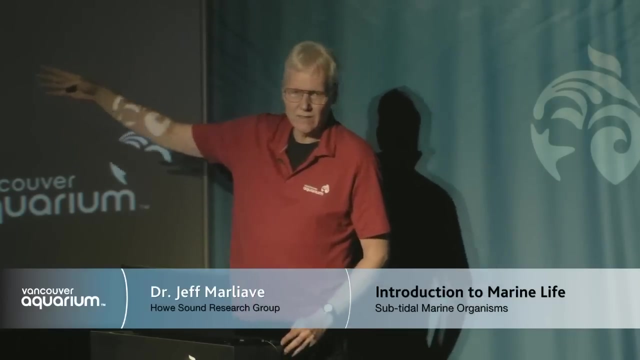 that way. But when looking at nearly half a century of seabed biodiversity data, natural groups fall out And the purple color shows coast of Washington, Oregon outer coast fully exposed to open ocean weather, And the animals on that part of the American coast are quite different from up in northern British Columbia and Alaska, where the water's quite a bit colder. You just have different group of species And the west coast of Vancouver Island is somewhere in between. Now, coming around Johnston Strait at the north end of the Strait, 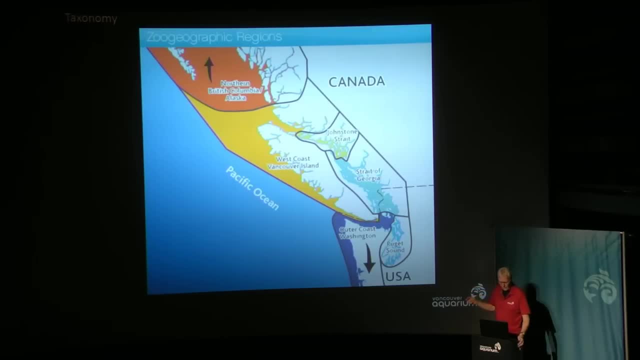 of Georgia has terrific tidal currents but no exposure really to wave action and heavy storms And that's characterized by a unique set of species, lots of interesting seaweeds and such different from the community in the Strait of Georgia. Notice that this outer coast community in the Strait of Juan de Fuca goes all the way. 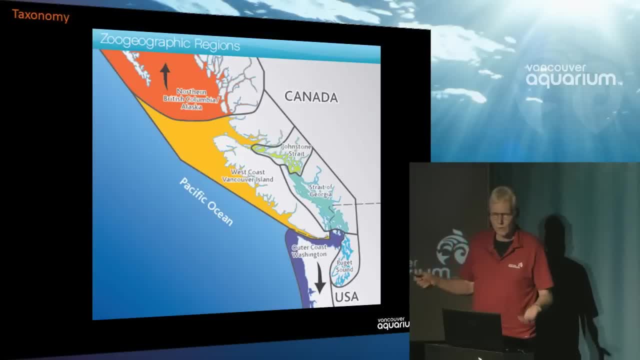 to Whidbey Island and the southern coast of San Juan Island, So you have totally open coast animals like purple sea urchins, surf grass right in this area And the species are so much an outer coast community that they act as a buffer, a big barrier between 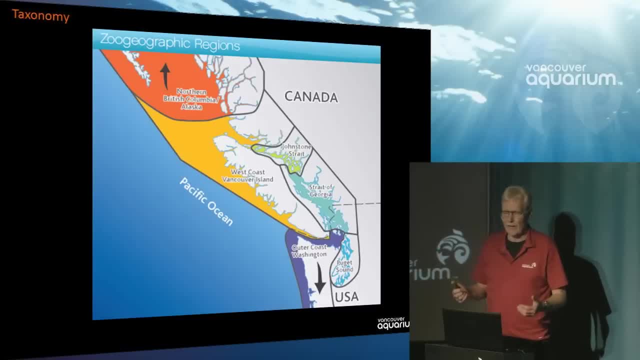 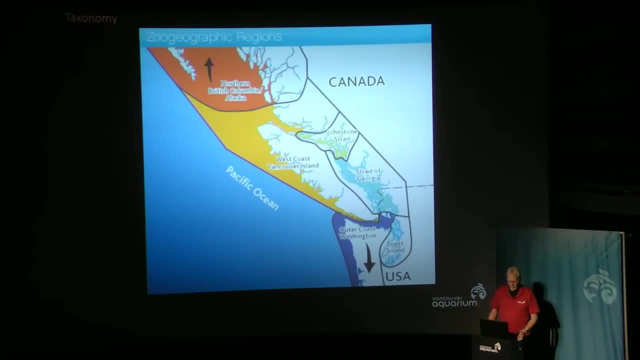 the Strait of Georgia community and Puget Sound. So Puget Sound in fact has a very special species diversity that's quite different from the Strait of Georgia. They're not the same, and this depiction of zoogeographic zones kind of blows the Salish Sea idea out of the 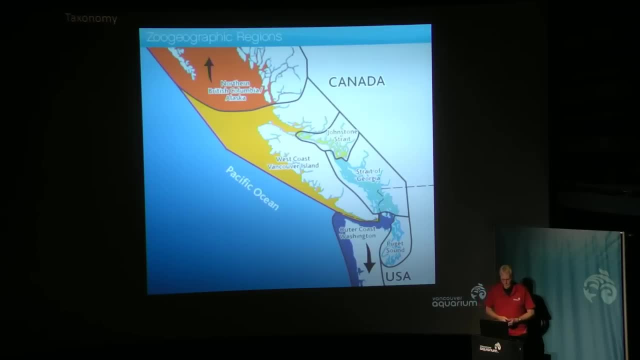 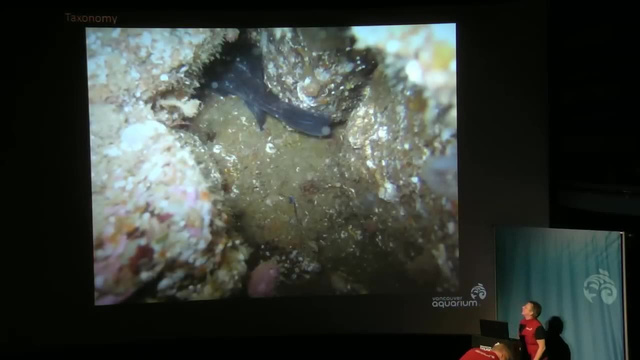 water as far as seabed biodiversity. So Donna's going to continue, And another reason it might matter is being able to identify animals can really help scientists, And it's a very important thing for them to do to help them keep their behavior and 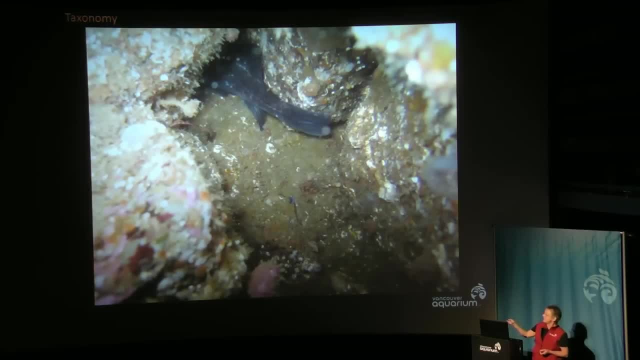 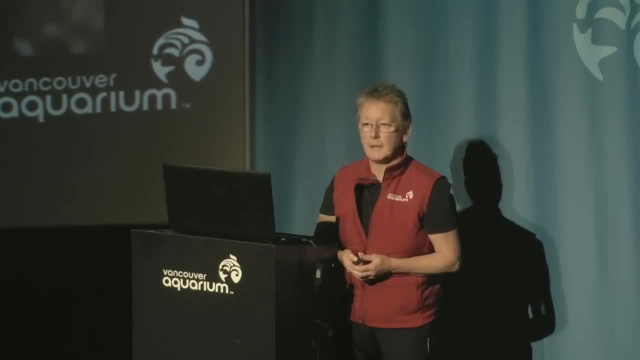 this is a picture of a fish that was seen at White Cliff Park. You can't always see the whole animal. This is the fish here. There's a tail in the back end, Just a little bit of the body. It's a black rock fish And this is a very important animal because of the 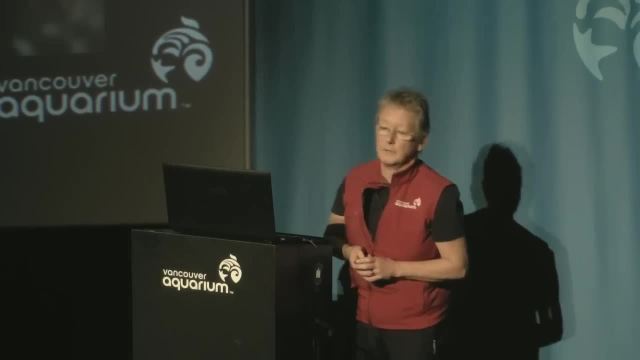 releases that were done at Point Atkinson. this shows that the animals had actually reproduced and traveled as far as the White Cliff area. So knowing that and being able to help with any identification or animal movements it's is really good for science as well. 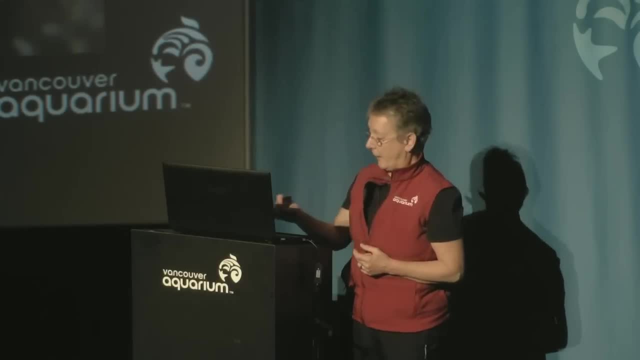 So anything any diver can do for that is really great. So if you're a diver, and beware, because citizen science will get you. It's a lot of fun. You get in the water. You start to learn taxonomy just because it's interesting. 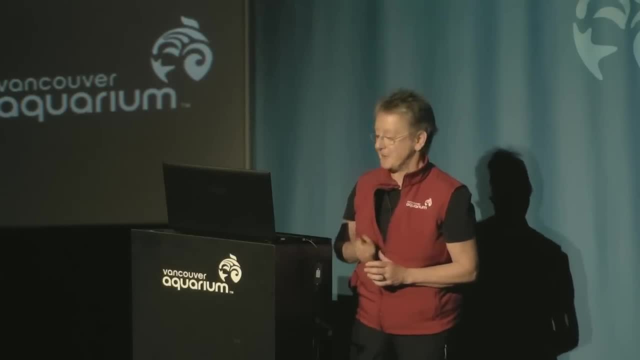 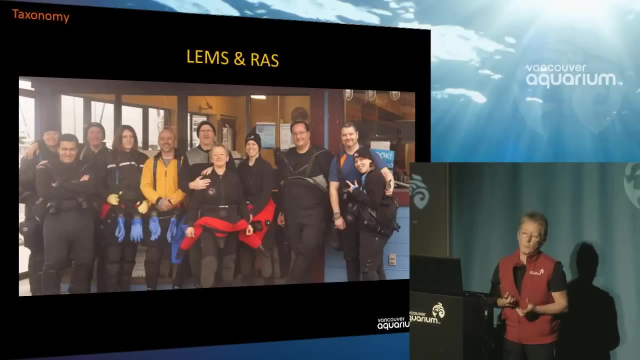 And scuba snacks help you get started, because there's lots of different shapes and sizes in there to give you an idea. So you usually start by just diving on your own and seeing things and then you want to know more. So you get out the guidebooks and you come to people like us. 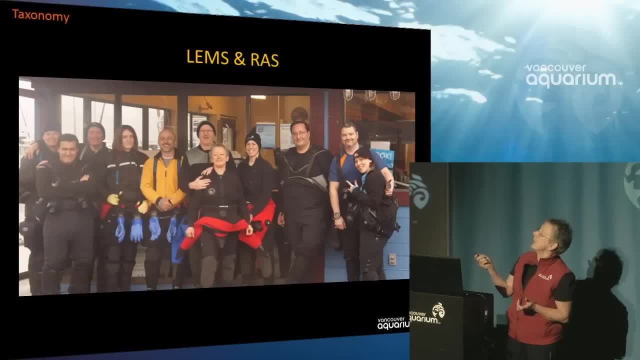 who are doing a lot of taxonomy as professionals- and we have our protege here, Laura- And then all the people around are a group of divers who were really good to us this year and every year they help us with the Lingcod Egg Mass Survey. 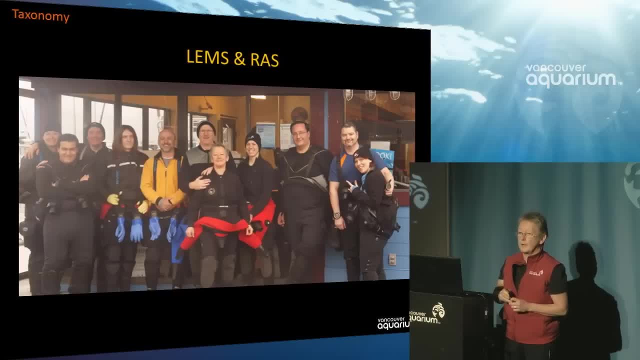 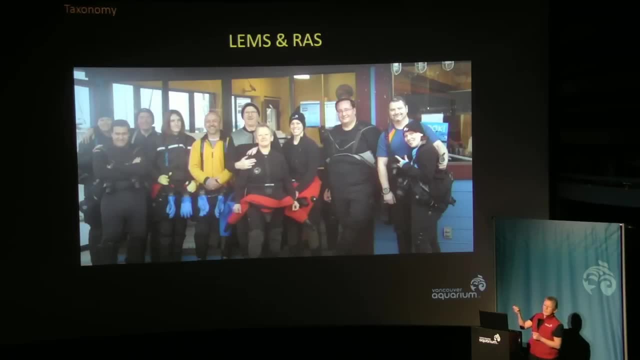 which is a survey that we do every year to try and help us understand their reproduction and their egg sizes and how they're changing out there. And also we have Rockfish Abundance Surveys running this time of year, and the divers are helping us do that too. 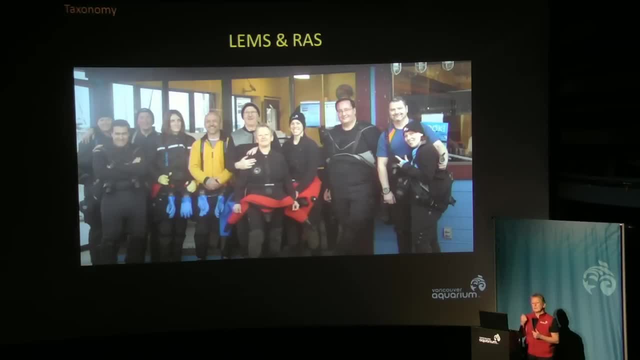 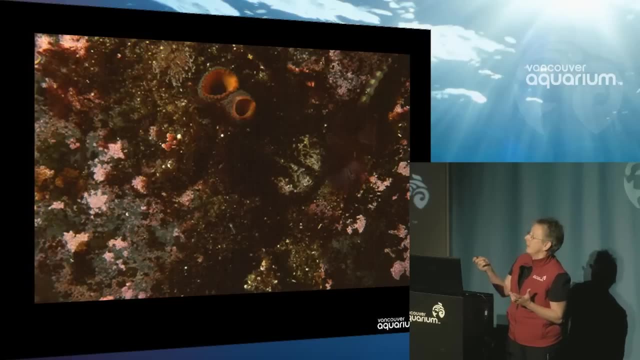 So the more these divers can learn about the animals associated with these species, it's really helpful as well. So first you learn to look in little cracks and look for animals like this that live in a crack. It's a clam kind of thing. 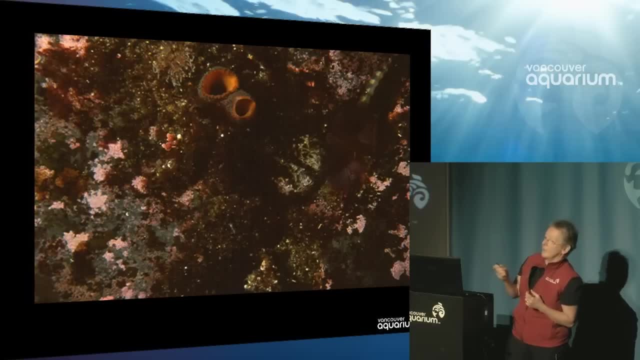 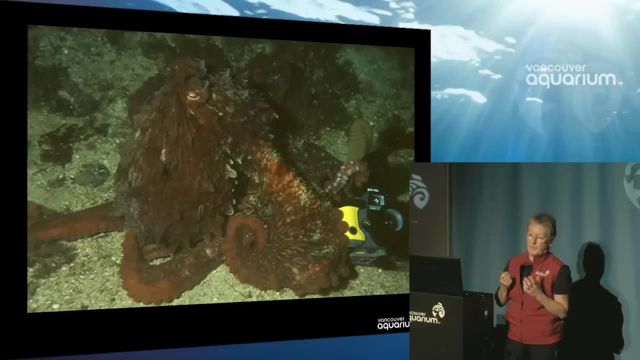 And there's some worms over here. You can barely see them, So you've got to get your light in there and you've got to get curious about what's happening. But if you're lucky, the animals will come to you as well. 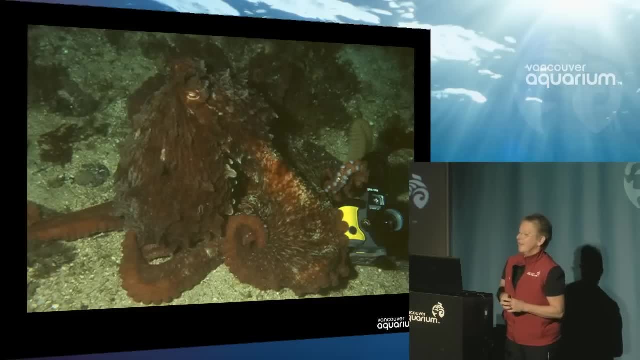 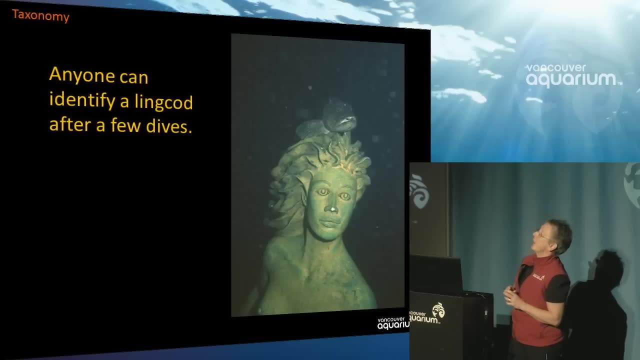 So an octopus might stay. They'll sneak up on you while you get your head in that crack and just you turn around and there it is. So they're curious, So you've got to look up and look around, sometimes as well as looking in the cracks. 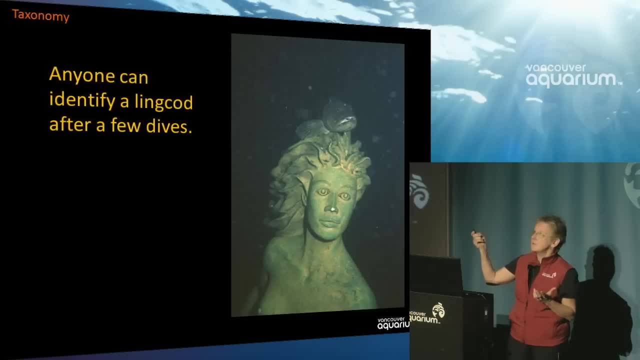 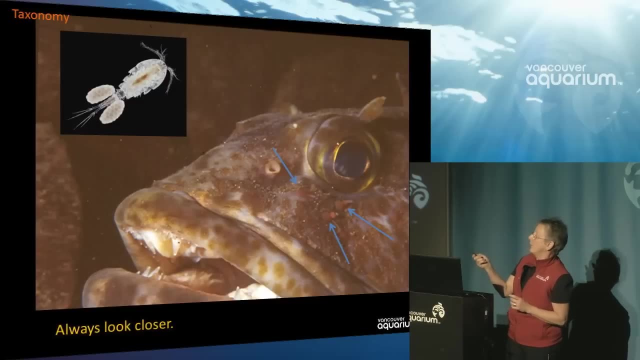 Now anyone can identify a Lingcod after a few dives because they're big, obvious fish. But the serious people will want to know what are these things on the fish as well. So you'll see more. So you always want to look closer. 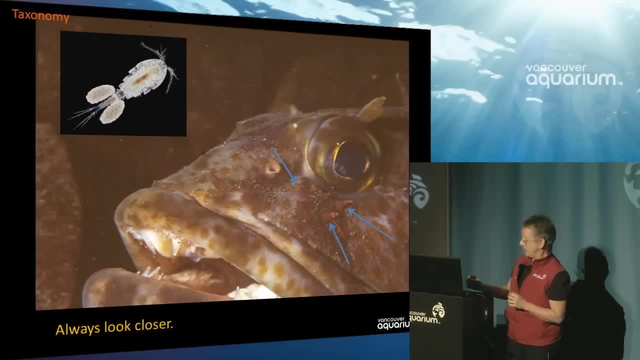 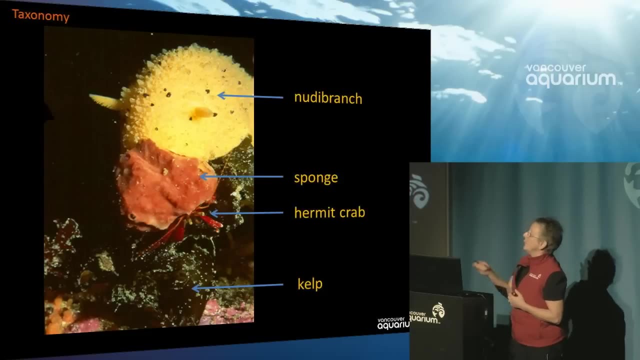 These are copepods. There's a close-up of what they look like, And then you'll see a parasite on the fish, And then we have associations, And that's another way to learn taxonomy. is we here? we have a sponge which has settled on the shell. 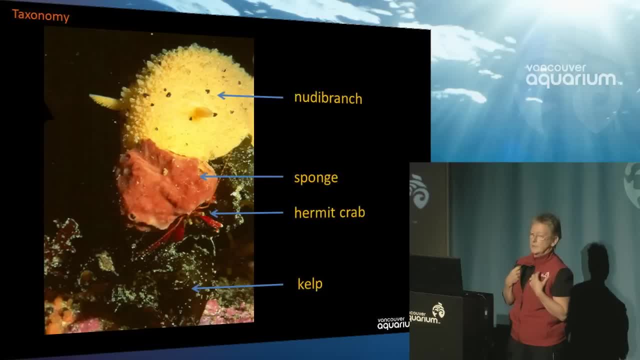 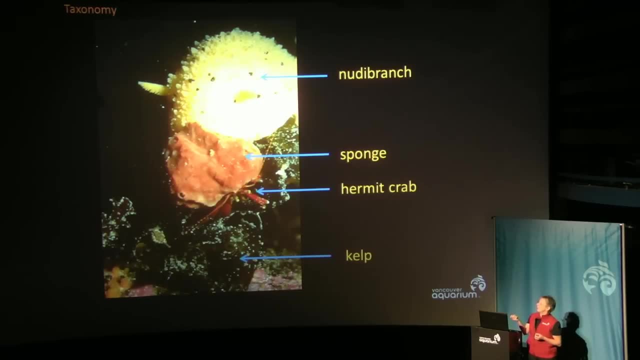 of a hermit crab and dissolved it. The hermit crab is fine, It doesn't hurt its exoskeleton, which is its outer coating. The hermit crab and sponge live together, And then the hermit crab is busy eating a little bit. 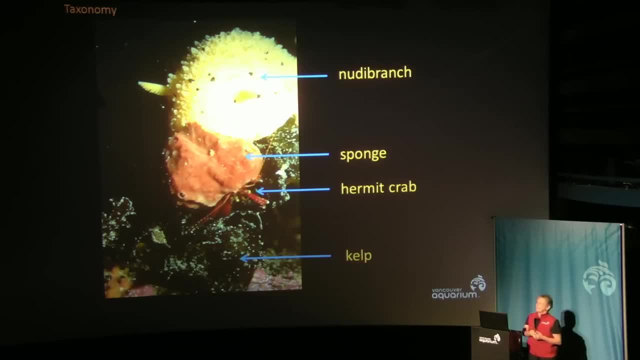 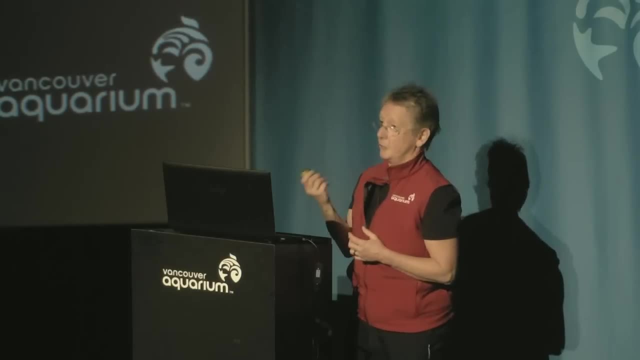 of stuff on the kelp And in the meantime the nudibranch has decided that the sponge is a really good snack because they really like to eat it. So clearly the hermit crab has stopped long enough to let the nudibranch eat. 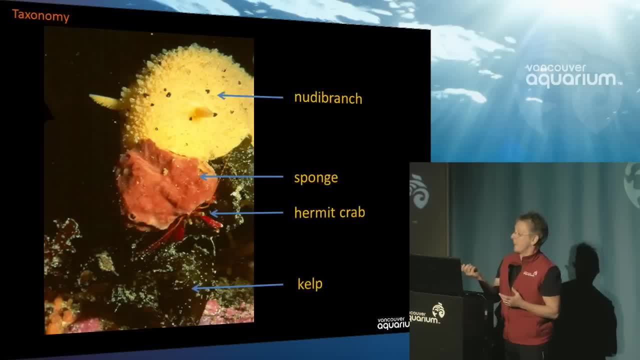 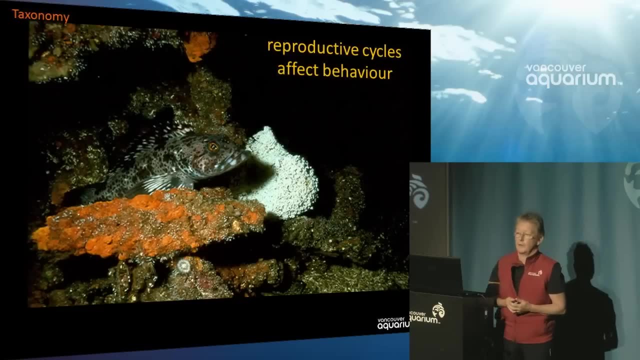 But it won't last for long. But if you know these associations you might figure out what's happening And it helps you to look further for what might be there. Animal behavior is another part of taxonomy. It affects behavior reproduction. There's a lingcod that we're. I was talking. 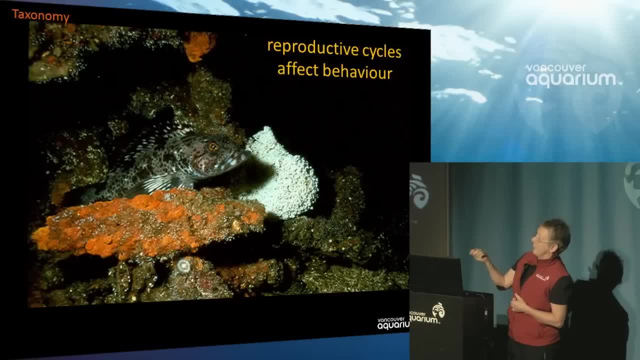 about with the lingcod egg mass survey. There's going to be more talk about that, But the lingcod will stay with its eggs, so you can be sure to find them staying in their territory at certain months of the years. Animal location is really important. 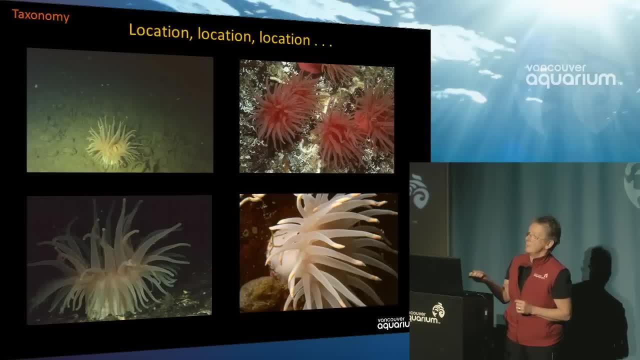 These, this animal, this animal and this animal are all the same And in some locations they look very different to each other. This these ones are: they like, they're grouped and they're dark, pink and they're on walls. 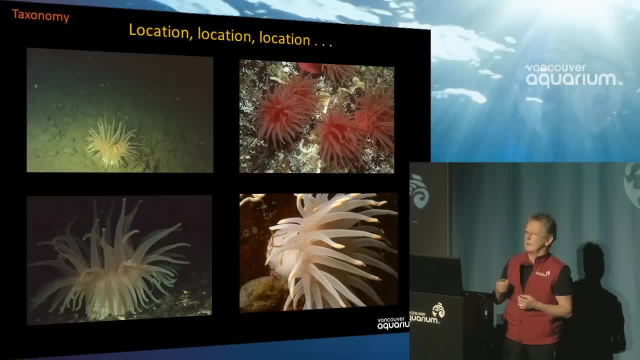 And in Howe Sound. they're singular animals out in the mud. They don't. you wouldn't think they were the same, but they are. But this one here looks similar. It's different. It has, if you could see close-ups of the detail. 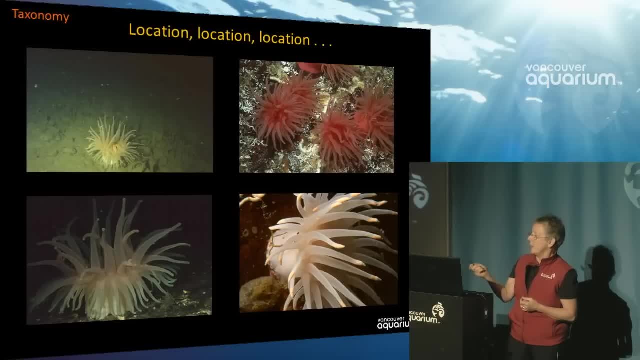 on these tentacles. this one has some marks that this one does not, And you have to be careful not to just quickly identify that as one of these, And that's how you lead to new species. This animal was found in Agamemnon Channel about 80 feet. 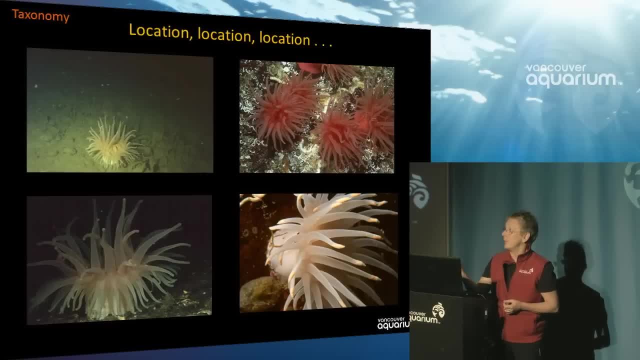 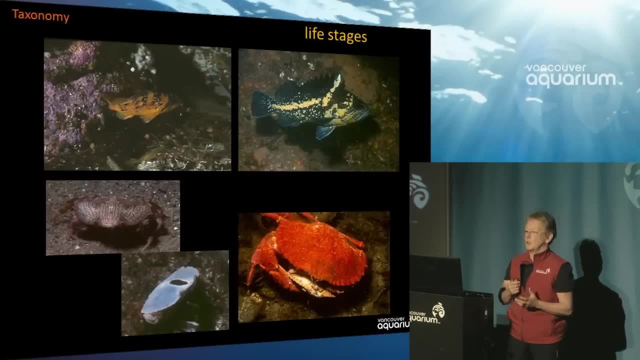 about 10 years ago and we still don't know what it is. But these ones here are all really common and they're all the same. Another way to learn identification of animals is to learn about their life stages. Some of them look very different from the adult. 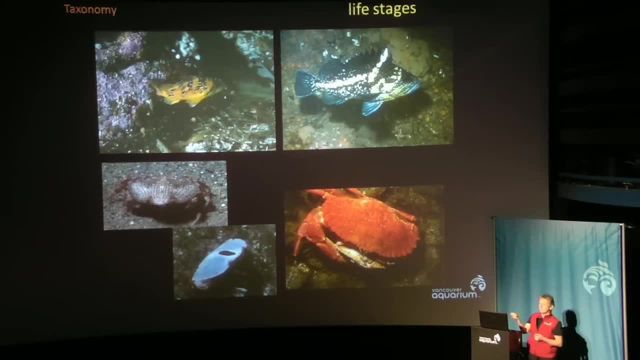 So this one will grow up to be a China rockfish, is a China rockfish, but will grow up to look like this. This is the adult stage And these two baby crabs will are red rock crabs And they have different, different colorings. 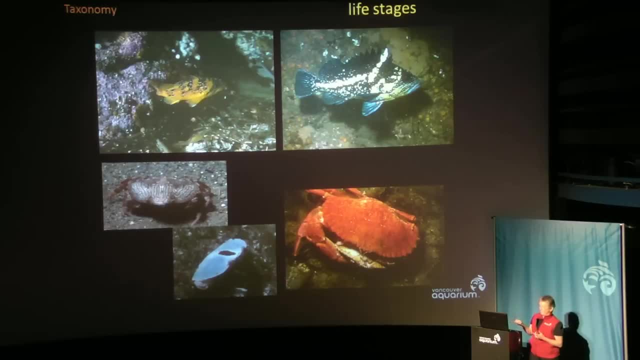 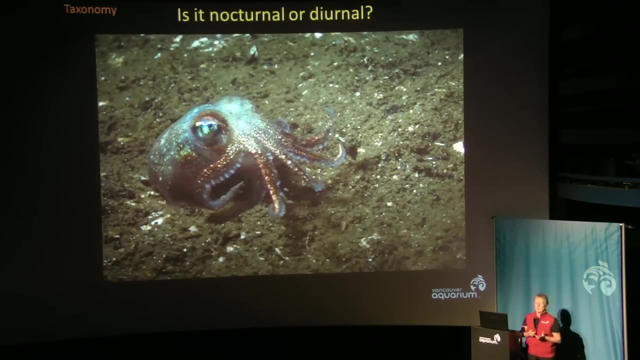 This, this. they're not the same. they're the same animal with different colors, But they will all be this in the end. Is it nocturnal or diurnal? It's hard, It's. it's it's If animals are out at night, sometimes they're. they're really, are just nocturnal. 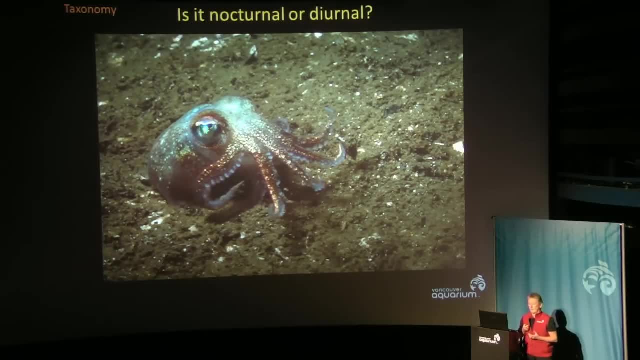 So you won't see them in the daytime. So you have to dive at all times of the night and day as well to to get to learn all the animals. It doesn't mean you won't see them in the in the daytime. 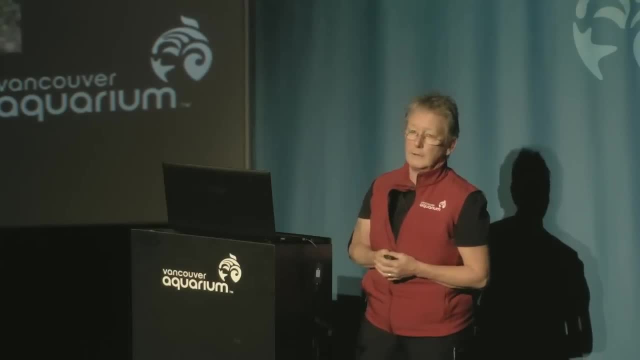 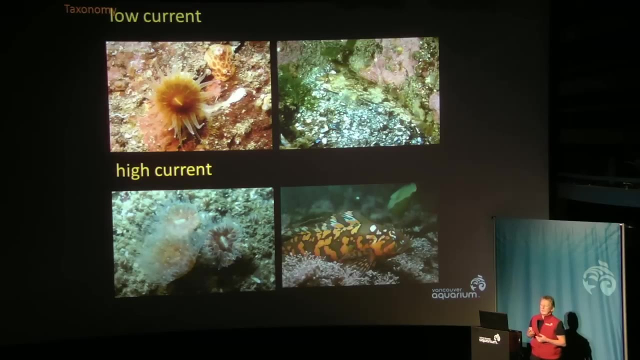 but they're mostly out at night Current Around. here we have the advantage of a lot of areas of the Haosan which are lower current than the outer coast, So we get distinctive animals in lower current areas, And so if you 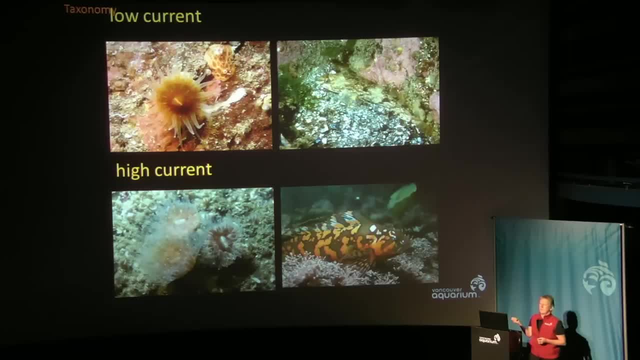 You, you can tell that this animal here is absolutely high current and you would never see it in Haosan. And then, if you did, you need to tell somebody because it's a really big deal. It shouldn't be there. 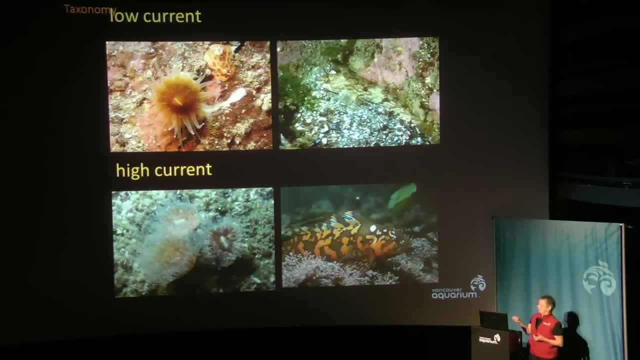 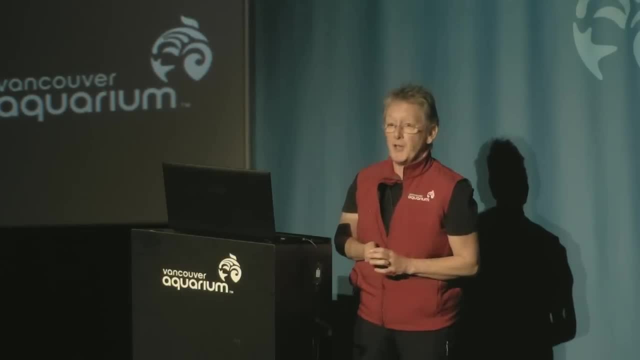 Something's changing and again. So high current and low current will help you learn identification as well. So keep good track of your taxon and get back to me on it, because I'm really curious if you have some lists for me. 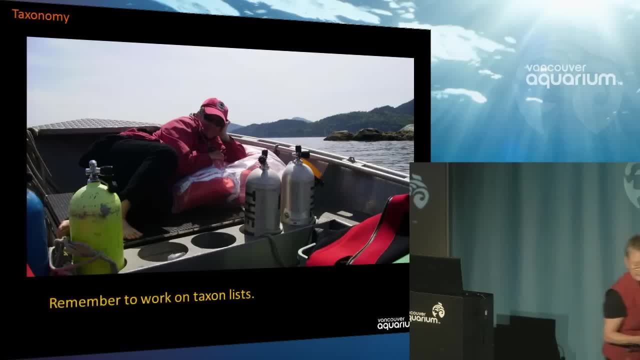 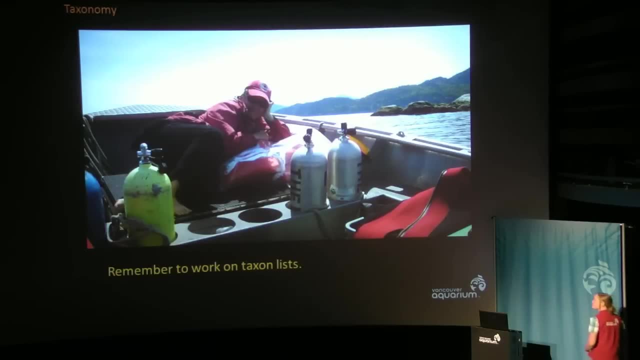 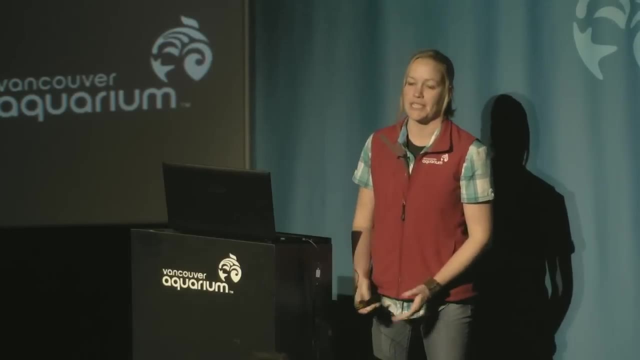 and I can add to my database. Thank you, Hello. so I'm Jessica, as Jeff mentioned, and I'm going to talk a little bit about marine ecology, particularly in Haosan, here. So, as you know, the ocean is an absolutely fantastic place. 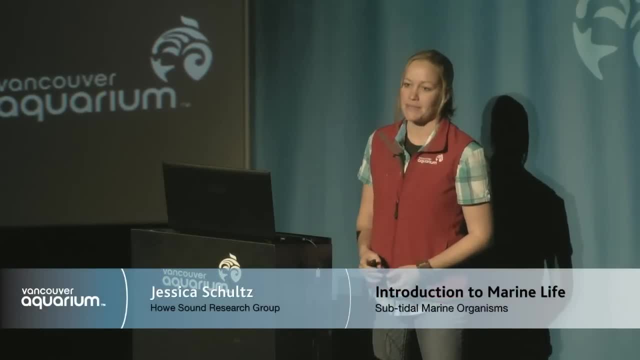 and it's got a lot of unexplored living space within it. Most of the living space on Earth is, in fact, in the ocean, but we know very little about about the ocean. So, whereas on land- and you can spend a lot where you- 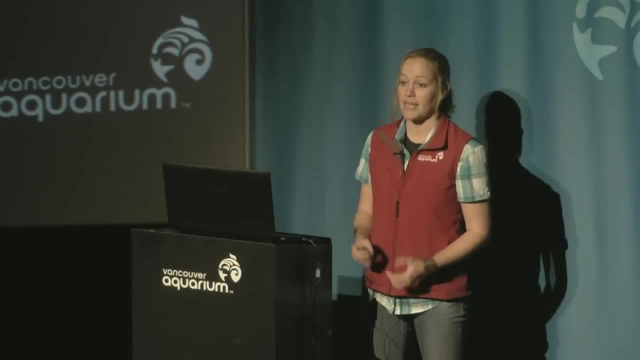 whereas on land, where you can spend a lot of time investigating animals and looking at different habitats, in the marine realm it's more difficult to explore because we're relying on technology and on the limited amount of bottom time that you have as a diver to look at different things. 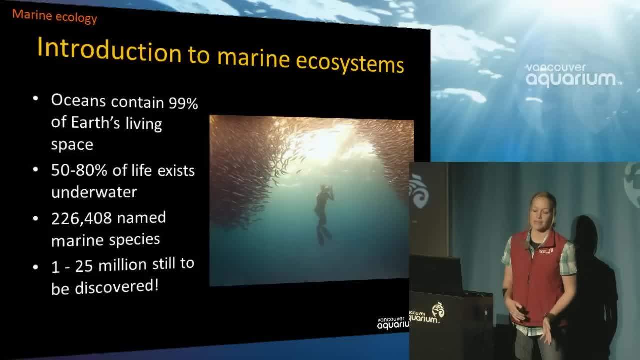 So one of the most diverse species groups of species on the planet is the insects. There's over 350,000 species of beetles alone. So if you compare that to the marine realm, where there's only about 250,000 of all different types of species known, 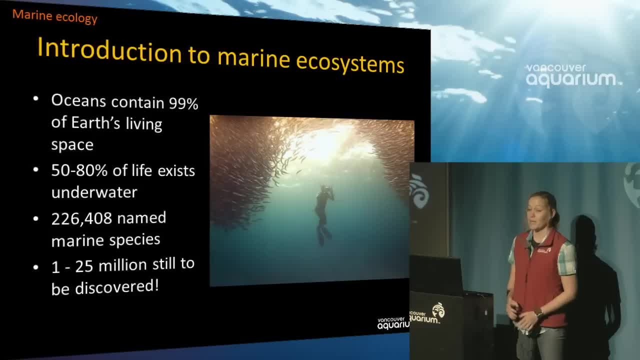 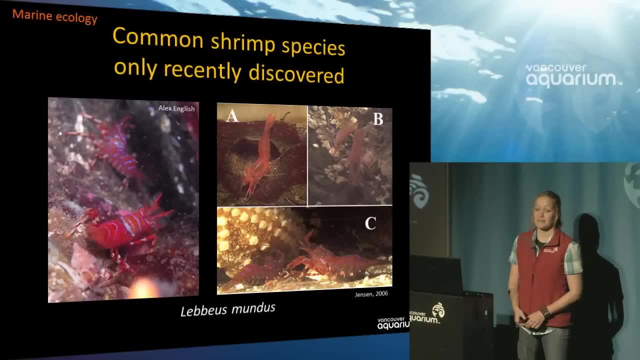 it tells us that there really is a whole lot to learn about the ocean. But you don't have to go down to the bottom of the Challenger deep in order to discover new species, For example this shrimp here called a Libius mundus. 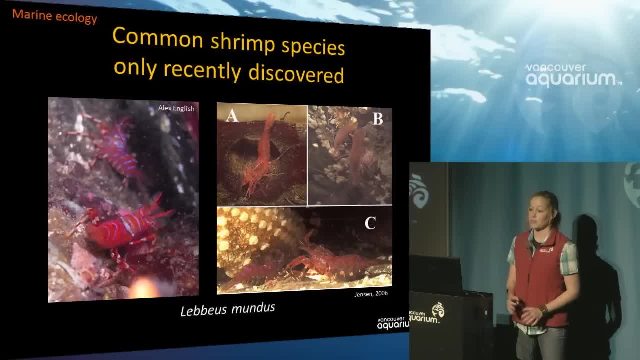 was only very recently discovered- about 15 years ago- And what's remarkable is that it's actually not that rare. You see it quite frequently. It lives in about 60 feet of water, so it's not particularly unaccessible to divers. 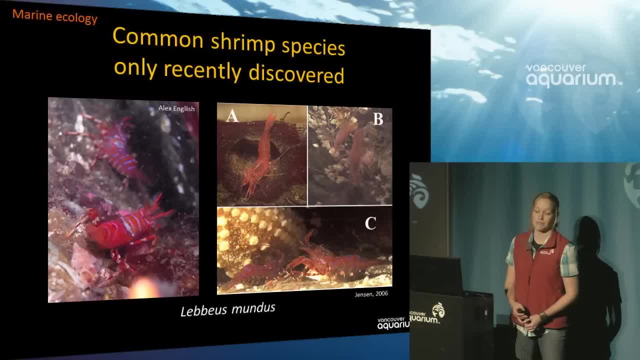 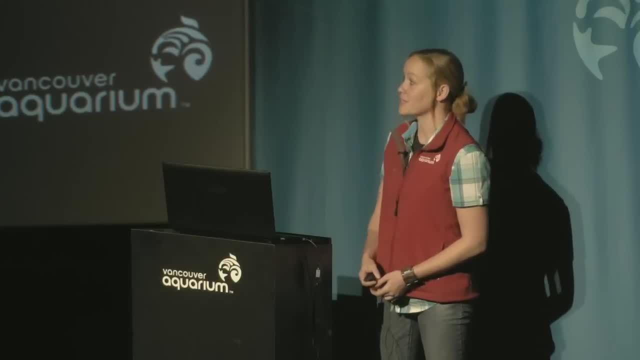 But it can be easily confused with a lot of shrimps that you see more commonly. So unless you know really what you're looking for and the details of taxonomy, you might swim by and miss something like this. Now our celebrity taxonomist, Donna Gibbs, actually helped discover. 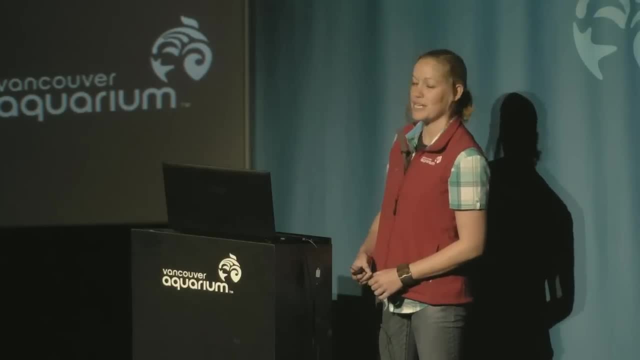 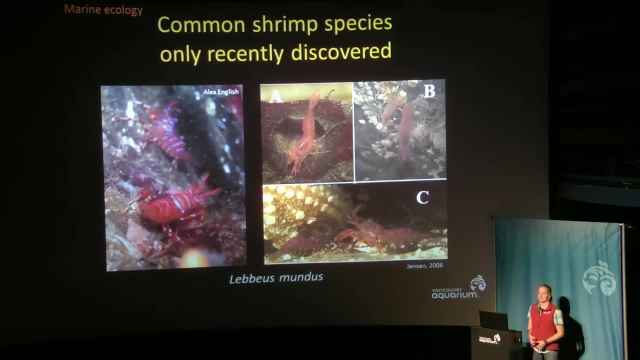 and collect the first specimen of this animal, And so her cat Mundi is actually named after it, because Libius mundus means elegant, cleaner, And, as you know, cats like to bask in their glory as they clean themselves. So there's a fun anecdote there. 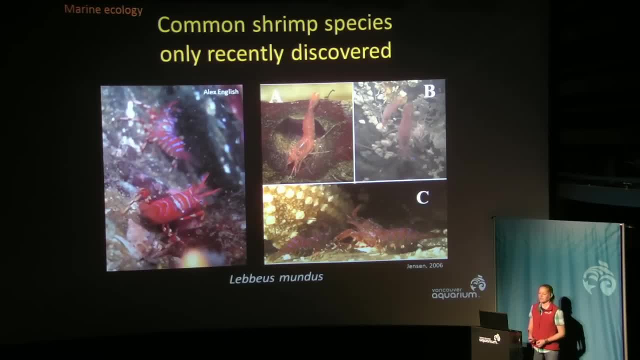 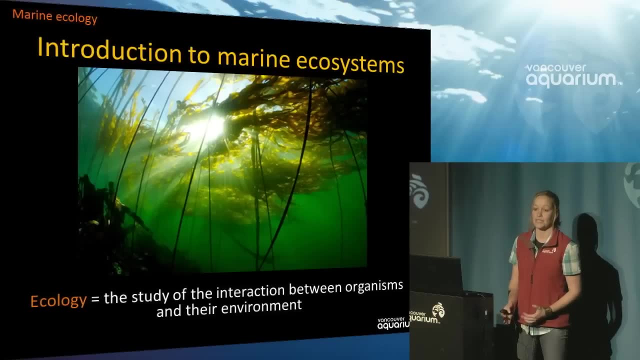 Now, once you know what you're looking at and you know the species that are there, then you can start to ask- ask other questions, like ecological questions. So ecology is the study of interaction between different animals and plants and their environment. 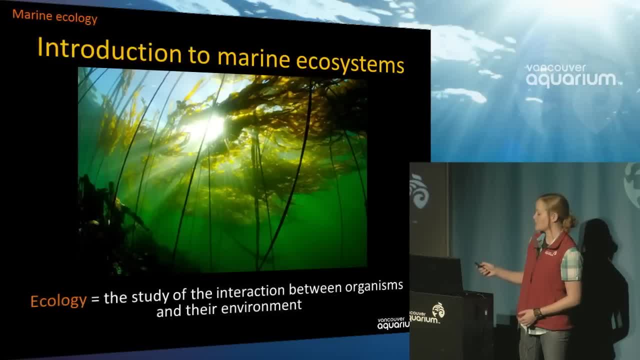 So we're asking questions like: why is there so much kelp in this picture? Is it because of the availability of light? Why, for example, isn't it all being eaten by the herbivores, like the snails and the limpets and the hermit crabs? 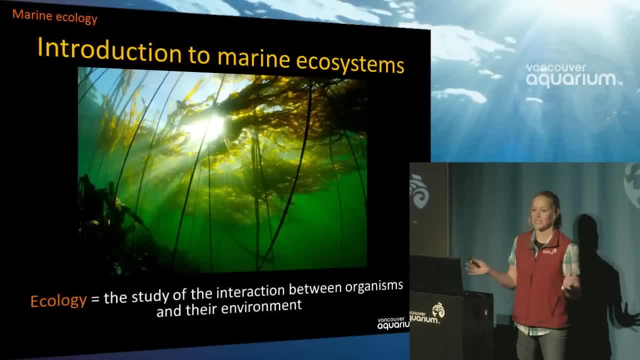 And will those populations of herbivores and plant eaters grow infinitely until they run out of kelp, Or are there other things that are keeping those numbers down? So those are the kinds of things that we're interested in asking, And those things can get a little bit complex when you start looking. 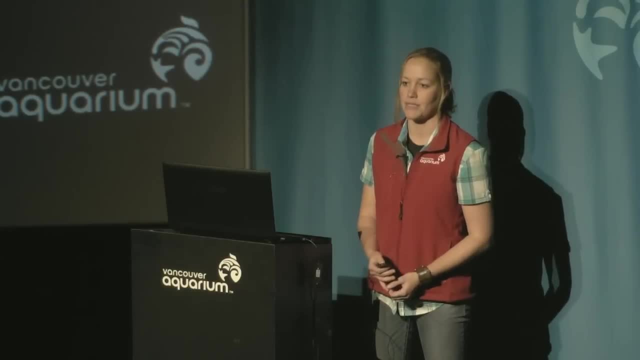 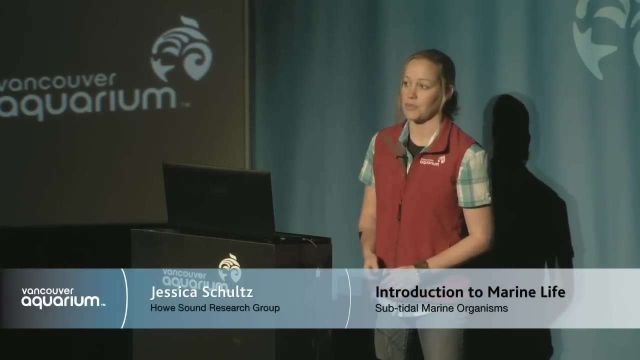 at all the different types of variables that are interacting in any one environment, And so, in an effort to get our heads around what's going on, ecologists divide ecological factors into two main groups. The first one is the abiotic factor. So an abiotic factor is anything physical. 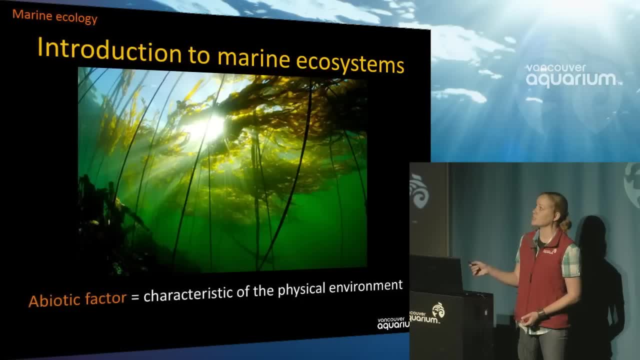 any physical characteristic of the environment, such as the light, which we mentioned earlier, or the chemical composition of the water, things like temperature. The other category, biotic factors, is the factors that involve other living organisms interacting with one another, such as predation or herbivory. So we'll go through a few examples. 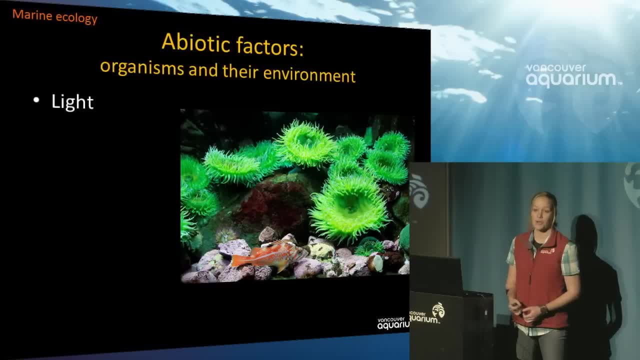 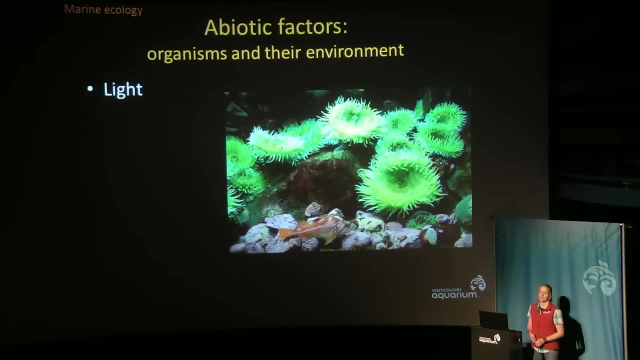 of both of these. With abiotic factors, one of the more obvious factors is light, So light can limit or impact organisms in a number of different ways. Here in this picture, we see an anemone that looks green, And the reason it's green is because there's microscopic algae that actually 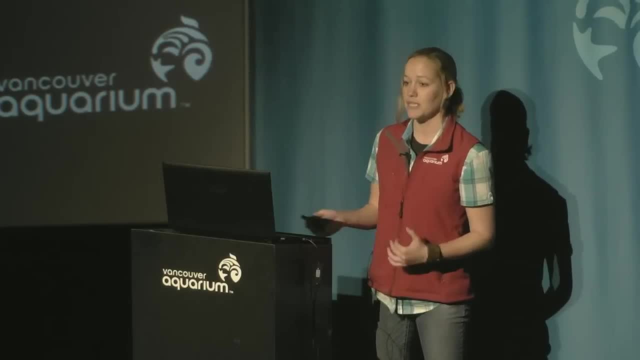 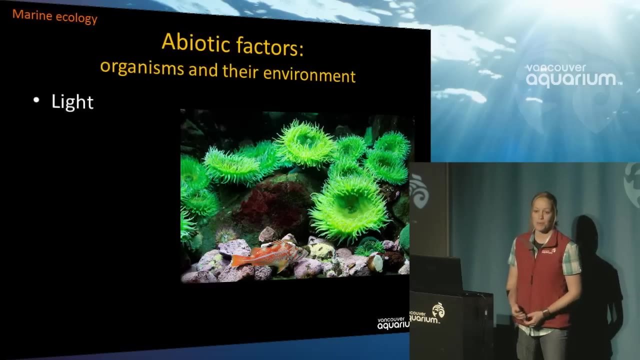 live inside of its tissues and photosynthesize, And they can only exist where there's enough light for them to produce energy out of the sunlight. So this same species of anemone, if you find it in deeper water, will actually be white, because that algae can no longer exist. Another interesting 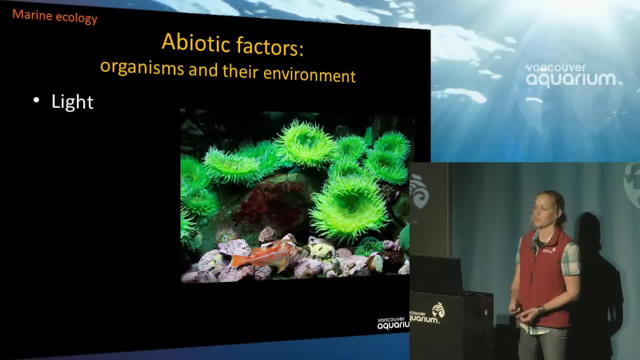 thing that happens in the marine environment is light attenuates or gets absorbed with depth. So this canary rockfish looks orange here because this picture is taken in an aquarium, But if you were actually at depth it would look brown. There's other things going on. 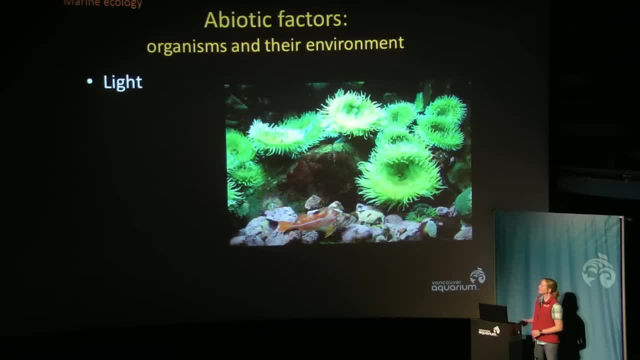 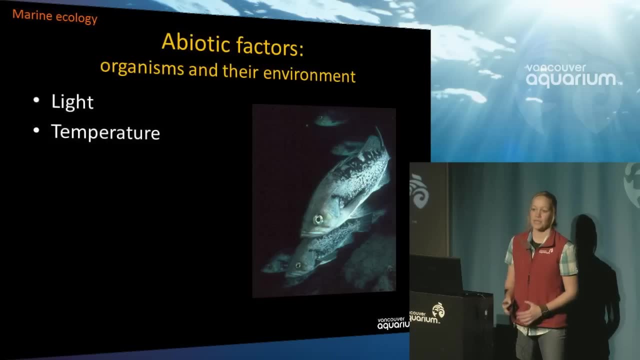 like we have some more photosynthetic pink algae and other animals that could be limited by light as well. Our next example is temperature. So most marine invertebrates and fish are exothermic, which means they don't regulate their internal body temperature like we do. So when the 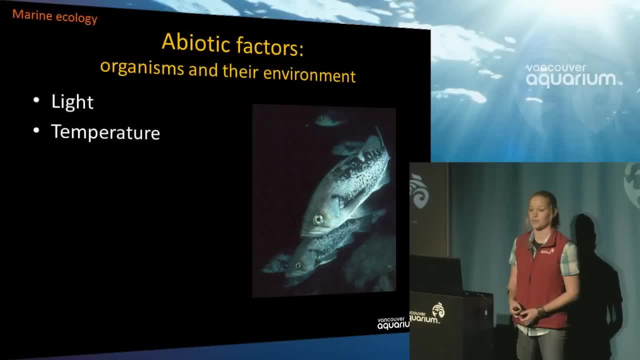 environment gets colder or warmer, the animal will also get colder or warmer. So that has a lot of impacts on physiology. Metabolism slows down and so on and so forth. So that's one of the factors that can slow down cold water and a number of other physiological functions as well. 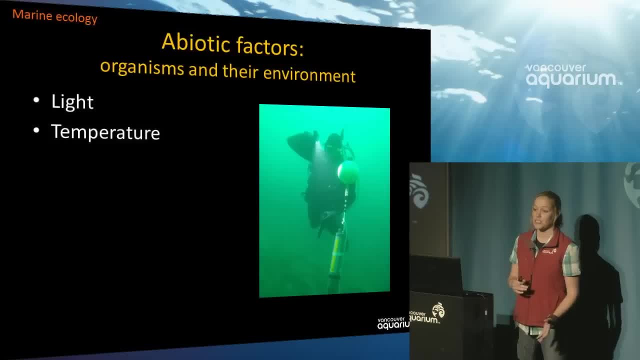 And so, because of those physiological differences of the temperature, it can really change the composition of an environment. So this is a sawn buoy, It's an oceanographic buoy that measures abiotic variables like salinity, oxygen content, temperature, And it's placed here in an area where 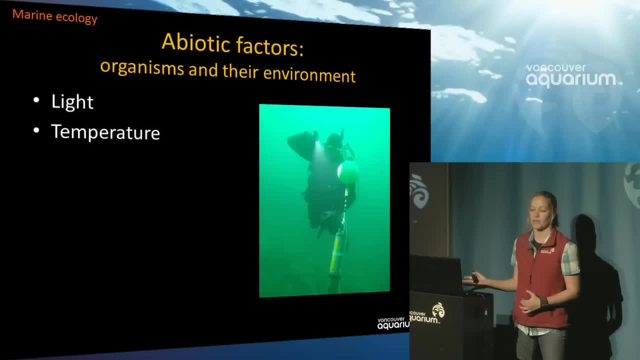 there's cold water upwelling And a nearby reef, where there isn't cold water upwelling, can have an extremely different ensemble of water. So this is a very interesting example of what we can do. So the temperature has not changed in the past. It's changed in the past and it's a very important. 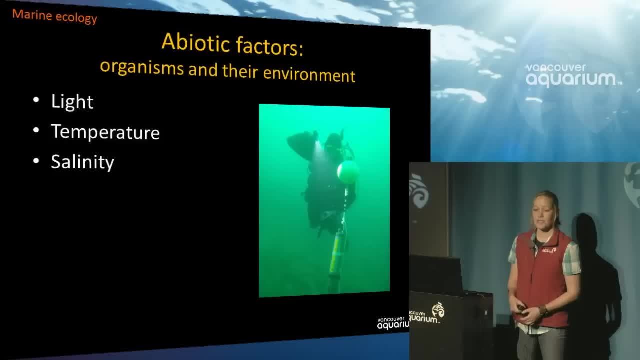 factor for organisms living, even though all other factors are very similar. So temperature is very important. Another one is salinity, So that means how salty the water is, And if you've ever spent a lot of time in the bathtub and your fingers get wrinkly, that's because the water in your body is. 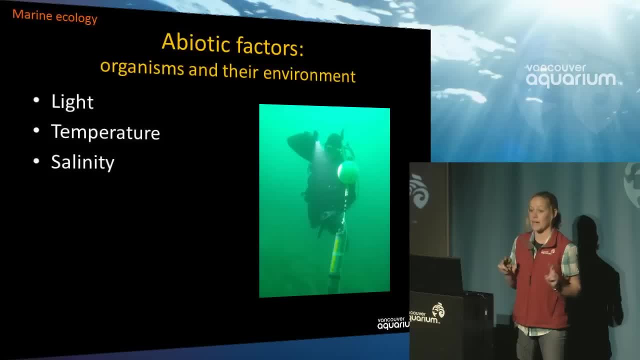 moving outside in order to compensate for the salinity. It's called osmoregulation Now for marine animals that are in the bathtub, so to speak, all the time. osmoregulation is a constant energy, and so having different salinities can really influence where 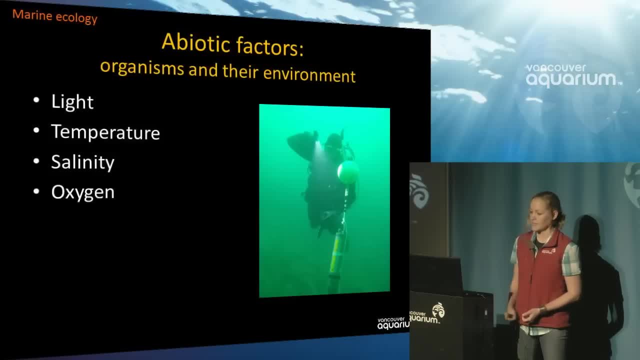 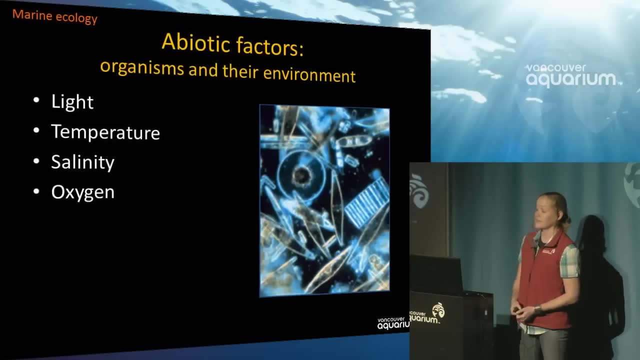 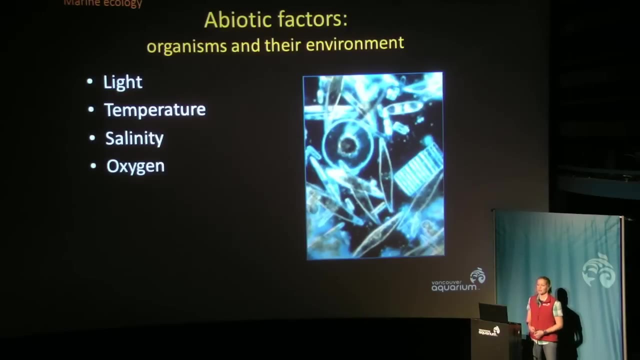 organisms are able to exist. Similarly, oxygen also will impact where organisms live. You can also have other chemical elements of the water, like in this case silica, will affect different organisms. These are diatoms. they're microscopic photosynthetic algae and they're made out of glass, essentially, and glass is. 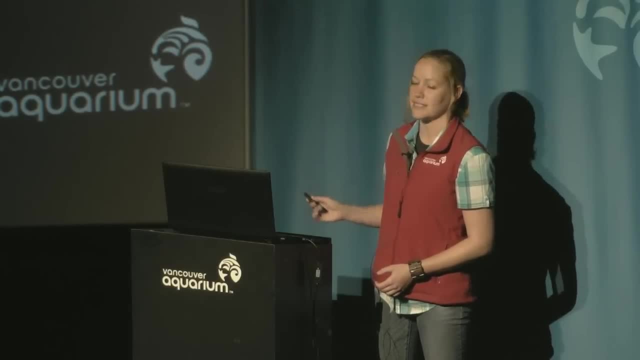 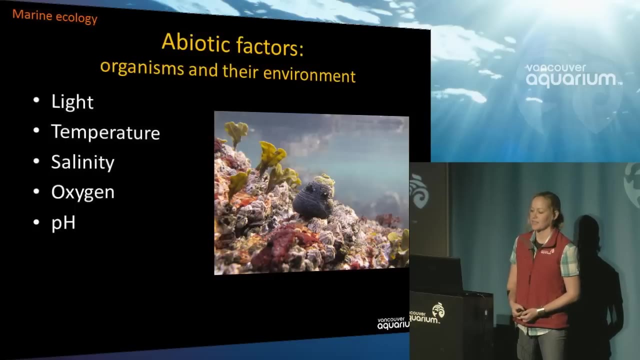 silica, So they'll do better in areas where there's a lot of silica content in the water. Another one, pH- that refers to how acidic or basic the water is, and acidity is is a widely studied variable at the moment because of climate change. When the atmosphere gets higher contents of carbon dioxide, it gets absorbed into. 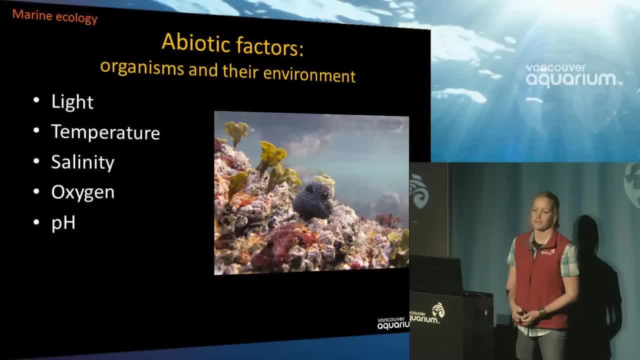 the ocean, which decreases the pH of the water, making it more acidic. That process is called ocean acidification. It's been referred to as the evil twin of climate change And for a lot of people who live in the United States, they're more likely to live in the 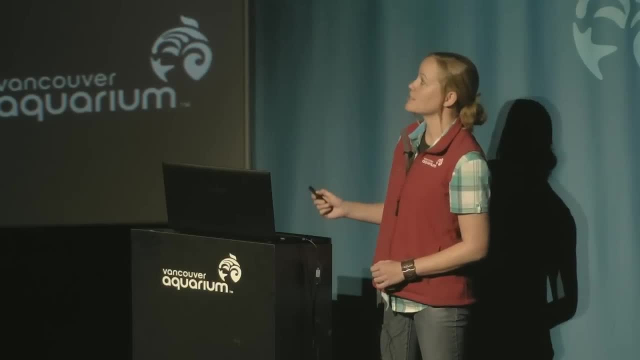 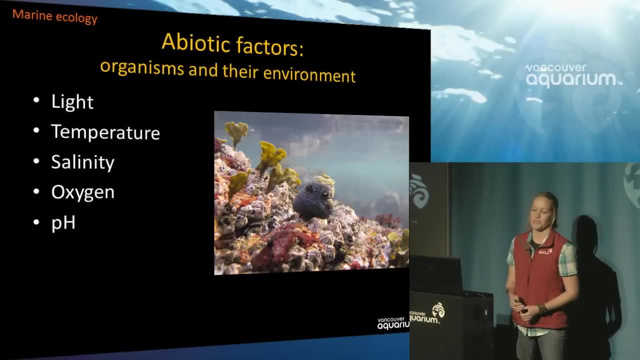 ocean. So you can see here that this is a very significant change in the climate change. So the fact that we have so many organisms in the marine realm, that makes a big impact. So this snail here builds its shell out of carbon, calcium carbonate, which is limestone, and building limestone is a lot more. 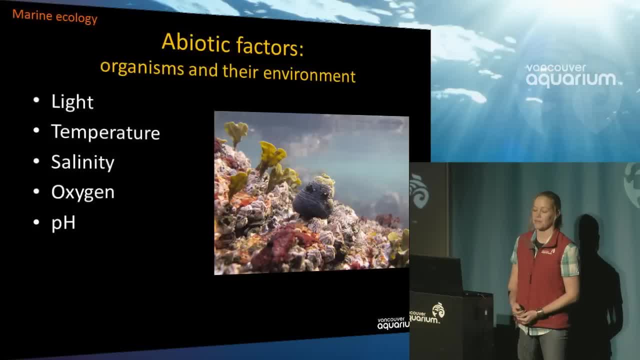 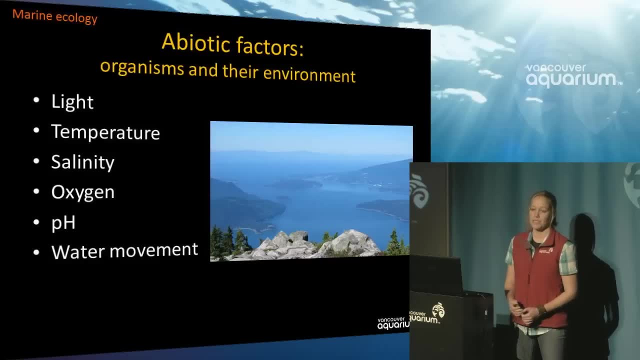 difficult in acidic water. Same thing with the acorn barnacles here. So any animal that builds a shell out of calcium carbonate may have a climate change. So this is a really active area of extension that is even more a much larger impact on the climate. So we 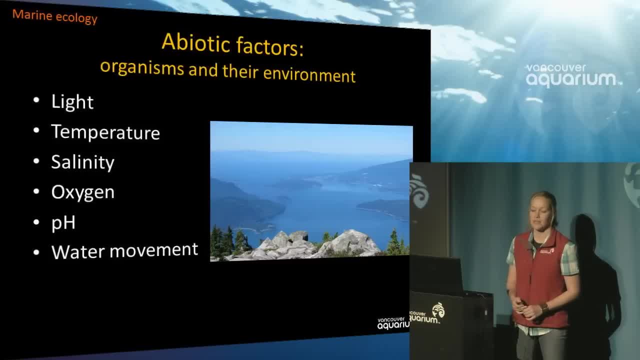 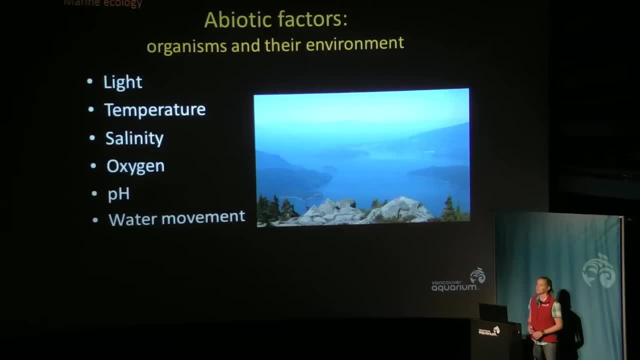 mentioned how low and high currents can have a different group of organisms living them, and that's because water current and water movements will affect all the other variables, such as oxygen, salinity, temperature and, at some degree, light will also change with current as well, And when you consider all abiotics. 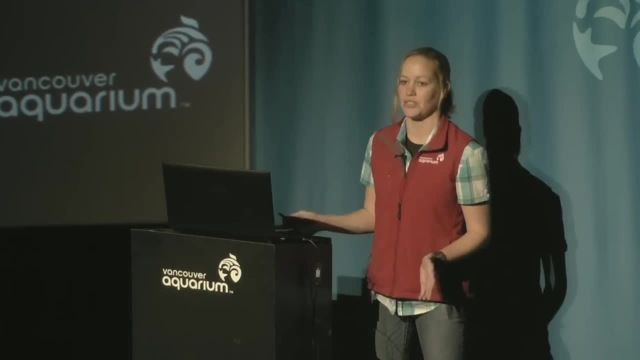 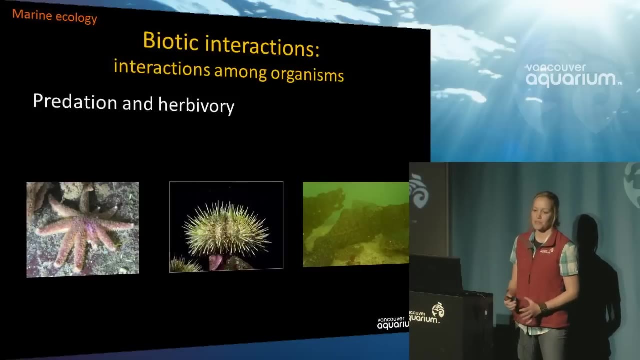 conditions together and over long periods of time. that's when you start thinking about climate, which is the long term changes in different weather conditions. So now we're just going to move on to the biotic interactions. So the first one is first one we'll talk about is predation and herbivory, So that's animals eating. 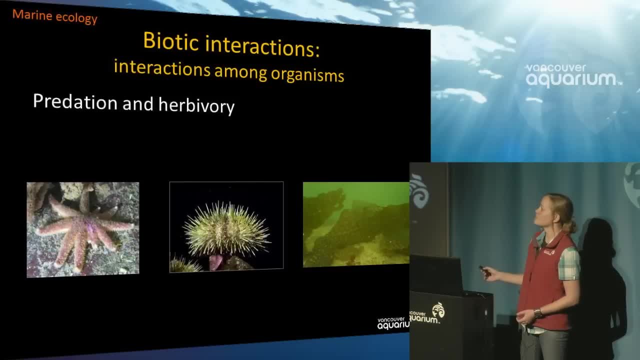 other animals or animals eating plants- in this case algae- and that's one of the more readily observable interactions you can see in nature. Biotic interactions can be considered either positive or negative. So in this example, for the sea star which eats the sea urchin, it's a positive thing for the sea star because 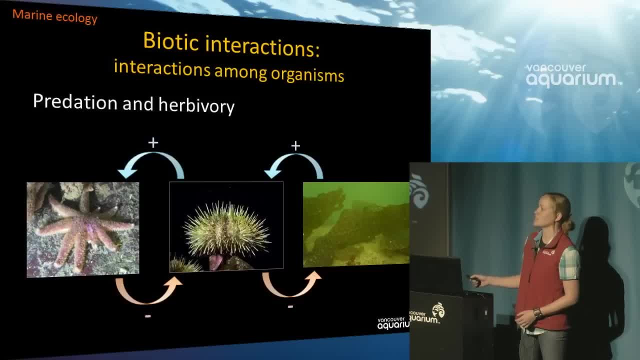 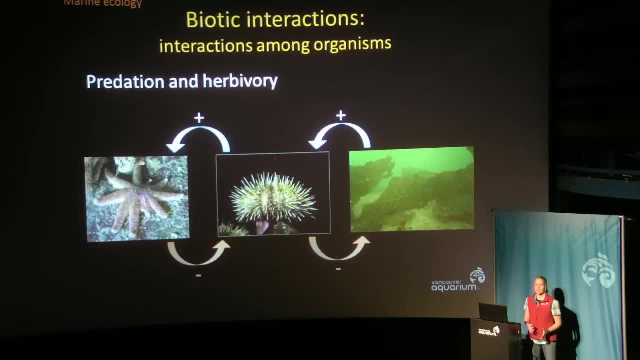 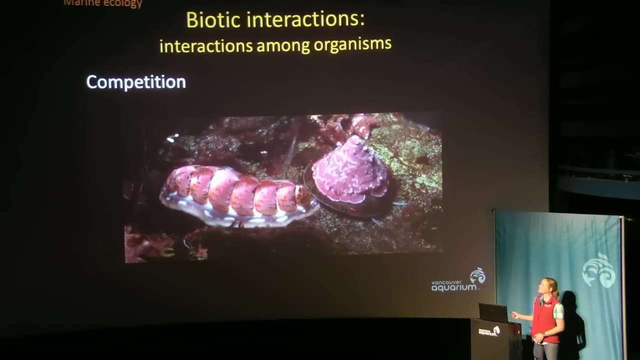 it's gaining food, and of course it's a negative thing for the sea urchin, because they're threatened by predation. And exactly the same interaction cycle is taking place between the plant eater and the algae. Next example is competition. So in this picture we have a snail and a chiton which both graze on. 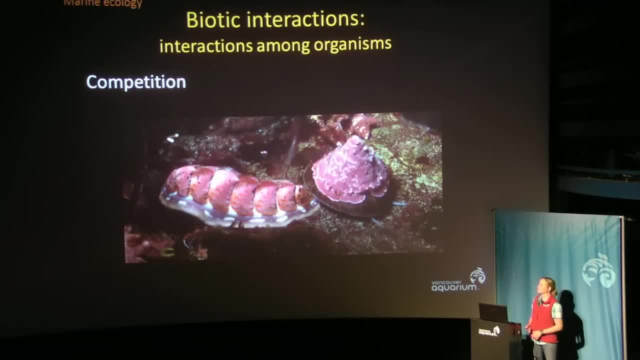 the surface of rocks for microscopic algae or larger algae if they can get a hold of it as well, And so they're competing not only for food but also for space, And in the case of competition, it's a negative, negative interaction, because they're competing for food and they're competing for food and they're. 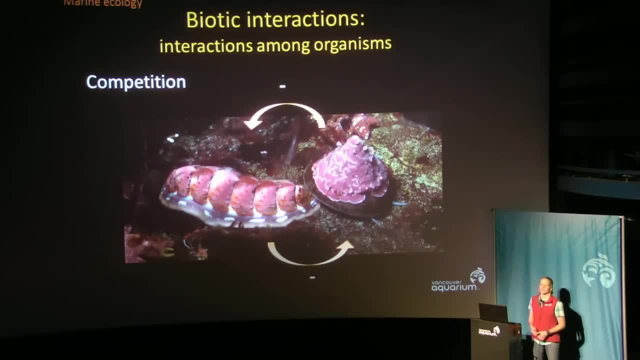 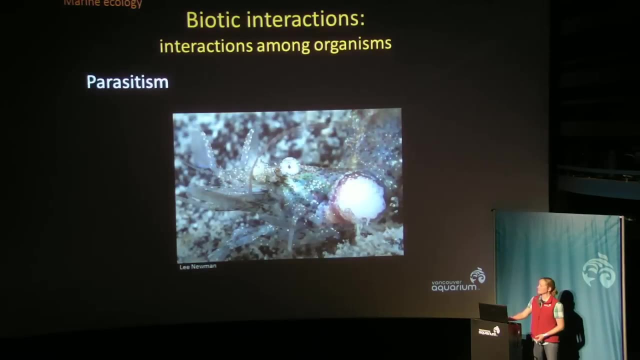 competing because both organisms have to lose out in order to compete for the resource. They're spending more energy to compete or they're obtaining less of whatever resource you might be referring to. So competition isn't necessarily for one thing, but it can be for a number of different things at the same time. Next, 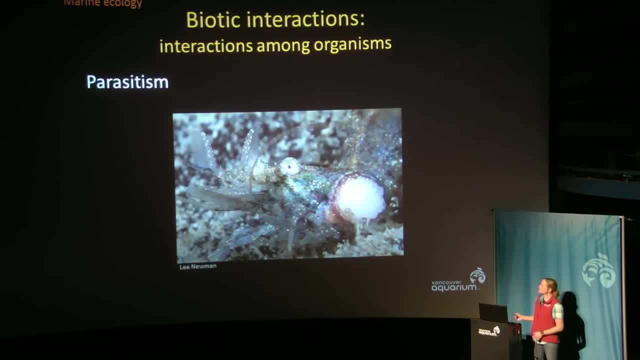 we'll just mention parasitism. So here we've got a shrimp that's got a parasitic, parasitic isopod that's actually laid its egg mass underneath the exoskeleton of the shrimp. So in this type of interaction it's good for the parasite and negative for the. 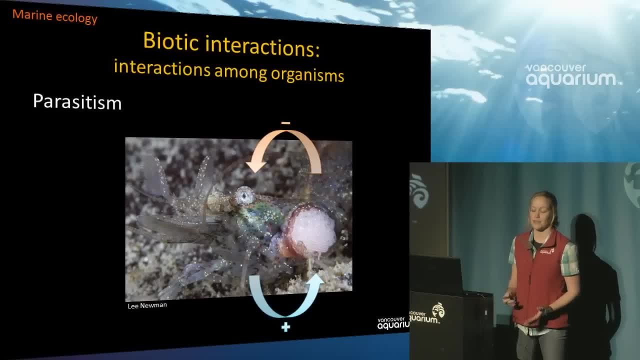 host And while most hosts don't kill the correction, most parasites don't kill the host, because it's actually better for a parasite if the host can persist, because it can draw the benefit for a longer period of time- There's still going to be at least some negative impact for the shrimp. It's going to have to sustain the 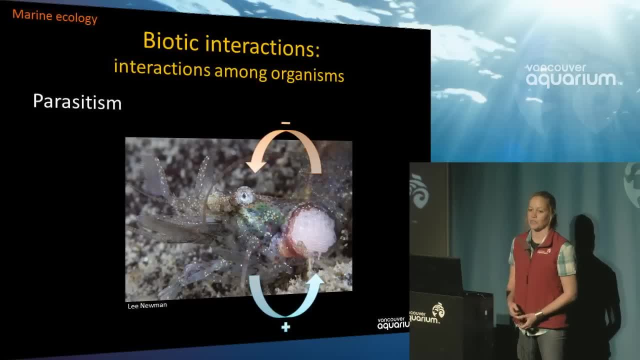 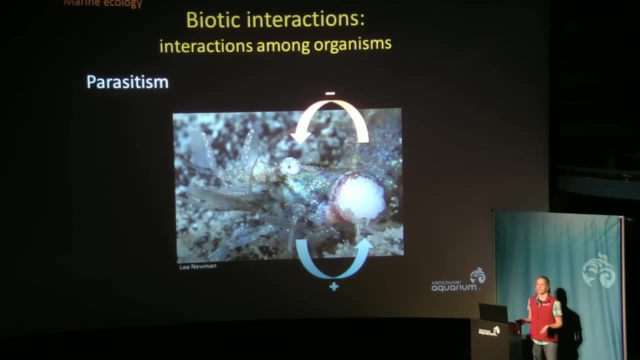 injury, of having its exoskeleton ruptured and it's going to be more vulnerable to infection and that type of thing. Whereas for the isopod it gets protection for the eggs and in this case, once these eggs hatch, they'll rupture the exoskeleton, go off to infect a new. 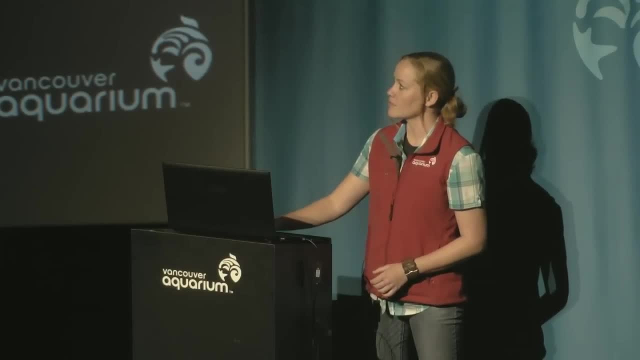 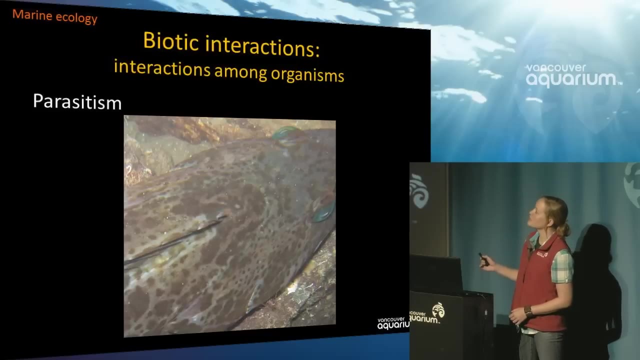 host and the shrimp will will not die. So parasitism can lead to other interactions as well. So Donna mentioned before that the lingcod can have parasitic copepods underneath the skin. But in this picture we have our cleaner shrimp- Our elegant, cleaner shrimp that we mentioned earlier- Down there picking off. 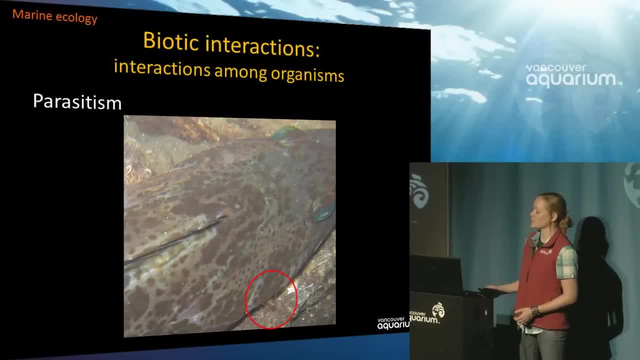 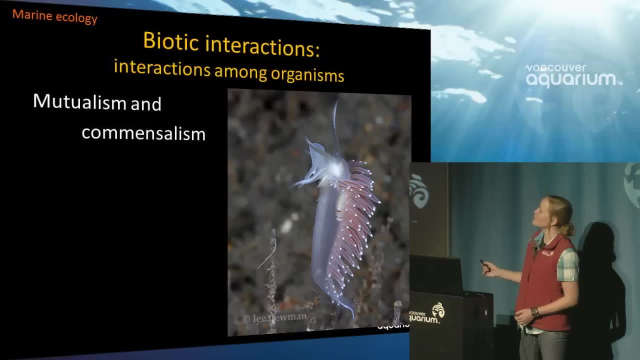 those isopods as a form of food. So this type of interaction is actually called mutualism or commensalism, which is our next interaction that we're going to talk about. In this picture we've got a nudibranch and it's got a scale worm. 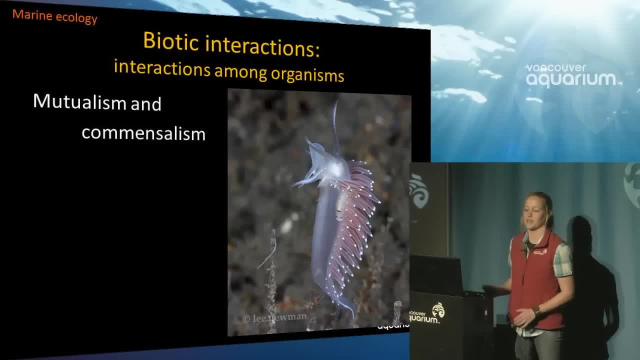 that lives on the side of it. It's not harming the nudibranch or inside the nudibranch, but just living there as a way of transportation and protection. potentially So these stinging projections on the nudibranch might be protecting the worm and the worm will actually rear up kind. 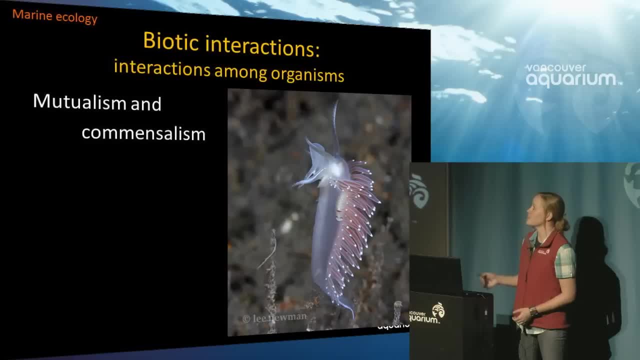 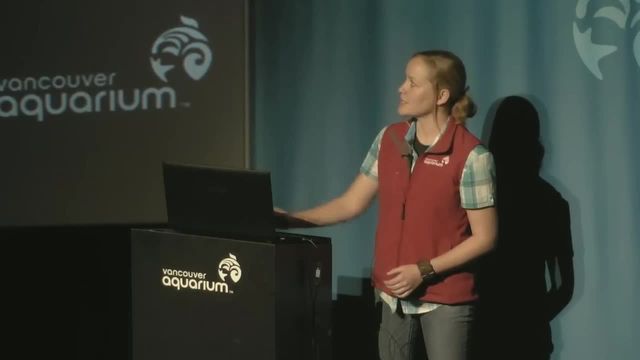 of like a guard dog when other organisms get, get closer. so that's been observed when this, when this worms on snails and limpets and such. so it's probably going to happen with the nudibranch as well. so this type of oops in this type of 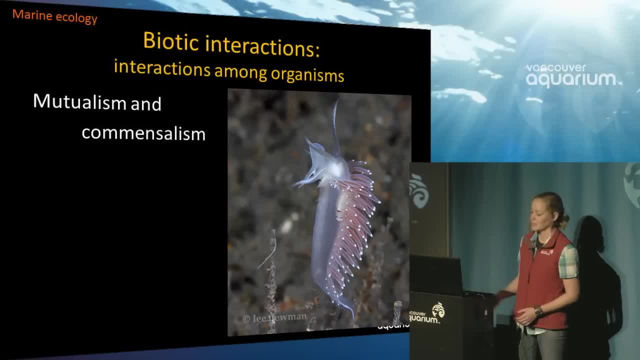 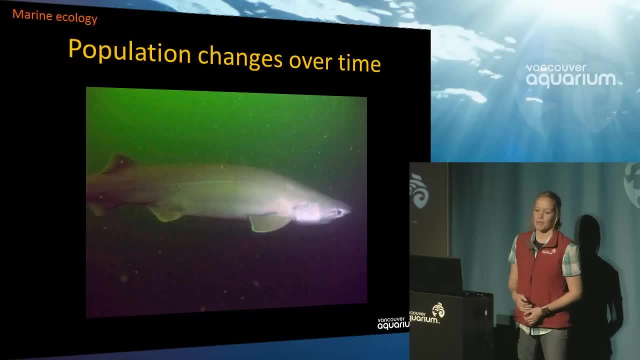 interaction. it's positive, positive or neutral for both animals, so that one's mutualism, when inter, when biotic and abiotic interactions are present for a long period of time, they can lead to population changes. so one example is with the sixgill shark. it hadn't been seen in our biodiversity records. 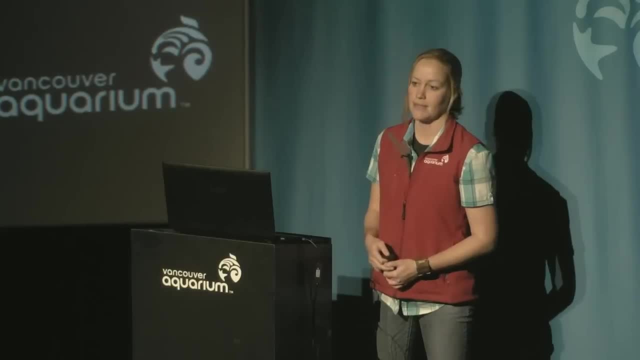 previously at all, until 2011, when it was seen once, seen once in 2012 and it's been seen three times this summer, so that might be from a result of more food availability, with the return of, potentially, the Pollock and herring and other animals. we've also been seeing more cetaceans, and how 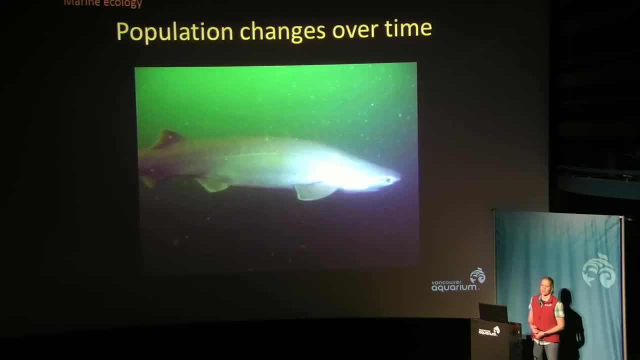 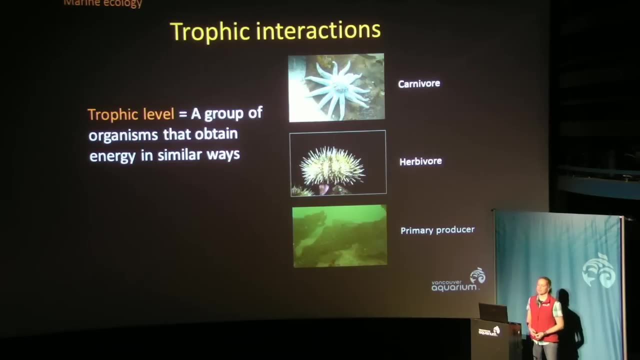 sound recently, and that might be from a whole number of different factors which are probably related. you can also look at more than one interaction at the same time. so ecologists often talk about trophic levels. so trophic levels are defined by how an animal or plant obtains energy. so in the primary later, 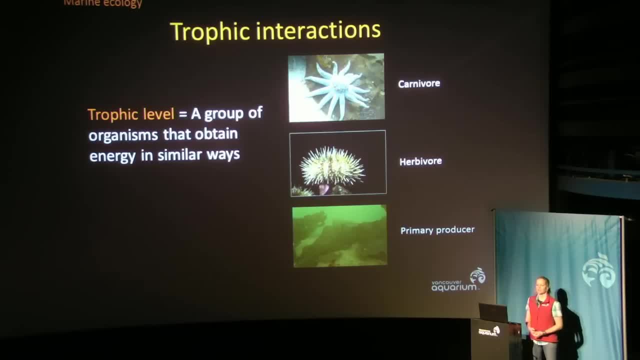 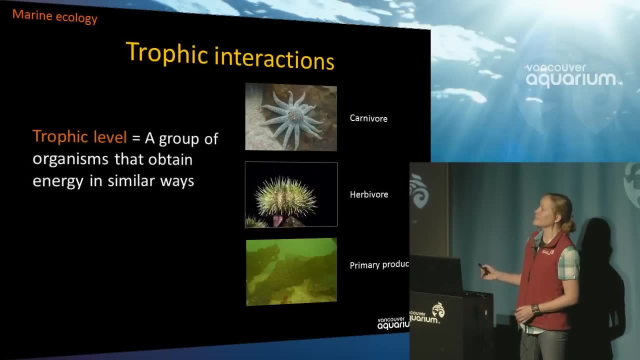 layer at the primary producers. they're obtaining energy from either the Sun or from chemistry. they don't need to consume anything else to get energy. the second level, the herbivore or plant eaters, are consuming the primary producer, and then the carnivore or predator will be consuming herbivores and 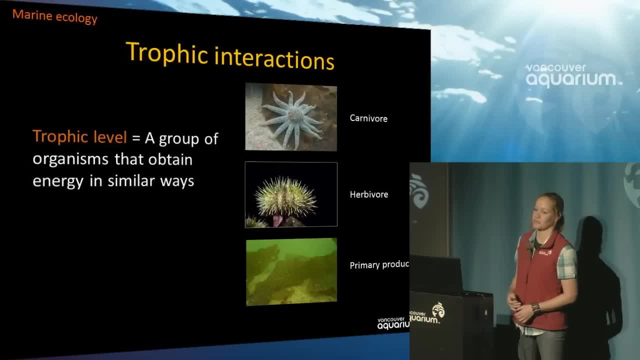 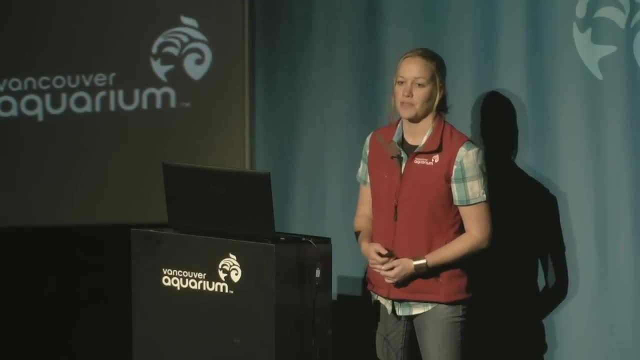 you can have multiple trophic levels at each. in each division. trophic levels can be act, can regulate populations, so equal. just like to talk about either bottom-up control or top-down controls. So that refers to what's limiting the growth of the population In. 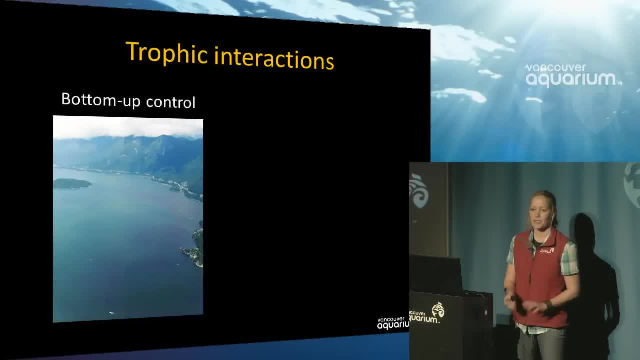 the marine world there's not very many examples of bottom-up control, but a terrestrial example might be a hare and a wolf. So when the hare population is reduced the wolf can't grow as much in numbers because it doesn't have a food source. So that's a bottom-up control. 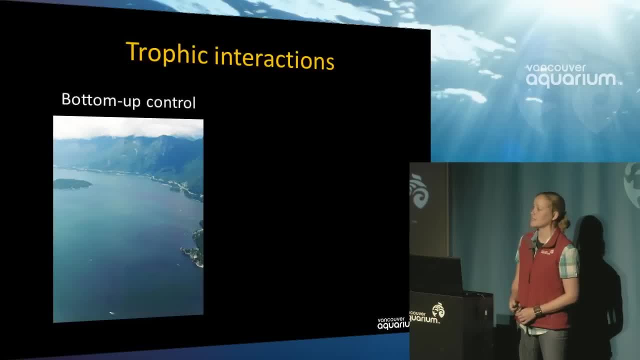 One example that we do have in the marine realm is that of plankton blooms. So when there's more sunlight and more nutrients available- which is on the bottom level of a trophic level- then the microscopic organisms are able to reproduce more rapidly, And this 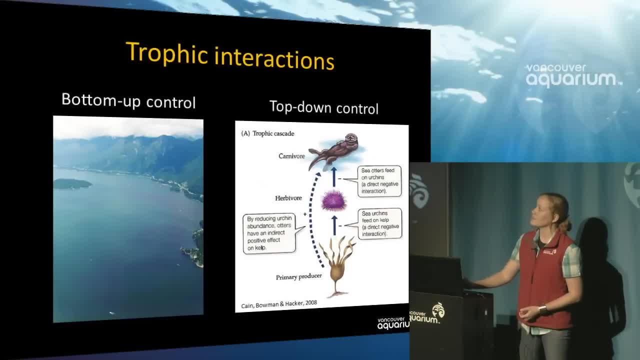 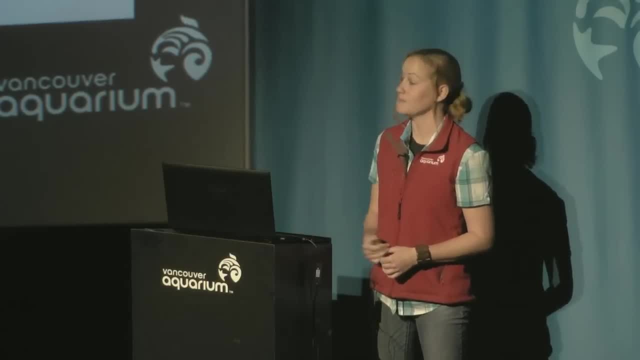 is a dinoflagellate bloom in Howe Sound. Top-down mechanisms are more common in the marine realm, So this is where a predator or herbivore is limiting the level below. So this is a famous example in ecology where the presence of a sea otter is reducing the 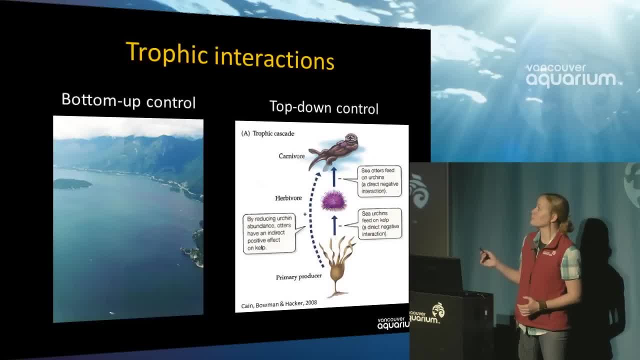 number of green urchins And similar. correction, in this case, purple urchins And similar. the purple urchin reduces the amount of kelp that can be present in the system, So when the sea otters aren't around, the urchins can just eat unchecked and consume a lot of. 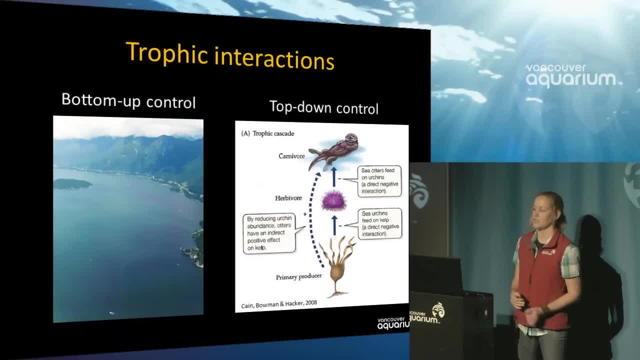 algae, which will bring down the kelp forest, and that has a lot of other ecological impacts as well. So then we can have indirect interactions. When sea otters are present, they limit the number of urchins that are around and indirectly increase the amount of kelp. So that's why 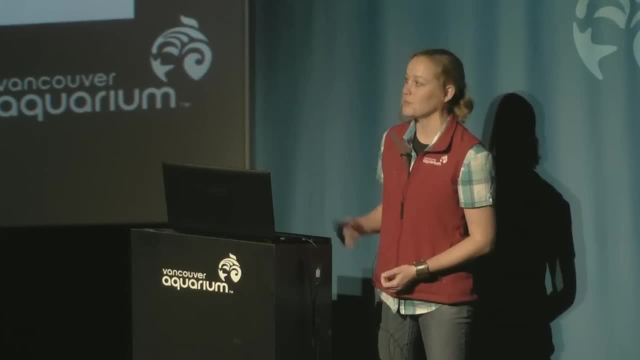 sea otters are present. They're such an important element to the ecosystem because they can maintain kelp forests, which allow for juvenile fish to have more habitat, and other organisms as well. Kelp systems are very biodiverse, So this is a really highly studied system, And when you get these indirect 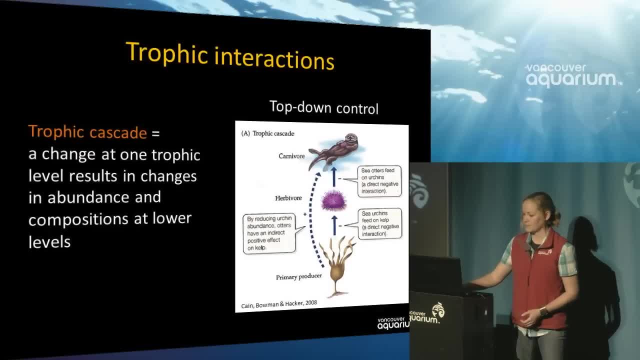 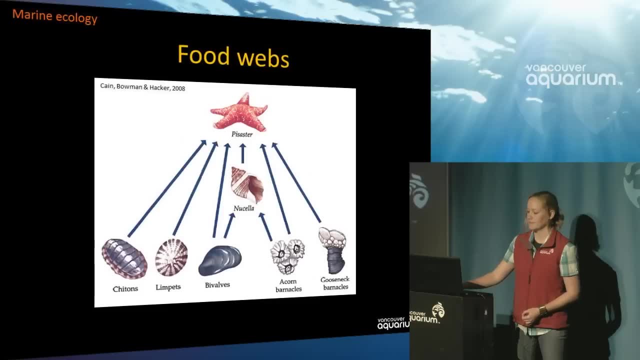 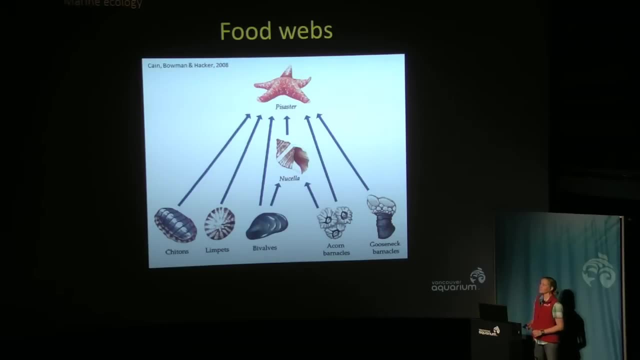 interactions like this. it's referred to as a trophic cascade, So that's where a change at one level will influence another level. You can also have food webs, where there's interactions happening in more than one direction. So if you're just looking at the top down, 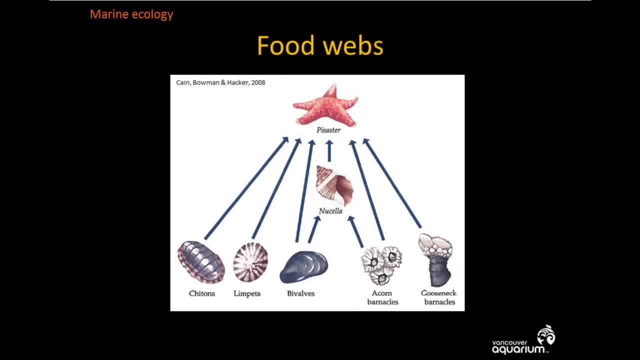 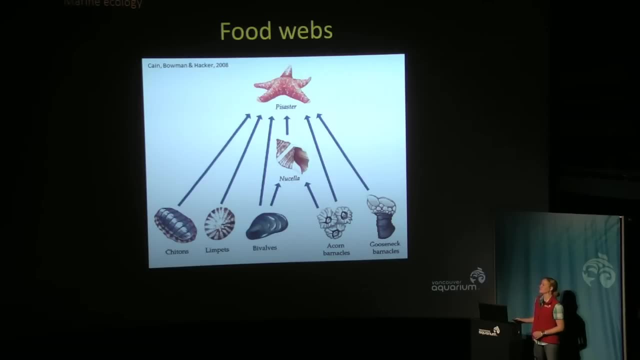 or bottom up direction. we've got the okra sea star, which consumes all the other organisms in this food web, nusella, which is a dog whelp, and both of these animals will consume mussels and barnacles. and then the sea star will also eat the chitons, limpets and the 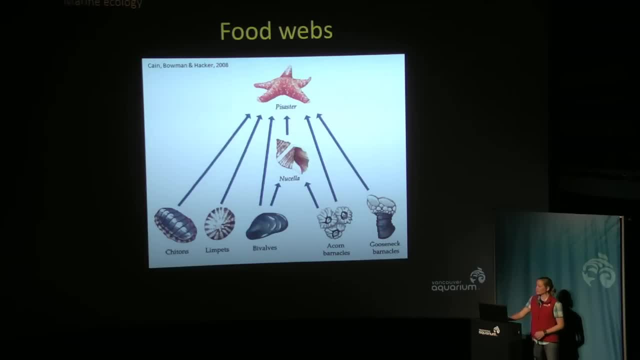 gooseneck barnacles as well. So that's when you're looking up and down, But from side to side. all the organisms in the lower level are also competing with one another, so they have a native interaction between the different groups and that can lead to some more interesting types of interactions. the sea stars. 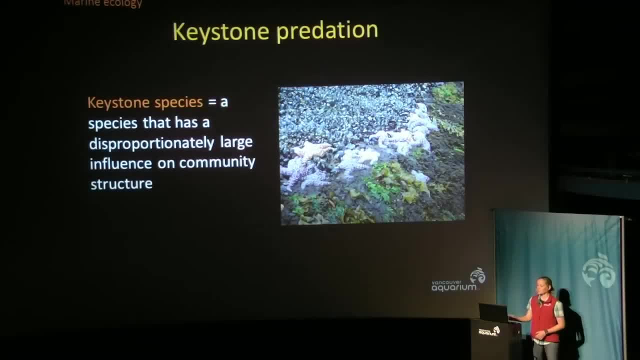 primarily like to eat the mussels, and so when you look at the intertidal realm, you can see that the sea stars will limit the number of mussels that are around, and by limiting the number of mussels actually is a benefit for the other animals in the bottom of the of the food web. here because 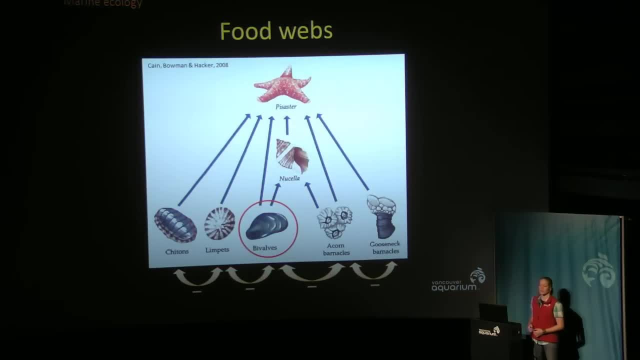 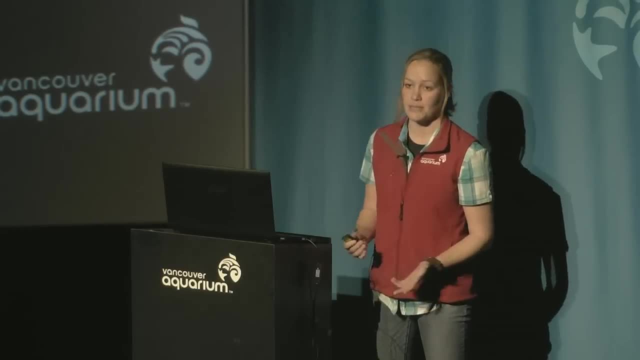 they compete for space. so without the muscles there the other organisms are able to reproduce more, occupy more space and actually by having the sea stars present increases the biodiversity in the system and you have that type of interaction. it's referred to as keystone predation, so the 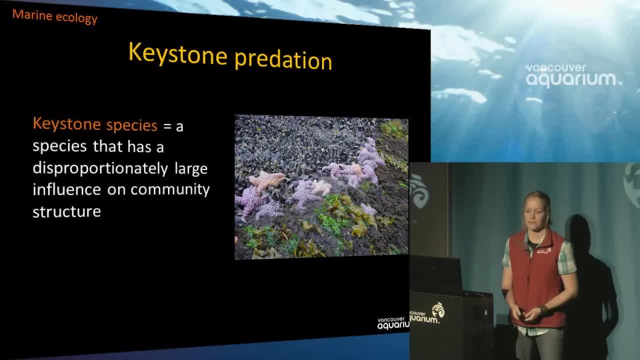 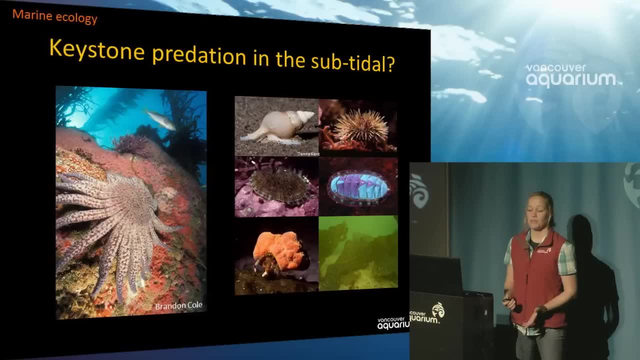 sea stars are having a disproportionately large impact on the ecosystem by increasing biodiversity when they eat mussels. does pre keystone predation occur in the in the subtitle? the subtitle ecosystems are a lot less studied, but we think that the sunflower star here might be having a disproportionately large impact on the subtitle community. it's a voracious predator. 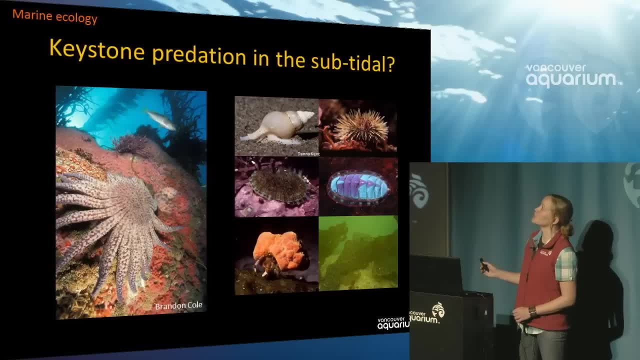 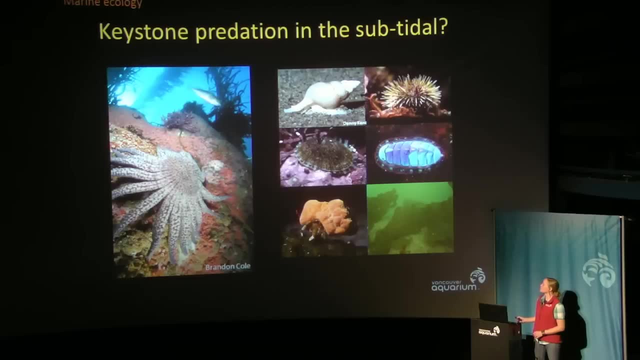 it eats pretty much anything that'll come across, including snails, urchins, chitons- i can't see what that is, i think it's an olympic hermit- crabs and possibly even kelp. and not only do these animals get reduced in number when they're 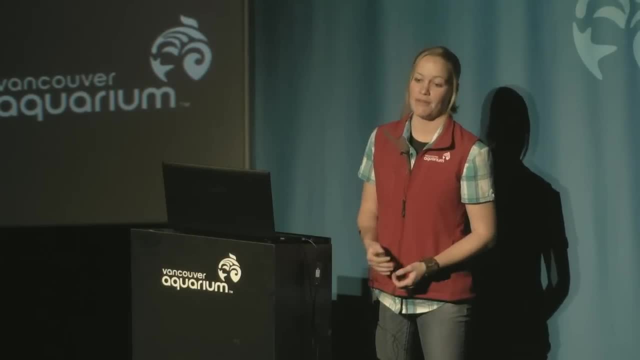 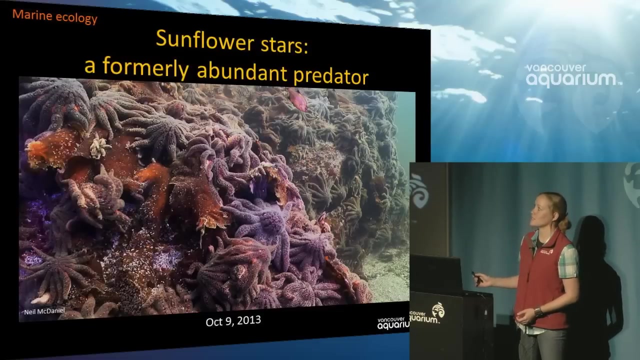 eaten by sunflower stars, but they also have adverse behavioral reactions by moving their distributions and expending energy in order to get away from the sun stars- correction: sunflower stars. so last year in a since about 2010, sunflower stars have been extremely abundant in these. 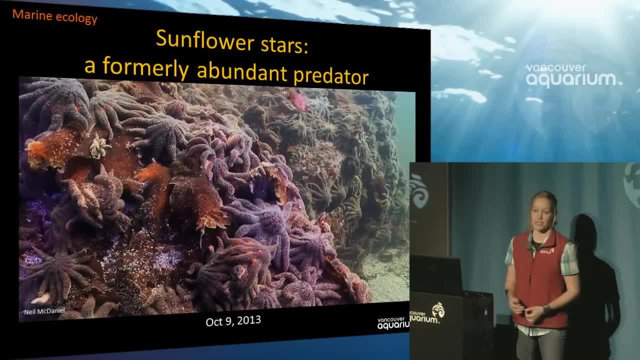 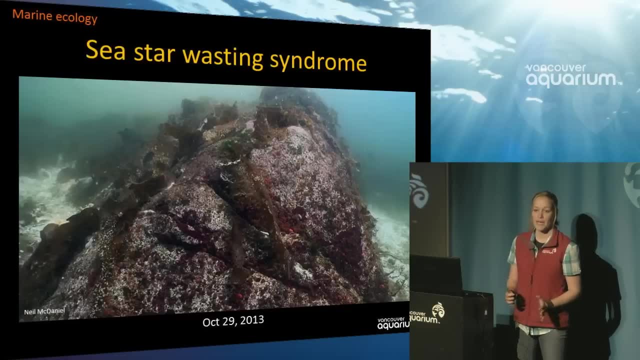 in this area. however, last year about this time in late august and early september, the area experienced a sea star wasting syndrome. so there was a mass more fatality event of sea stars and to date it's been documented from alaska down to southern california. so in the sea star wasting syndrome sea stars would lose their internal body pressure. they 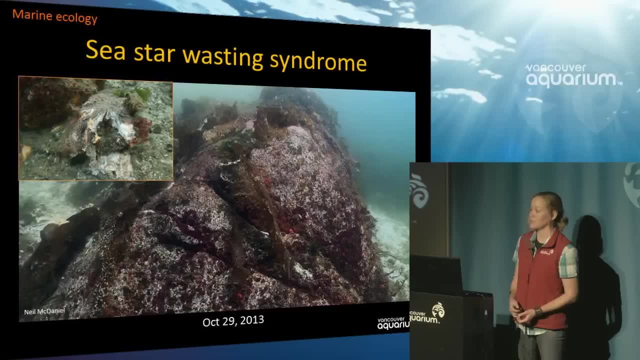 start twisting, developing lesions and eventually disintegrate in place. so you can see this image here that on the left and right is actually a river of ossicles, if you like, which is the decaying, necrotic debris from all the sea stars. this picture here is the same rock as the previous. 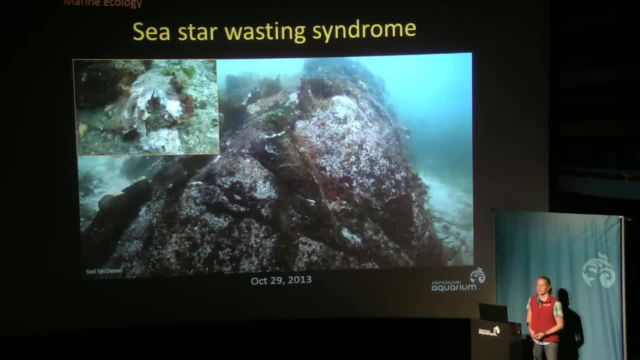 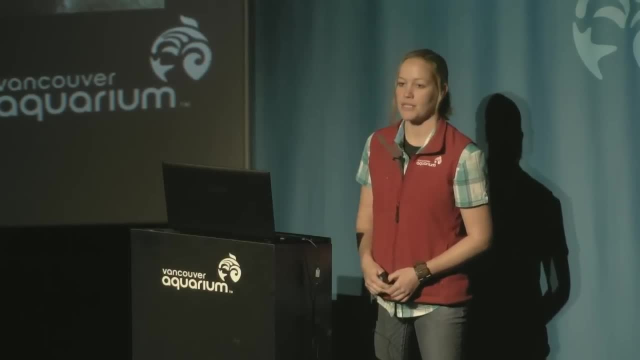 picture where all the sea stars were on there, so provided a natural experiment to investigate ecology. we're not sure what's causing the sea star wasting syndrome, but it's likely a combination of of biology: biologic factors like their abundant, previously abundant population, and abiotic things such as climate variables. so that's. 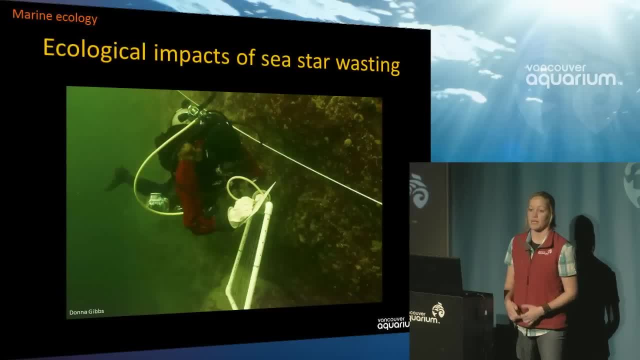 still under investigation, and one way that we're investigating it is by looking at the ecological impacts. so here we're doing a underwater transect, so that's essentially a underwater transect. so that's essentially a underwater transect. so that's essentially a measuring tape that's laid down underwater and we'll go down and we'll count all the fish. 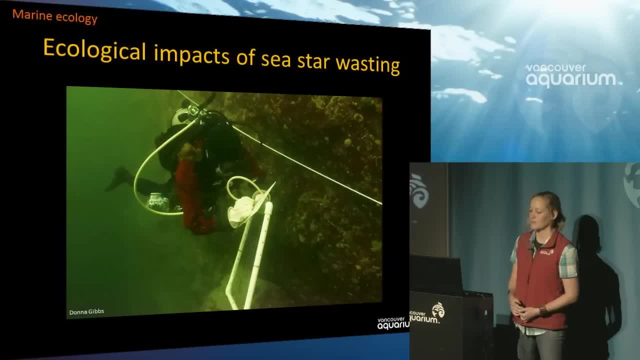 invertebrates and algae along that length of measuring tape. and in 2009 and 2010 a previous study did the same thing, looking at about 40 different sites and how sound. so we're going back to those sites this year, and next year probably as well, and we'll do the same study at the same sites. 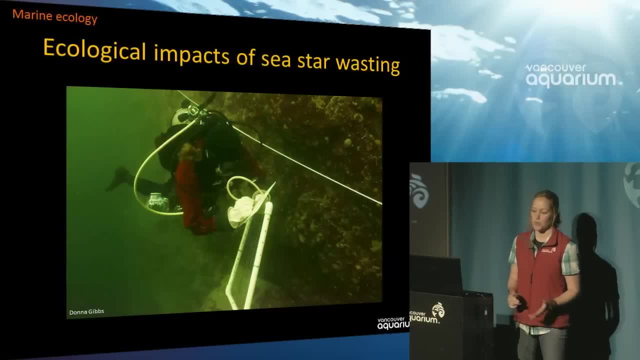 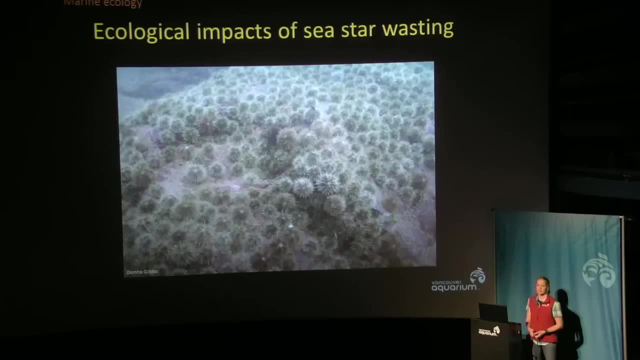 and the same depths so that we can compare the community before and after sea star wasting syndrome. i don't have too many results to share just yet, but one of the most striking things we've been seeing is a huge abundance- increase in abundance of the green sea urchin, probably because it's been 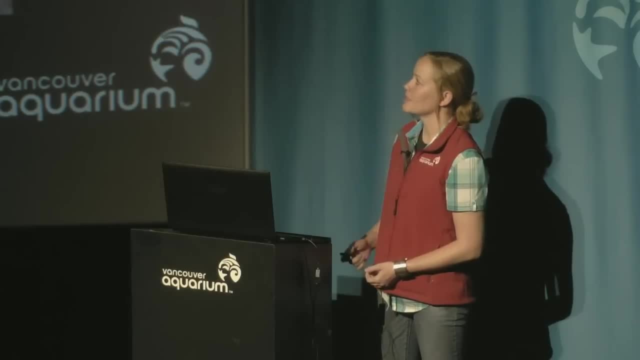 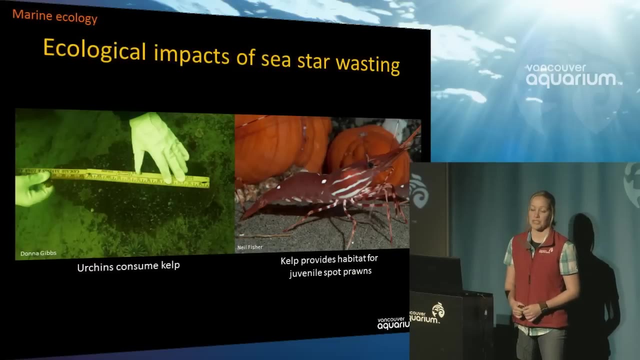 released from predation by the sea stars, and this might have other trickle-down effects in other parts of the community too. so we're going to see some of these concepts in action. in action like trophic cascades, so the trophic cascade in this case is that the sea urchins consume the agarum, which is the sea. 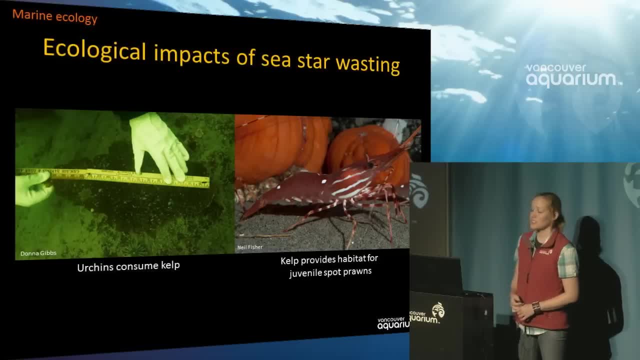 colander kelp and the spot prawn actually uses the kelp as somewhere to settle when it's a juvenile. so the spot prawns will settle out of the sea water and use the, the blades of the kelp as shelter and they'll live in and on the 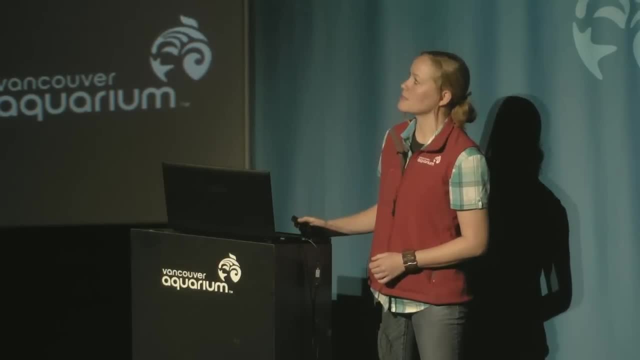 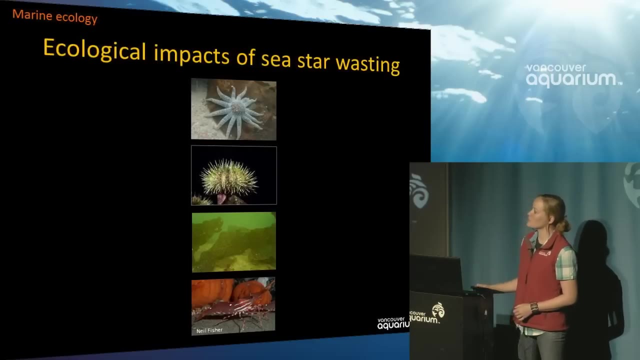 kelp. but with this, with the urchins being so abundant, they're consuming a lot of the kelp. so here we have what's sort of the normal or pre sea star trophic interactions. so we've got the sea star consuming the sea urchin, sea urchin consuming the algae. 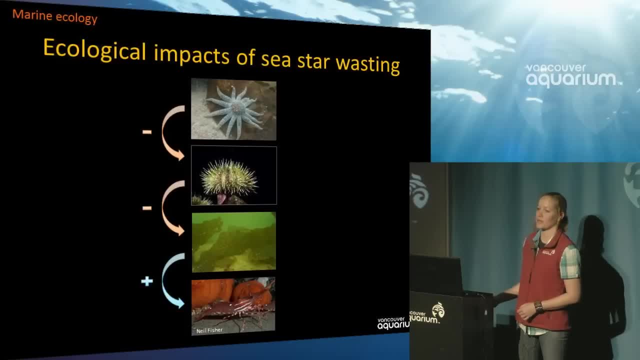 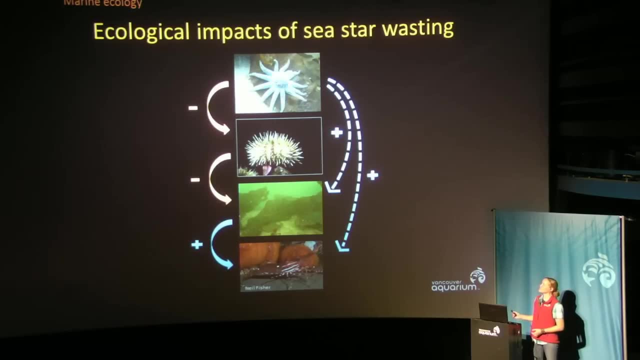 and the algae, providing a positive benefit for the spot crown by supplying nursery habitat, and the indirect interactions are that the presence of the sea star is good for the agarum because it reduces the amount of herbivory by the sea urchins, and it's also good for the spot prawn because it 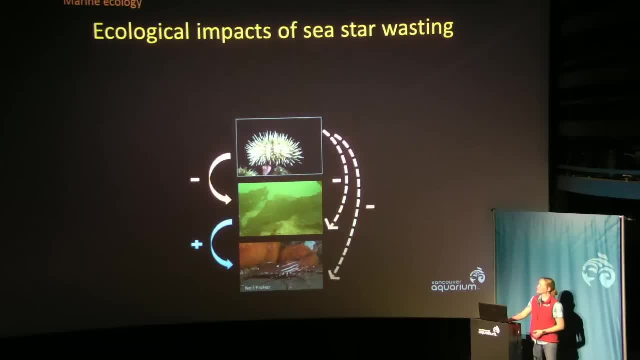 allows more habitat for nursery grounds, but in the absence of the sea star, we have an abundance of the sea urchin, and now there's even a reduced amount of kelp and a reduced amount of habitat for the spot prawn. so here we get to see a local example of trophic Cascades and 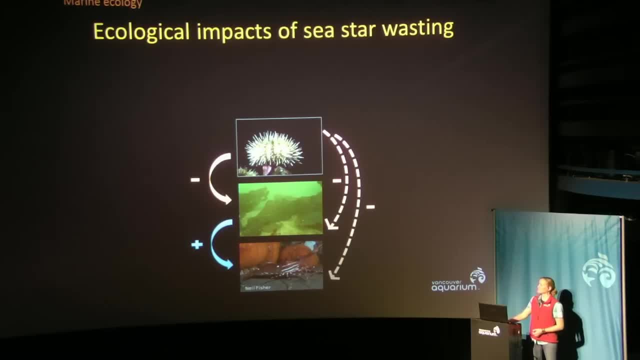 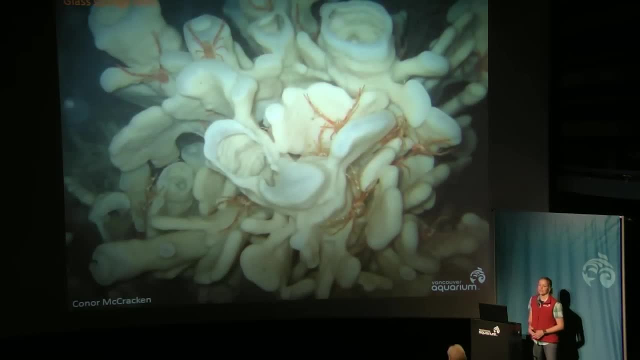 Keystone predation having an impact here in house sound. so that's an active area of research for us, and with that I'm going to pass it back over to Jeff, who's going to discuss a unique habitat here in house sound. thank you, uh, I'm going to switch gears now and talk to you just one thing. 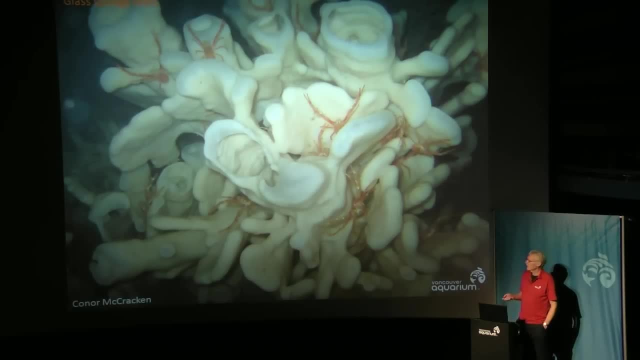 because it's kind of unique in house sound in that we can actually do a lot of diving around glass sponges and this is a shot of a cloud sponge, afroclistis, vastus, and you can see lots of little squat lobsters, a type of crustacean, and they. 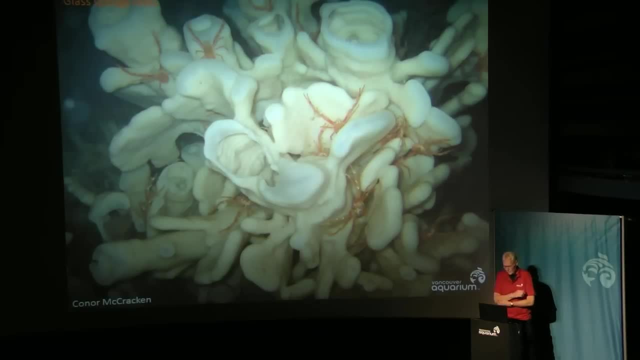 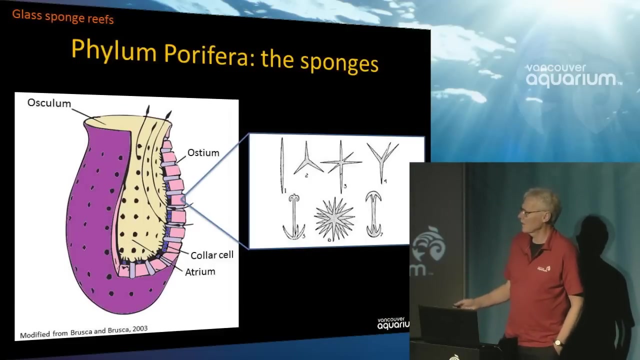 can be super abundant on cloud sponge reefs, and this is something that uh is really special to be able to see, because in most parts of British Columbia you have to have a submarine to get deep enough. now, sponges are very primitive living things that have a structure that enables the tissues to pump sea water. 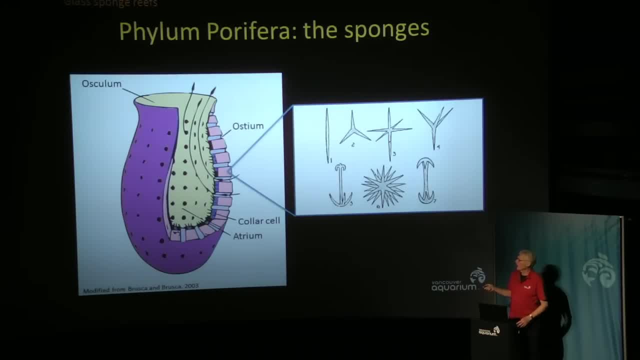 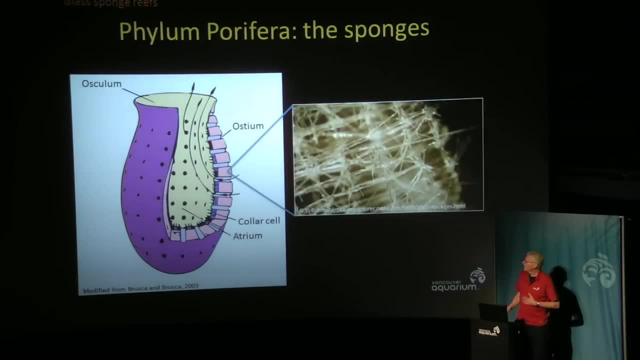 through and they filter out food items through an opening called an osculum and in the glass sponges, the skeleton or spicule Network. the architecture of the sponge is made up of glass, of silica, just like, uh, Jessica was mentioning silica being the building block for diatoms, part of the plankton that blooms in the ocean. we and most of the plants, 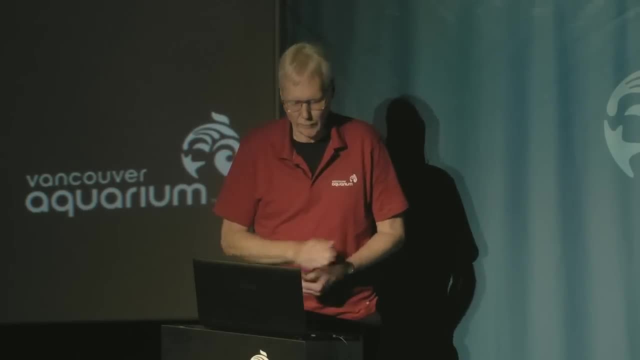 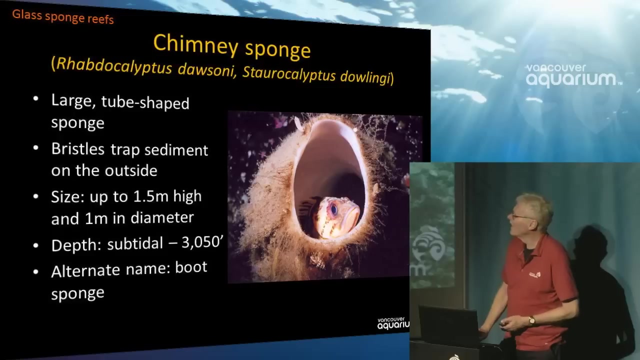 and animals on Earth are made of carbon atoms. carbon is the building block for most life, so it's kind of special to have these silica-based organisms. um, now, there are a couple different types of glass sponges, and the chimney or boot sponges are types that I like to say functions. 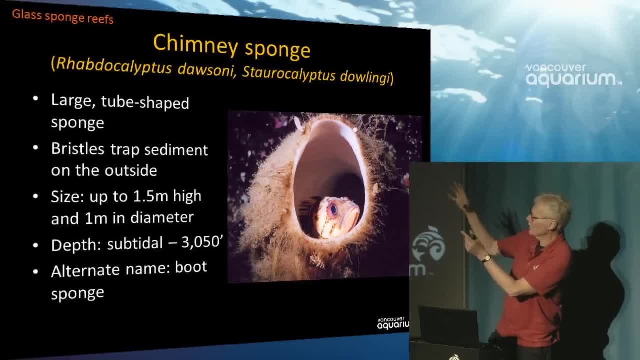 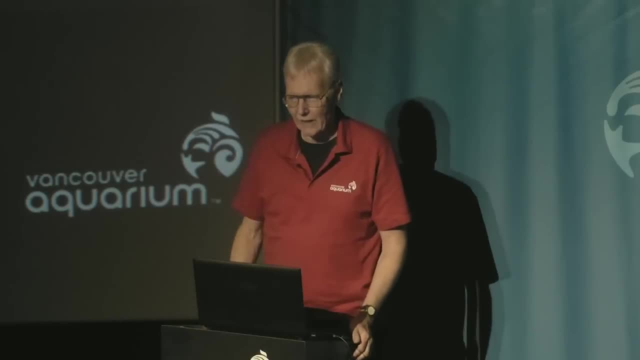 like a reverse vacuum bag because the glass spicules are in a sort of a sloppy uh mat on the outside and uh, during a diatom bloom they build up, they filter water through and a big mat of diatoms builds up and it looks very, very dark brown and then over the weeks and months it gets. 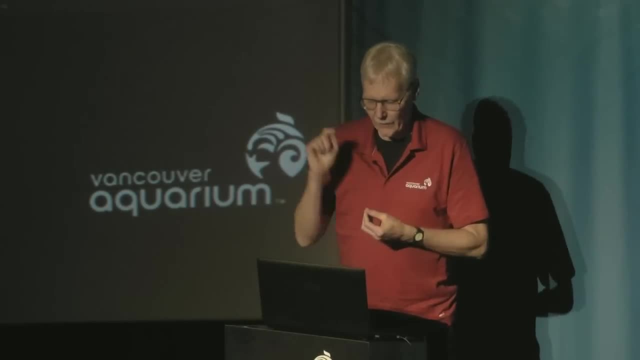 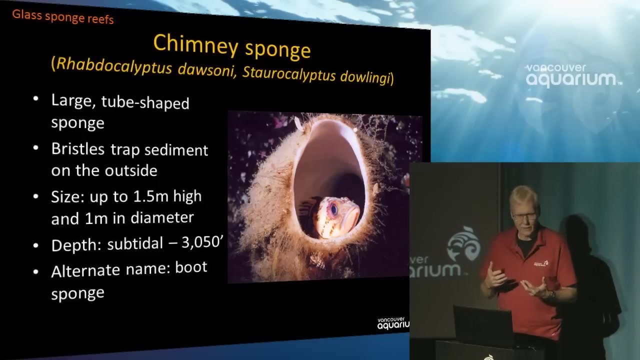 slimy and dusty looking, and so it's breaking down. now the sponges directly feed on bacteria, and bacteria are what's breaking down the diatoms. but the the breaking down of all these diatoms may actually release a higher concentration of silica into the water. nobody really understands what concentration of silica means to uh growth in glass. 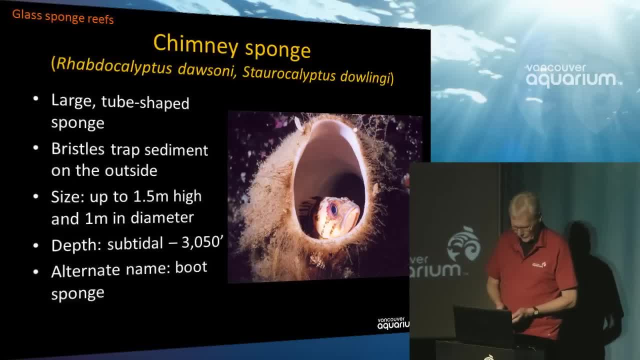 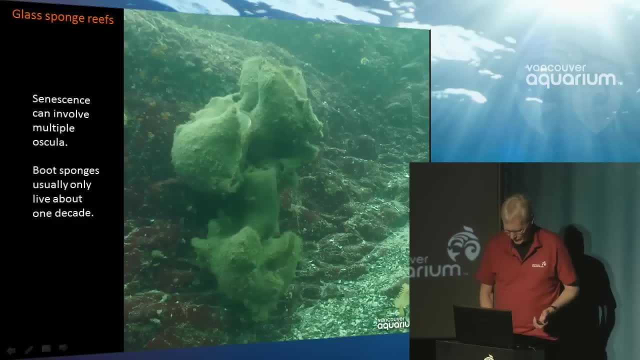 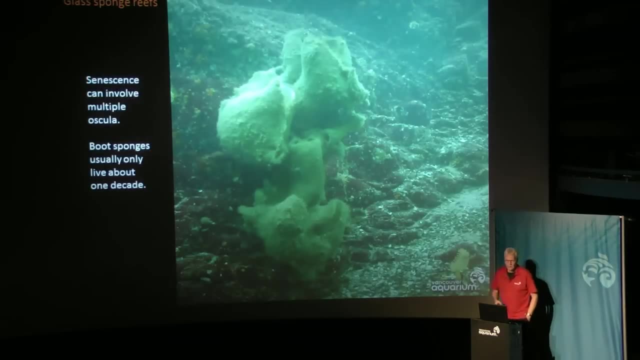 sponges. but, uh, it's, it's something that, uh, that we can take an interest in. in-house sound: oh, what have I done? come on, oops. so, uh, there used to be sort of a legend that these glass sponges are centuries old. don't touch. 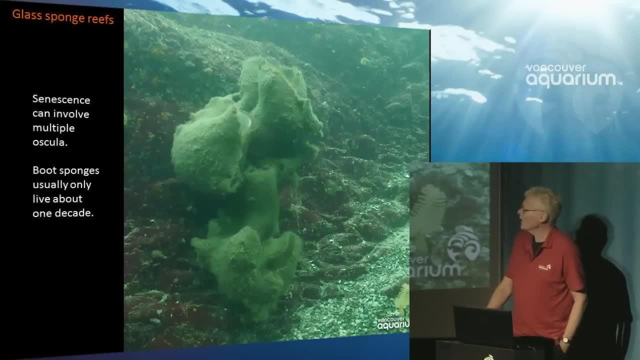 them and we've been following them- uh, in-house sound- for quite a while and we've found with the boot sponges that we can actually follow the whole life cycle. we physically tagged some of them but we've had real trouble in that they change shapes so much that you can't really recognize. 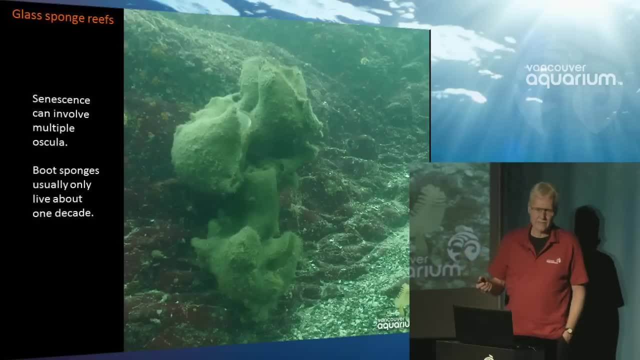 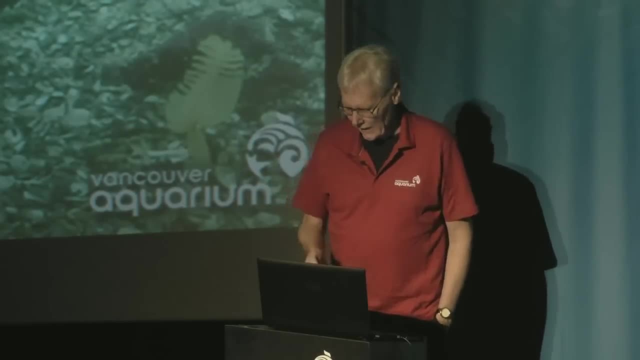 them from one season to the next. what we found is that we can recognize the geology of the rock formation. we kind of map the crevices and ledges on a cliff and keep track of the sponges and what happens is they get sort of disorganized, they get all ripply and rumply and form new oscule. this is 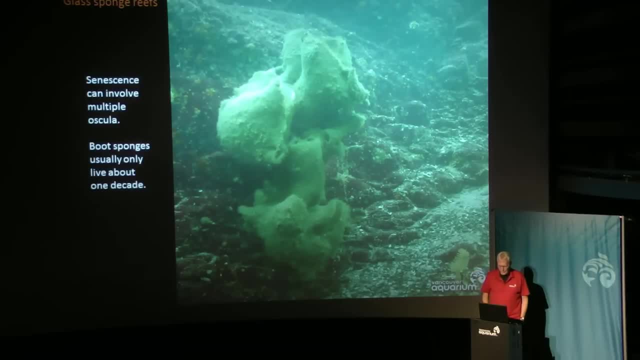 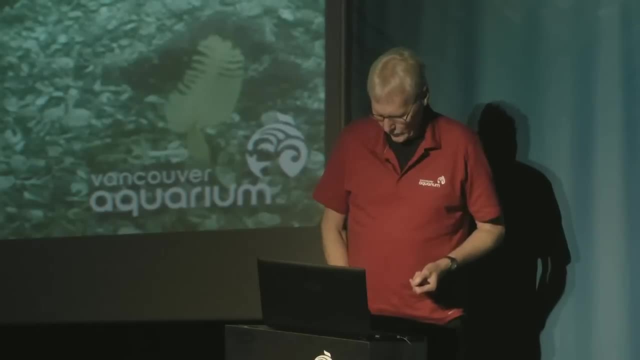 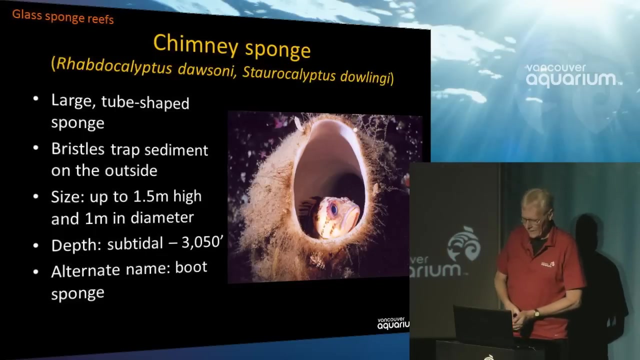 probably several boot sponges clustered here, but eventually their tissues get so disorganized that they just fall apart, and this occurs from young to old over the space of about a decade. so this is a young glass sponge with one tight osculum, and this the genera and species. getting back to taxonomy, rhabdoclyptus dawsoni and starclip this: 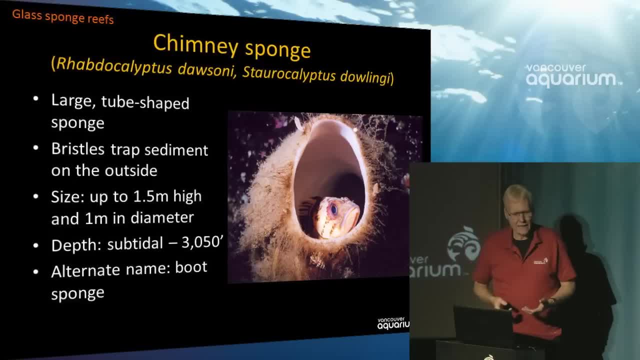 dowling eye were erected back in the 1890s when scientists dissolved the sponges in acid, looked under a microscope at the shape of the spicules and saw all the different shape of spicules. so they actually came with two different genera, rhabdoclyptus and starclip. to starclip just. 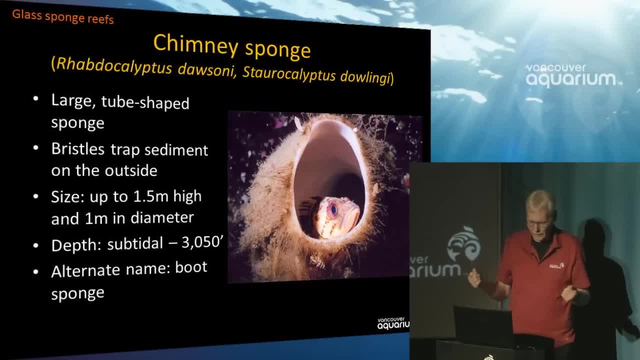 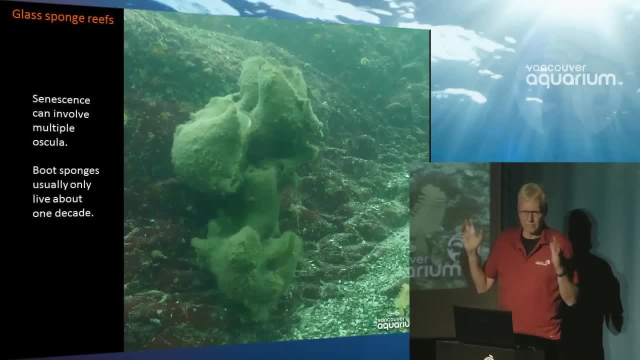 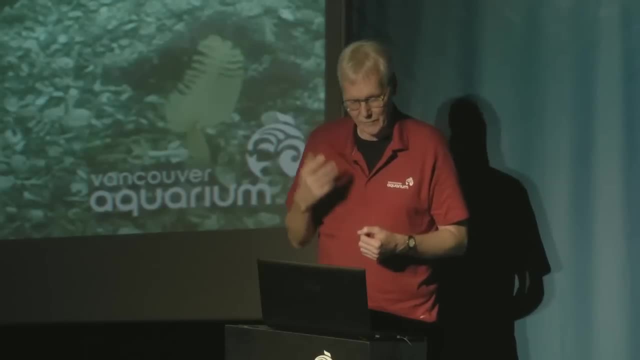 being all flared out, sort of like the rca victrola trumpet and uh. what I suspect is that, in fact, if some young scientists were to go back- good old-fashioned science, dissolving these sponges in acid and looking at the spicules- something that people aren't really doing right now- you might find 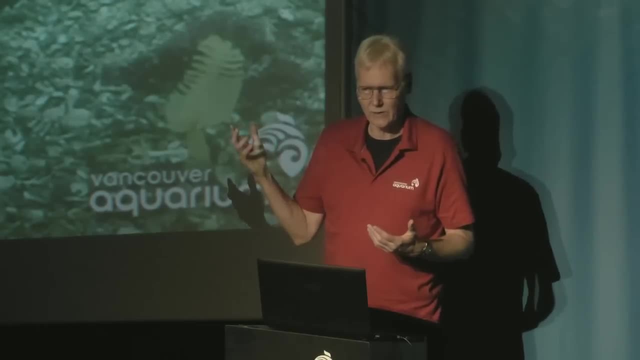 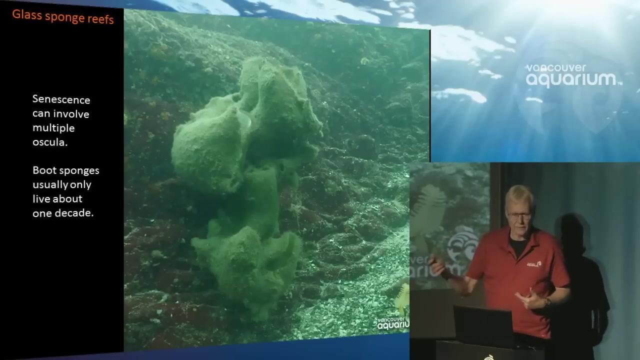 that, when they get all rippled and disorganized, that their spicules are those of the- uh, the star ecliptus dowling eye. it could be that these two different genera are really just life stages of one type of animal, so that's one of the advantages of being able to more or less live with them in. 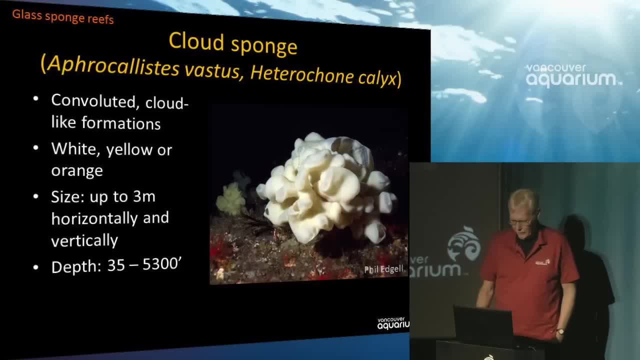 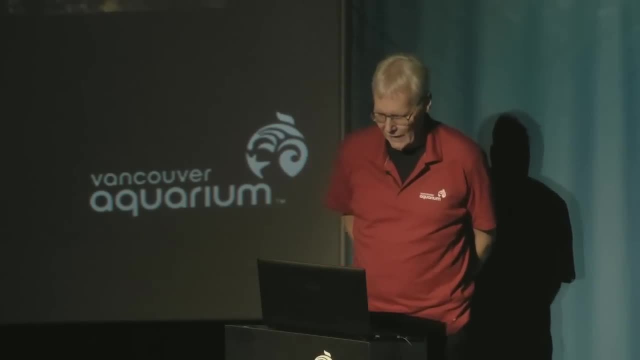 the same way that you're looking at them. so the cloud sponges are a different family within the glass sponges and we only have two genera in how sound: afroclistis, vastus and heterocony, calyx and and for the most part, all we see is afroclistis and it's the one that's named the cloud sponge. 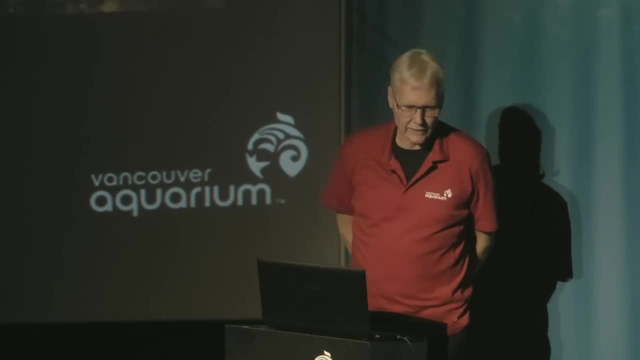 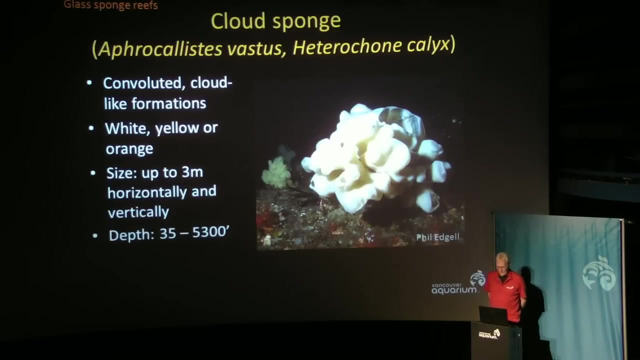 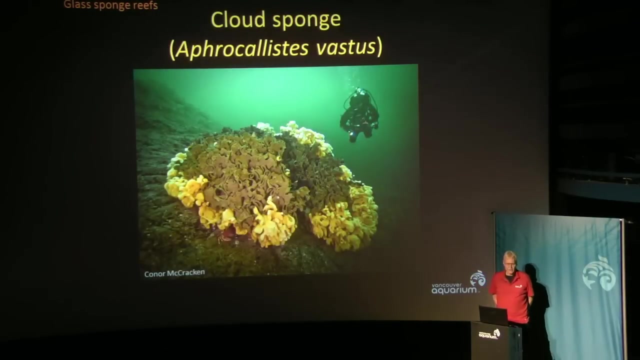 and uh, they occur from way up in Alaska all the way down in southern California and such, living on rocks, usually at tremendous depths. uh, more recently, though, that they were found to form Reefs in British Columbia. uh, oops, now this is a cloud sponge in very shallow water. in house sound that had is about the size of a. 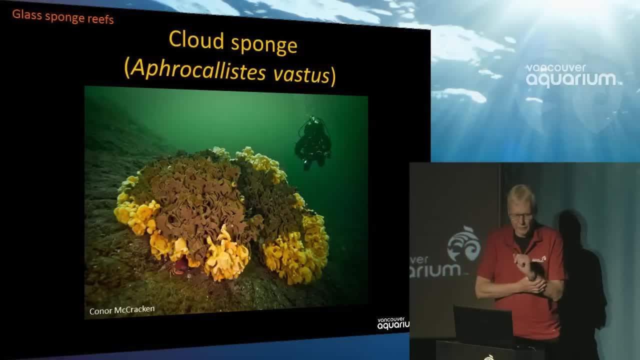 Volkswagen and it had been a big, beautiful sponge up until 2009, when we were actually diving on it at the beginning of the great 2009-2010 El Nino- a very serious warming period- and the whole thing turned translucent and look pasty and Donna was noticing a particular type of 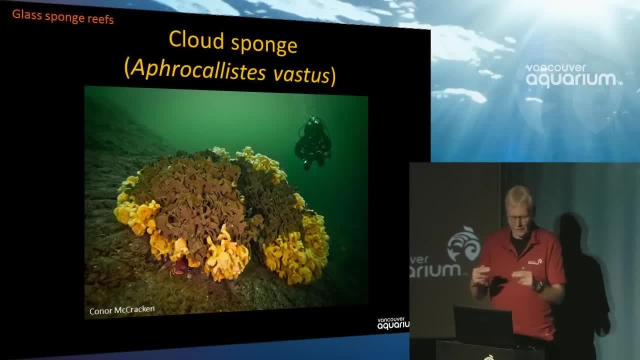 starfish, that's a predator on sponges, zooming in if a starfish can zoom um. but you know, their arms were pointed as if they were making it a rapid high board dive onto these, and they were actually climbing onto them, meaning that the tissues were failing and we thought the 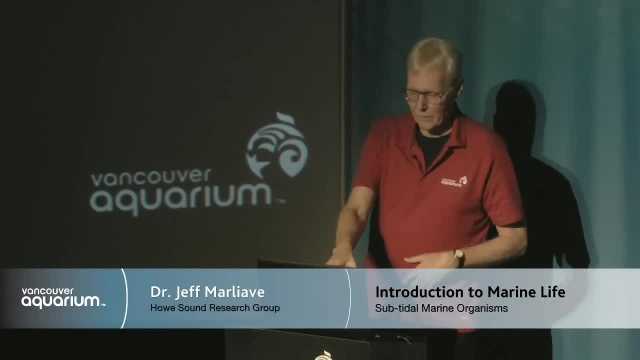 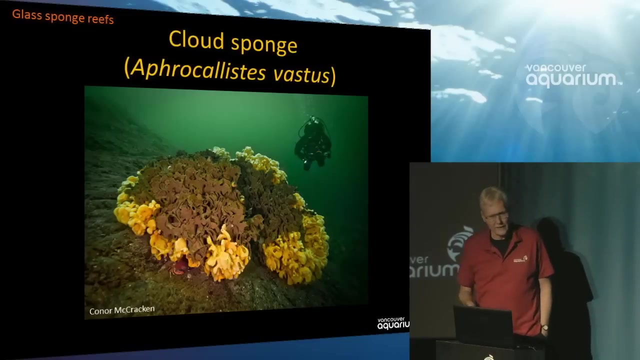 whole thing had died because it was so shallow, and this is about a year later, a little over a year later, and the dark brown is where most of it is dead, and then, around the edges, some of it seemed to survive and recover and actually started growing fairly rapidly, because 2010-2011 we had a La Nina, a cold period, so this 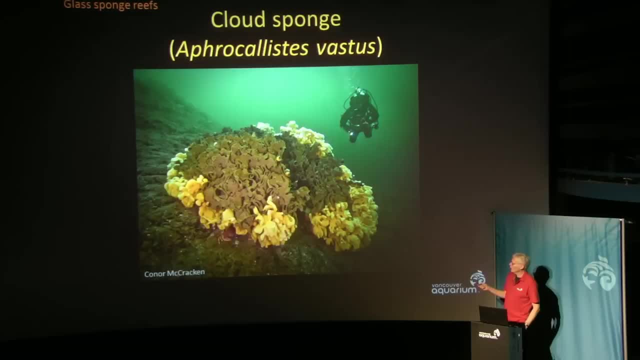 is the beginning of the cold period and, please note, there's a juvenile quillback rockfish right there, there's one here, one peeking over the top here and there's one up right here, and so these sponges are a very important nursery for juvenile quillback rockfish, a species 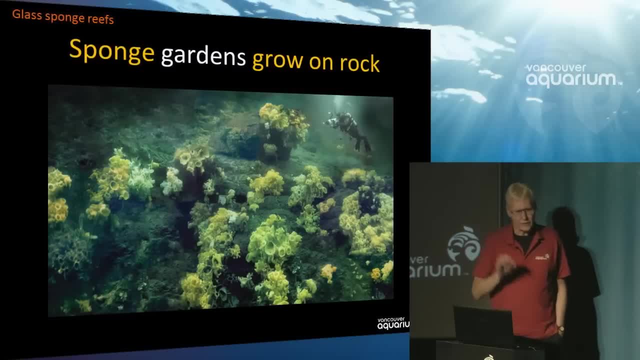 listed as threatened. now, if the cloud sponges are growing on rocks on a cliff like this rather well-known Cliff at Texada Island- it's called a sponge garden and lots of baby quillback and yellow eye rockfish will settle into the area around the sponges. they hide inside the cloud sponges and then 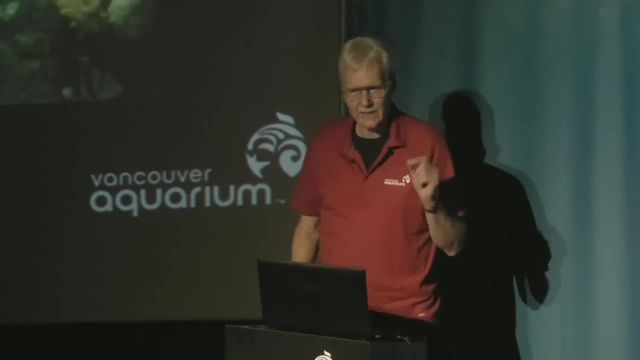 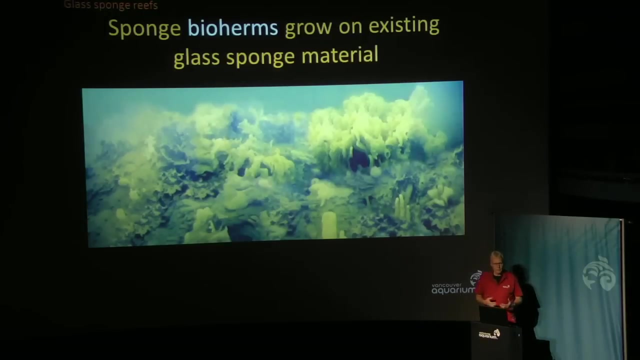 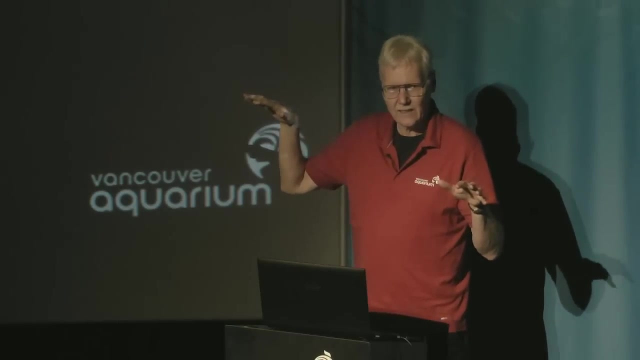 they're out on the rock community finding all kinds of tiny little animals that they can feed upon. if the cloud sponges are growing on dead bodies of other cloud sponges, previous cloud sponges, then that is a sponge Reef or biohorm. so glass sponge reefs are built up on silted in skeletons. 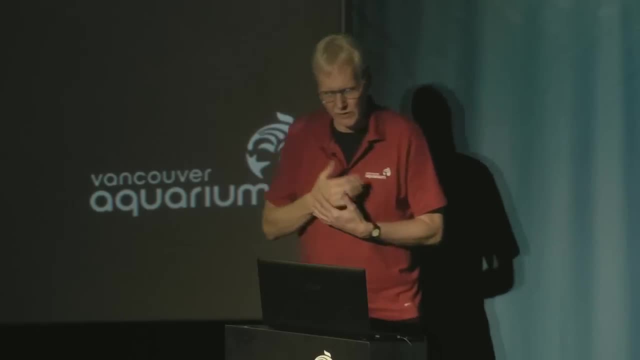 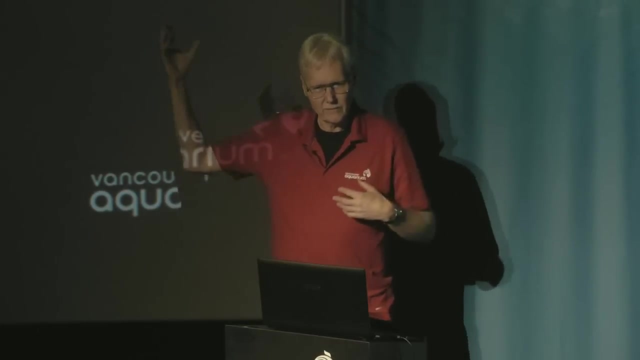 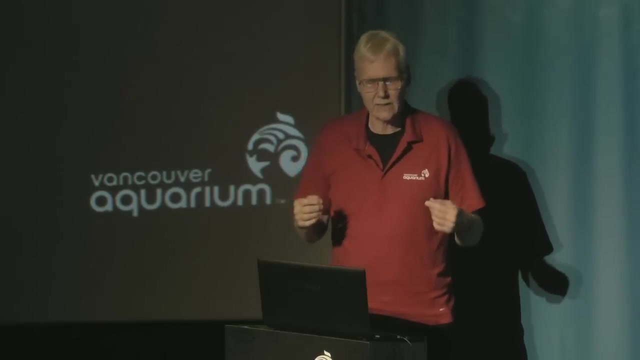 of previous glass sponges and those silted in skeletons become geologically stable. so the geology of mountains, including the Pyrenees in the Alps, includes this chalk-like substrate that was once glass sponge, reef and and in ancient times, the biggest, largest living land form in the history of the. 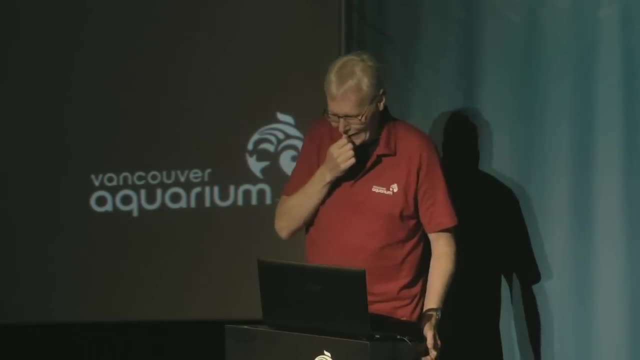 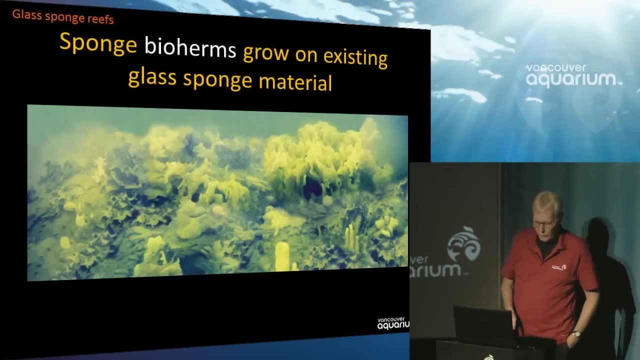 Earth was a glass sponge reef that spread all across Europe and it was thought that they had all gone extinct during the Jurassic until just a couple decades ago, when they were found in British Columbia- and the sponge reefs only occur in British Columbia, and actually this picture here is 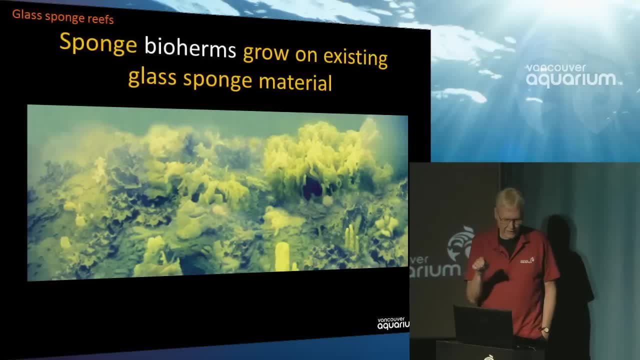 photo mural is a collage of snapshots that Donna and I took in-house sound reef that's shallow enough to dive on, and in all of British Columbia, the only place we know where you can actually dive on these sponge reefs is in Howe Sound. So this is what it's like. 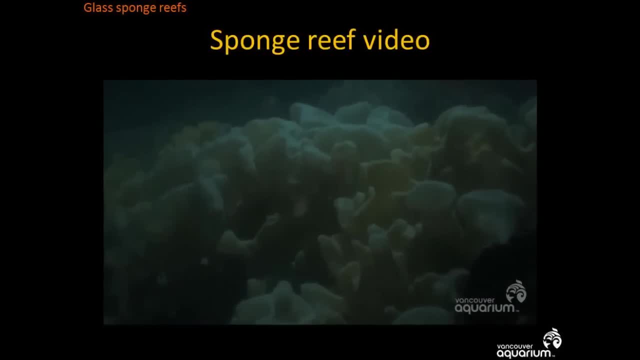 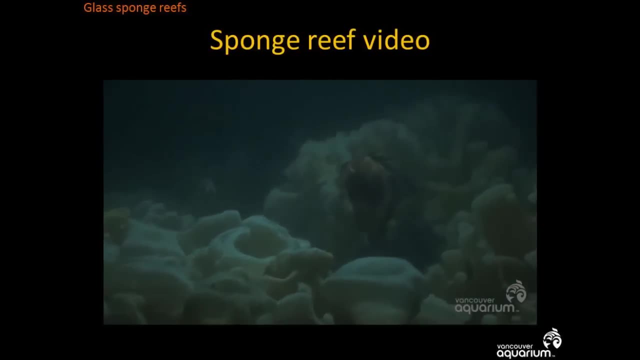 This is a dive that Jessica and Donna took on a sponge reef at the entrance to Howe Sound, and the second diver, Donna, was providing the lighting and it makes it a little more spooky- No bright lights right at the camera- but it gives you a feeling for what it's like. 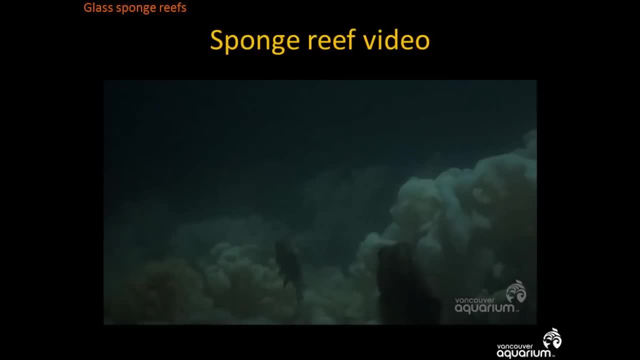 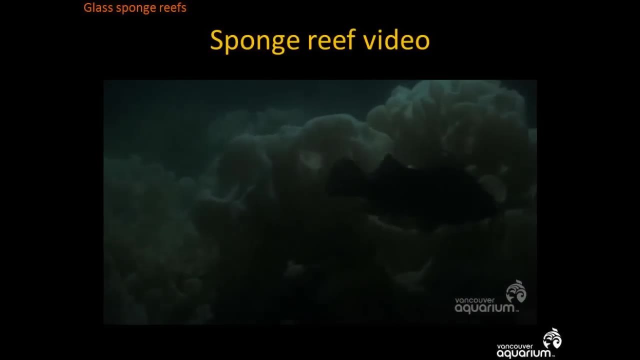 This was in broad daylight, but no light gets down to the reef because of the plankton bloom and you can see these broodstock quillback rockfish that have already given birth by this time of the season, but good numbers of them taking refuge in the cloud sponge. 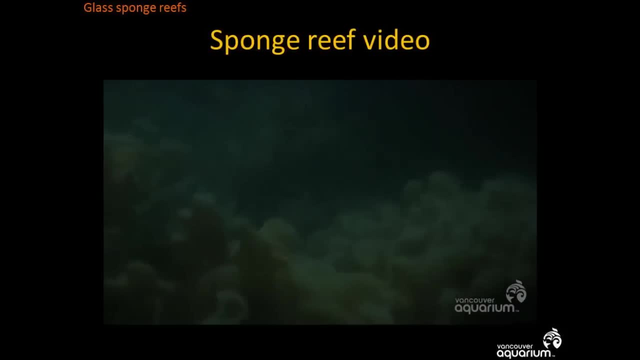 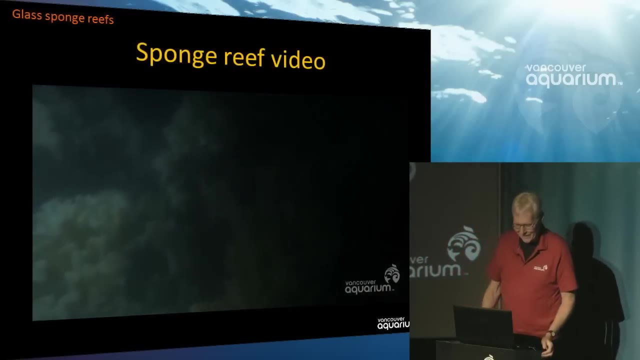 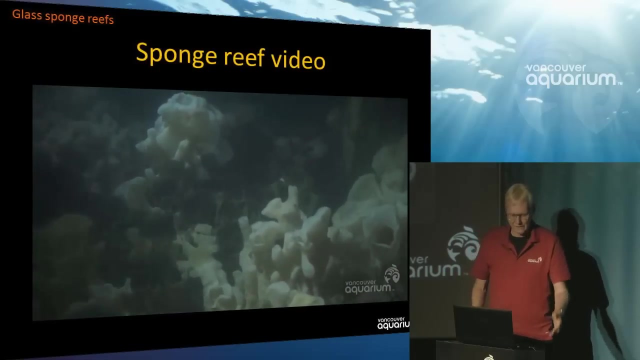 reef and Donna was talking earlier about the. I want you to know it was an English soul that they found on their way to the bioherm and when they get there they still don't really know how big the glass sponge reef is, what its extent is, how far it's going. 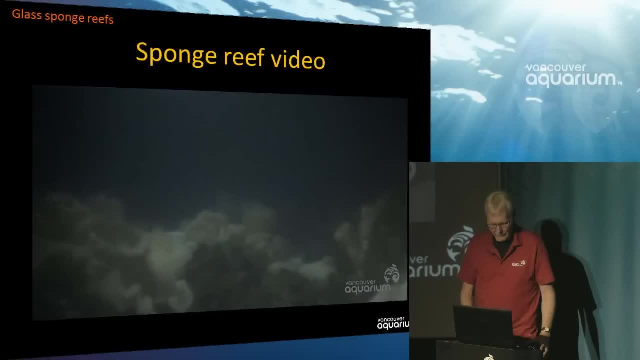 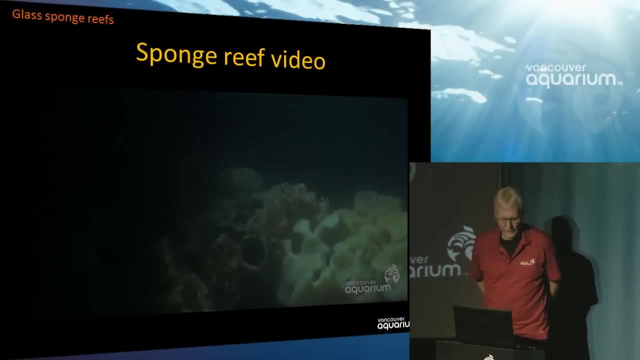 and where it goes, and that's part of the mystery of diving on these glass sponge reefs, but they're very convoluted and so where you would have had just smooth glaciated rock, you have this very complicated structure that provides a lot of refuge for certain types. 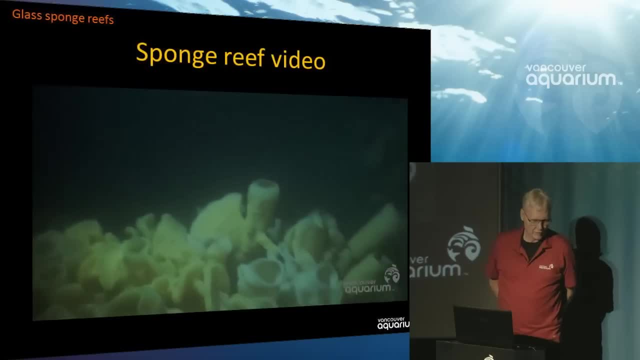 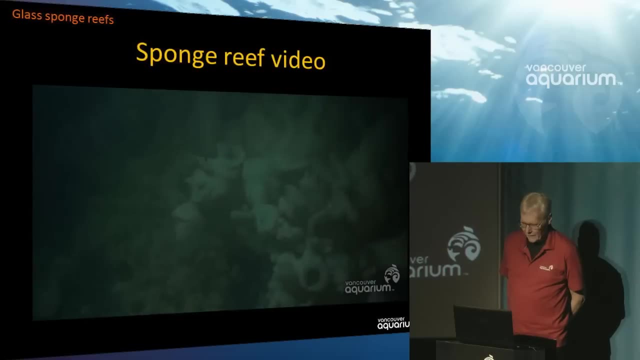 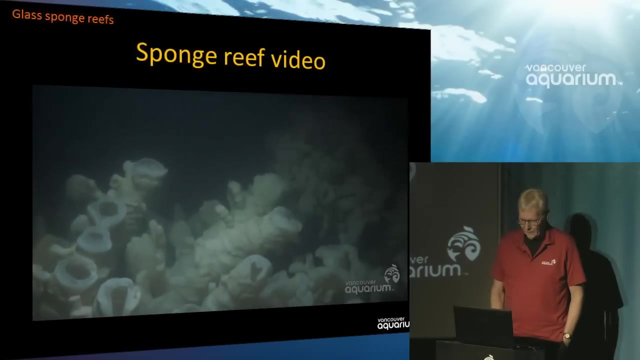 of animals, which include rockfishes and the squat lobsters. you saw in an earlier photograph any number of crustaceans, But it's It's only possible to dive on compressed air, in-house sound and see this type of reef structure. so it's something that we have specially available to us and we're 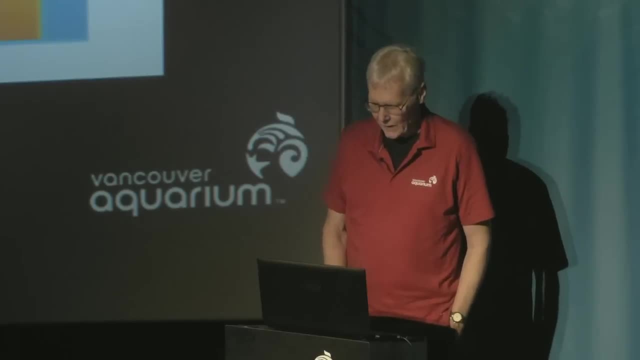 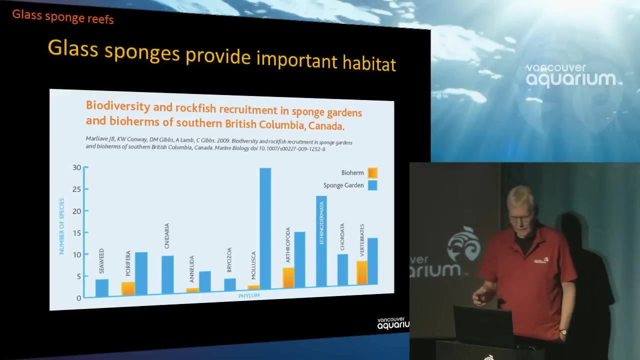 very, very pleased to be able to do that. Now, looking at the seabed biodiversity records that Donna has amassed through various dives in areas with sponge gardens and bioherms, it actually turns out that where the baby rockfish settle and grow in their nursery stages, on the sponge gardens, which are the 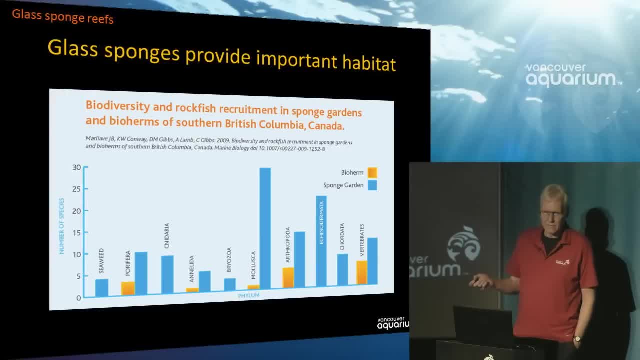 blue bars have a huge biodiversity and that's for the most part because of all the different types of plants and animals that live on the rocks around the glass sponges, whereas on the bioherm or the sponge reef really you have fish and you have shrimps and crabs on. 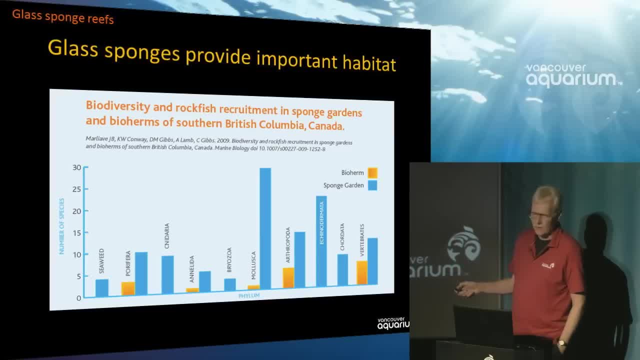 the sponges and you've got sponges, periphera, and there's one type of worm that lives on the mud at the base, At the base of these sponges, and there's one type of nudibranch or sea slug that lives. 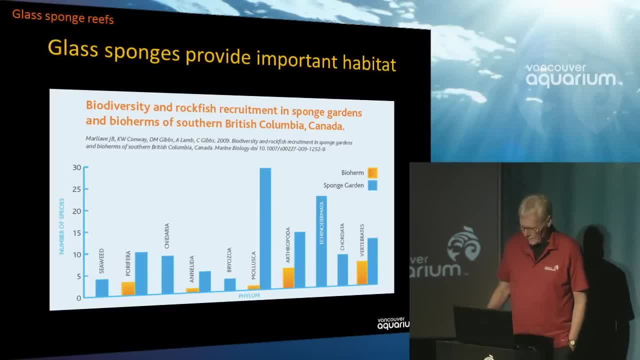 similarly at the base of the living part of the bioherm, But it actually has much less biodiversity, and so it's actually not good nursery habitat. What it is is a good grow out for rockfish, and it's when a quillback rockfish gets big. 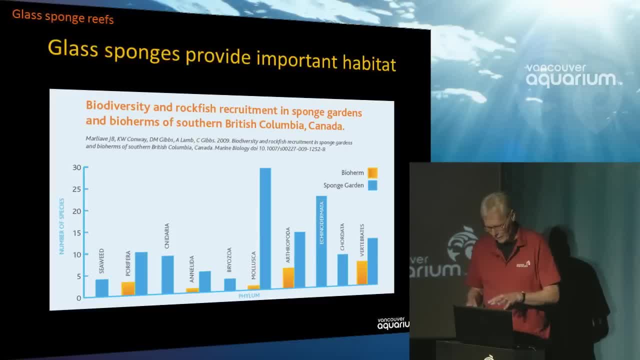 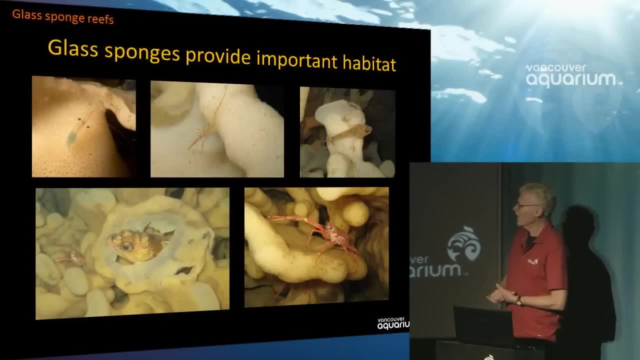 enough to eat those squat lobsters. then they move on to the bioherm and very typically there are sponge gardens Immediately adjacent to sponge reefs. So it's very important as habitat and I want you to take note that this little, this growing, 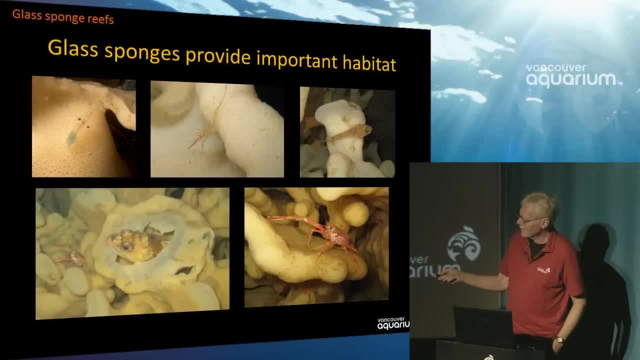 quillback sticking inside the sponge is causing a bit of physical damage to the cloud sponge. They're very delicate growths and the squat lobsters of course are very important food for the quillback. We don't know if some of these shrimp get eaten by rockfish. 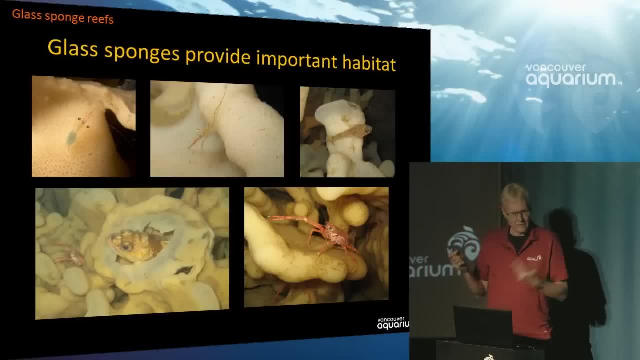 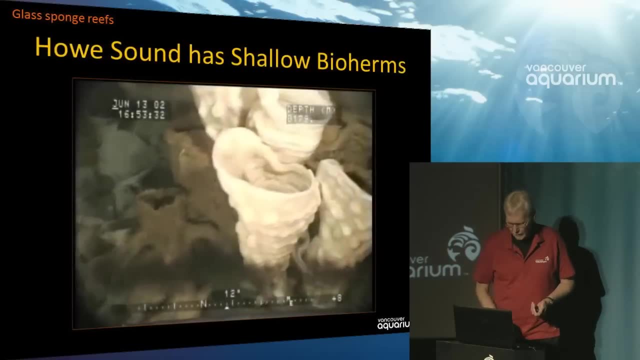 There's one type of shrimp that is not really named, and it's a sponge. It's a sponge reef shrimp. It doesn't live anywhere else, So there are still lots of things we have to figure out. Now, what's so special about being able to dive on a bioherm? 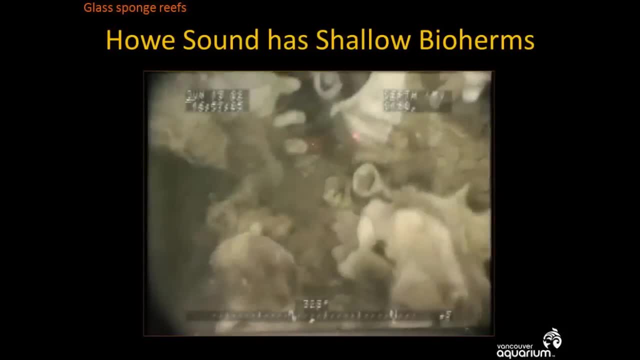 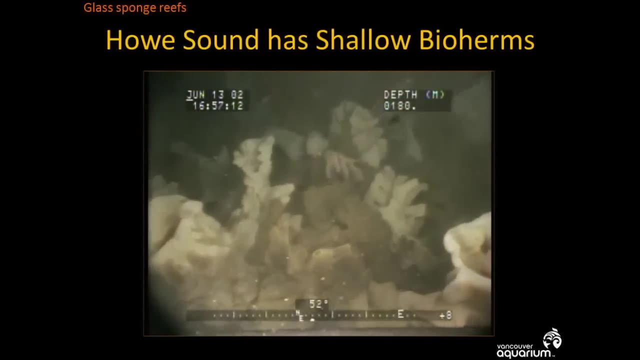 What's the big deal? Well, they're mostly in very deep water in British Columbia, so you have to send down a remotely operated vehicle, which means a little mini submarine with a video camera in it, tethered to a ship where an operator is operating it like a video game, and we 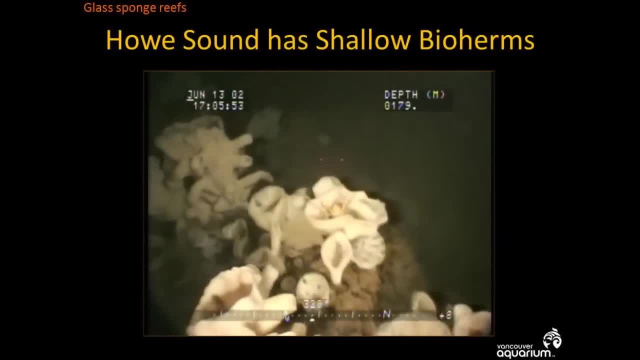 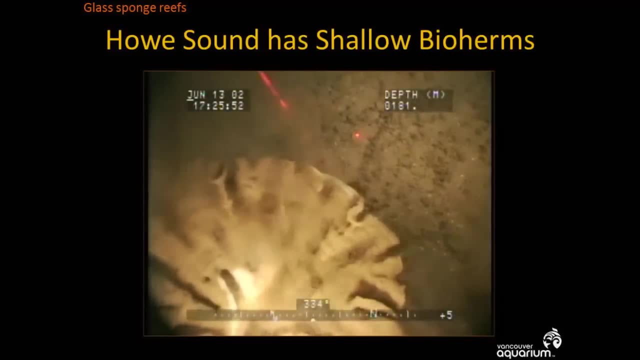 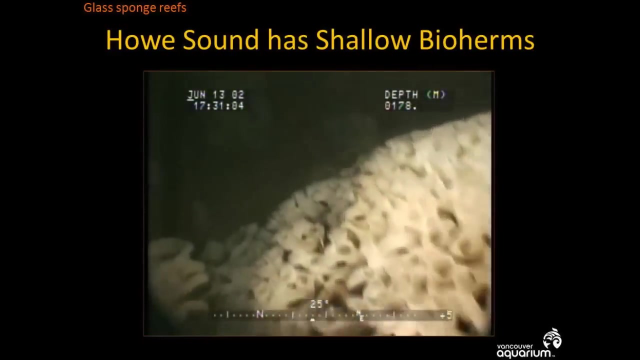 think that divers can be a little less clumsy than a remote vehicle, Which can cause damage, And so that's one of the beauties of being able to study them in-house sound, that we're not doing this level of damage. This is, for Ria Aka, by the way, a type of very delicate cloud sponge that does not live. 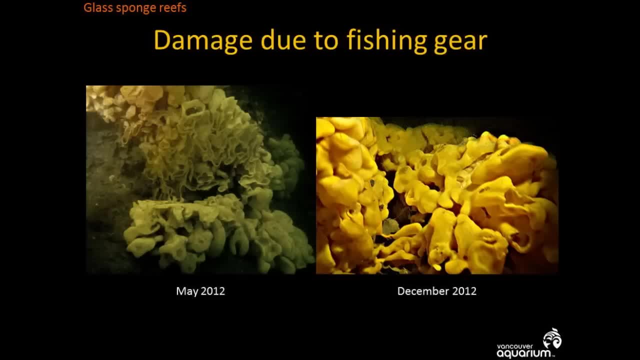 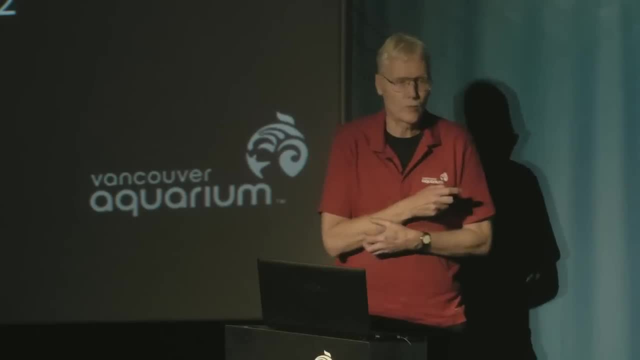 in BC And that's a vase sponge in that last shot. So that was kind of a cruel comparison showing that footage. But fishing gear causes a great deal of damage to cloud sponges. My cocktail party Story is that, oh, these cloud sponges have the same structural rigidity as a meringue. 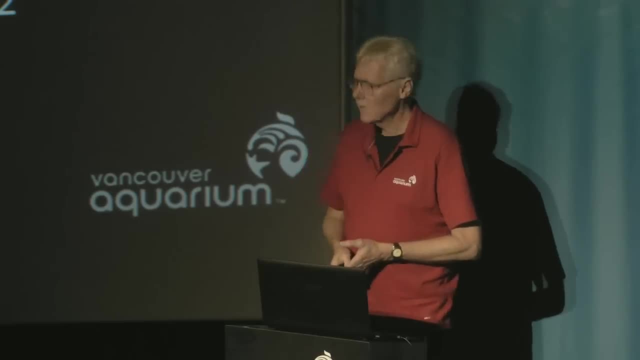 fresh out of the oven, You flick it and it's going to shatter. So in May of 2012,, we were very upset. That same big sponge that had been hit by the El Nino and that was recovering got sliced. 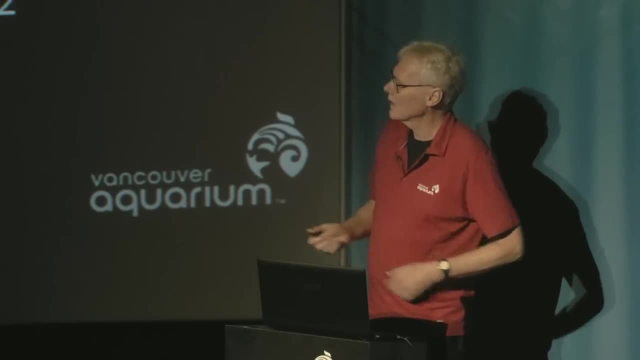 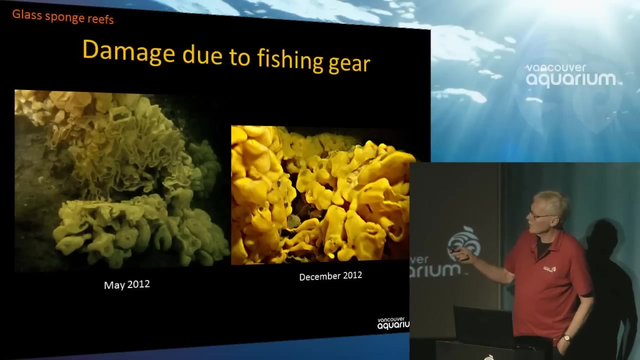 It just got sliced in half by a downrigger line And over on the left. this is the slice, Just like a cheese wire cutting it through, and you can see the internal structure. and this part had folded down. I was worried that it was going to become dislodged. 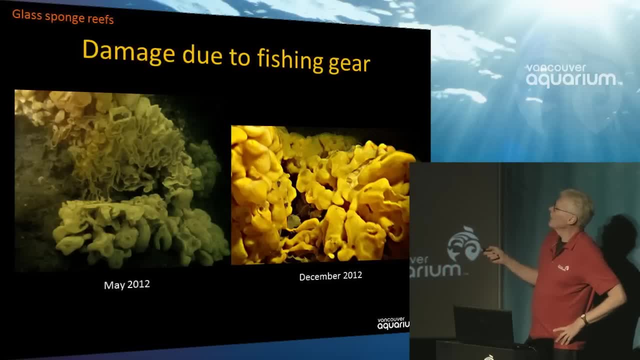 But in fact by the end of the year it was still lying there and the cut-open parts were heeling over. There's no glass spicule architecture inside these narrow heeled spots that can have sort of a spiderweb lacy appearance. 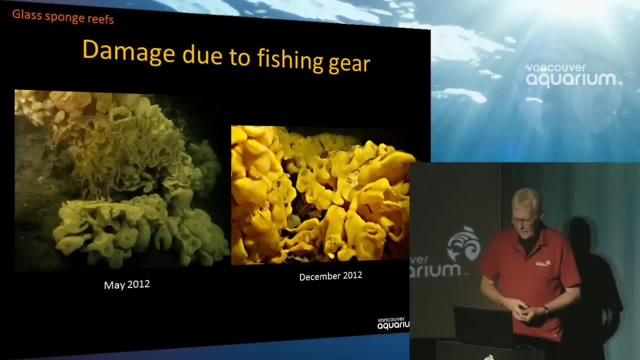 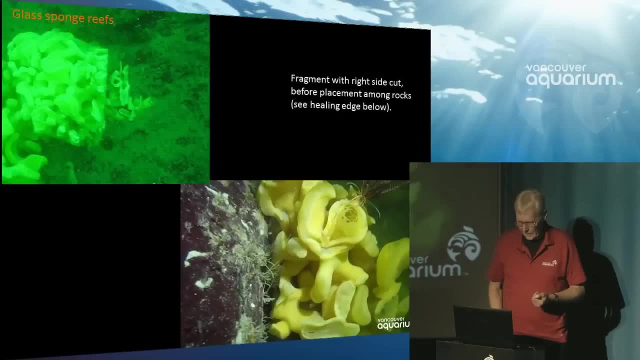 They can actually open and close in the space of a day, But this is La Nina. weather here: It's very cold, And this is La Nina, And there was tissue repair going on Now at the time of this incident. we were upset to see it. 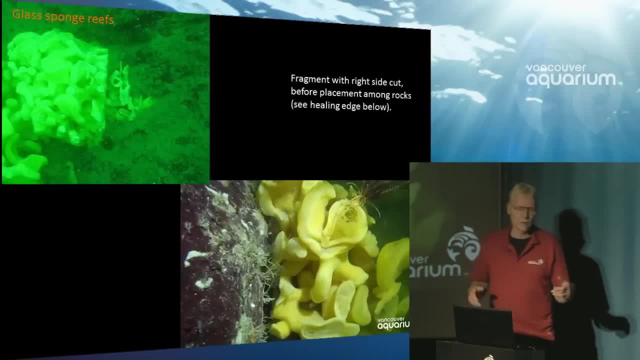 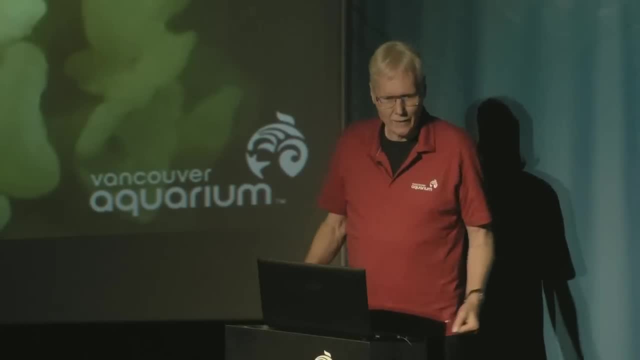 We were really upset And we wanted to do a blog posting about it and we were told: no, you have to have something on display if we're going to talk about it. So we went back and we were going to bag one of the fragments. 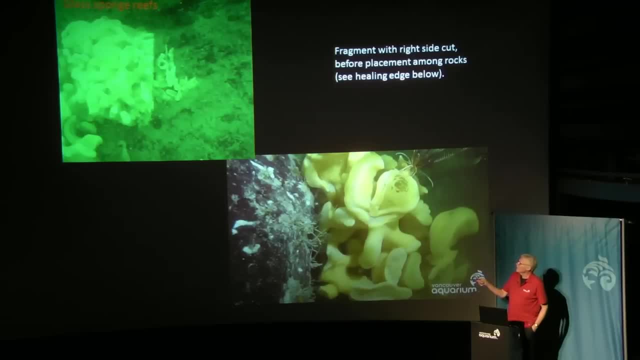 And over on the upper right. this is a piece that was. that's where it was cut off and it's lying against a full-living piece. Okay, Cloud sponge down in deeper water And we couldn't get the bag over it. 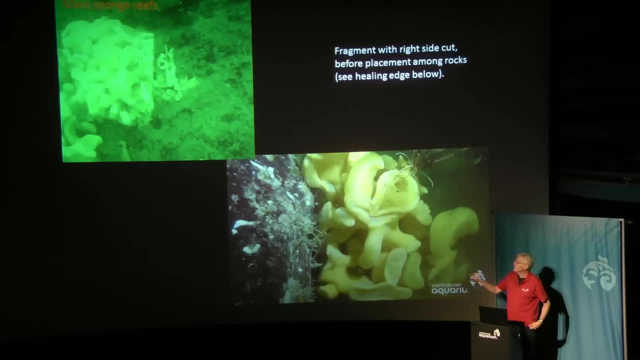 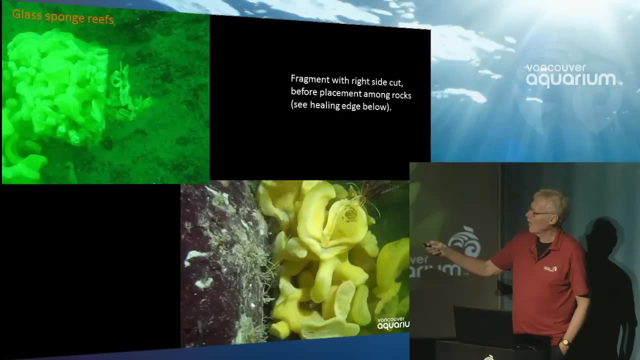 Donna was. I was stretching the bag and Donna was looking at it, And so she hesitated, took out her dive knife and made a big slice. parallel to this slice, And all of the good outer morphology on this side went on display. 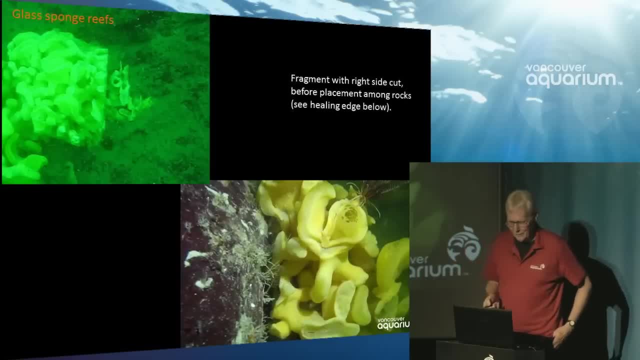 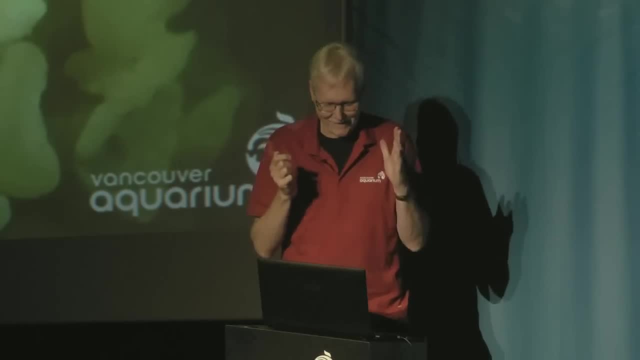 And we posted our blog narrative about the damage that can be done. But at the time that we got the piece bagged I looked at this giant Texas toast slice of cut cloud sponge and my heart was breaking over. what can we do? what can we do? 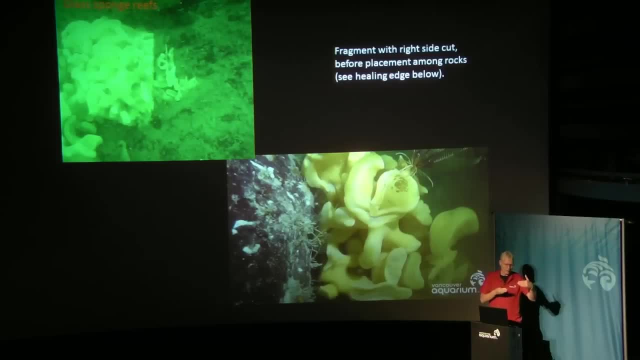 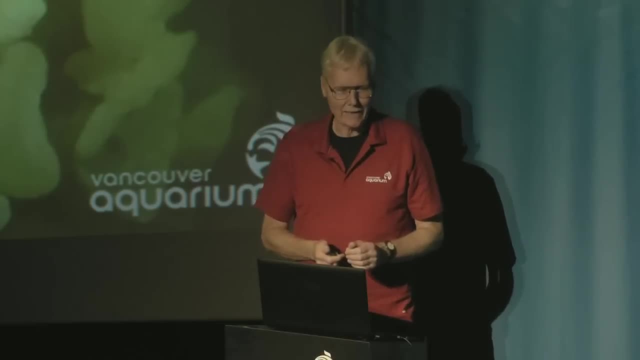 So big. I gently picked it up, looked around and there were two big rocks at right angles on a downhill slope, And I sort of tucked it in on the uphill side and thought, oh, that'll be good. We went back and saw, oh, it had wafted away, and so I got on my knees and I walked a couple. 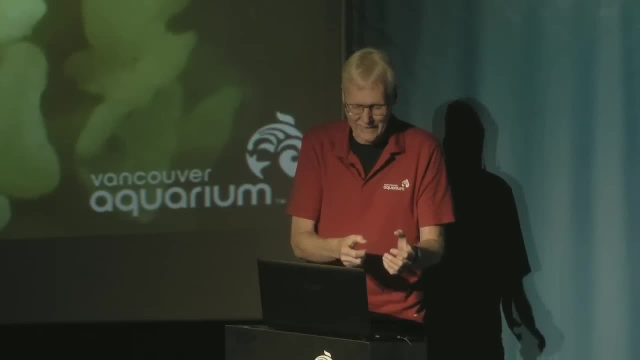 more rocks over And as soon as I would touch the sponge it would start shattering. so I just got it as close as I could, without quite touching, so that it was stuck in place, had about a millimeter of wiggle room. 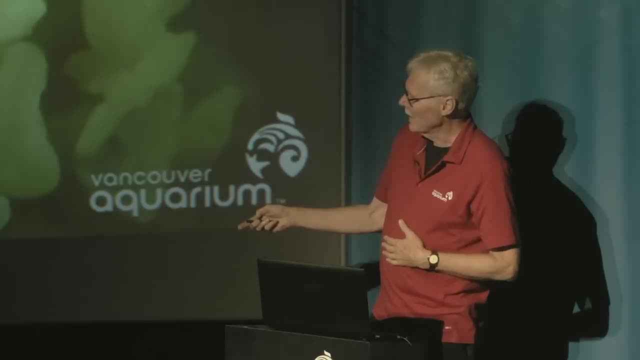 And so that's May of 2012.. And this is December, and this is part of one of the slices And you can see that it's healing over everywhere it was sliced and it's getting better. And this is another. this is a break that's healing over. 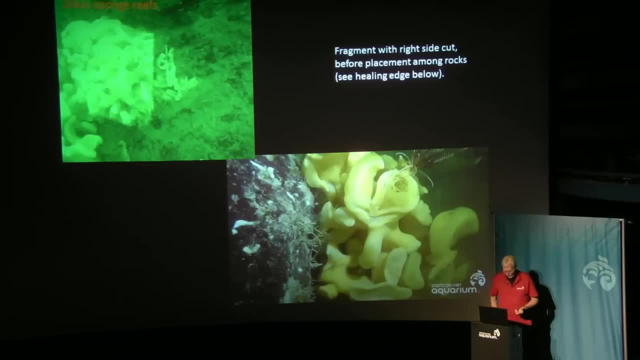 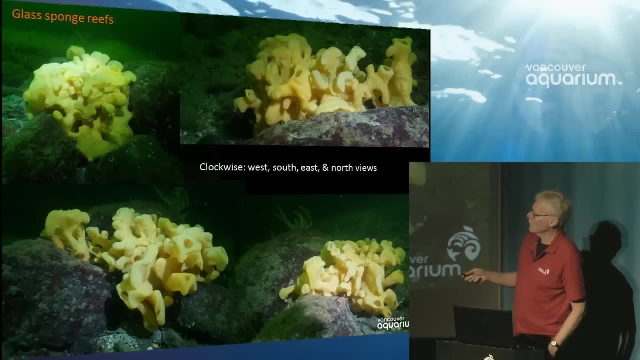 And so we were very interested in that, And at this point in time, two years later, I'm going to take you for a little tour of this fragment- Actually, it's a series of fragments, because there are a couple of loose pieces that were. 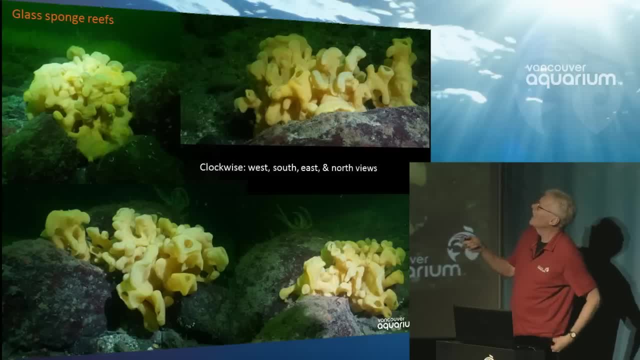 being crushed in my hands And I tucked them down in a loose spot And from going clockwise. this is the view from the west and you can actually see where it's touching the rock and, like buttress roots from a tree, it is fused. 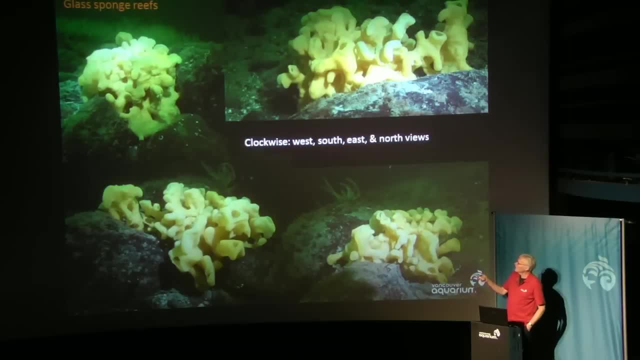 Everywhere it's touching it is fused to the rock. And then this is looking from the south. this is the biggest rock and that's where I was looking down in that other shot, where it was healing. And then from the east, these were loose pieces and they have. 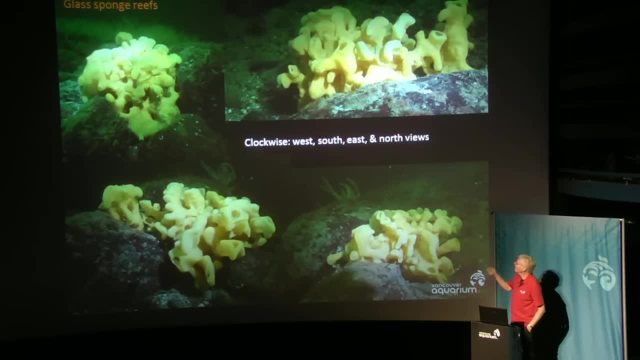 No, excuse me, Here I'm going clockwise. So this one right here. these were the loose pieces that have grown together and it's now growing out from the rocks that I had placed. These are the two rocks that were the big rocks and it's now looking like a nice little. 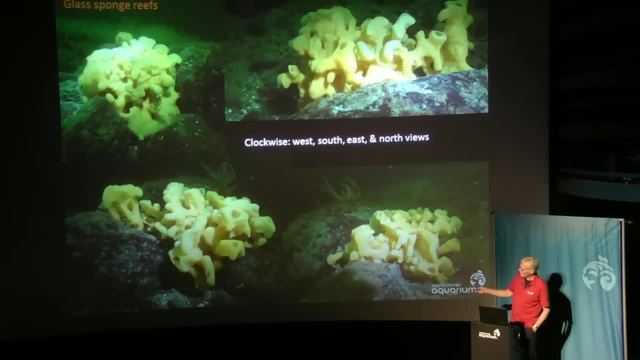 cloud sponge, And this is getting to a view from the north and you can see that it's sticking out from little rocks that I placed and bigger rocks, And so it's doing really well. but yippee, We put it there and it showed that it has the ability to reattach to rock. But in nature the odds are probably vanishingly small that a shard would fall down into a perfect fit so it wouldn't wiggle around and wouldn't get battered. When we've seen fishing gear damage in other cases, we've just seen it all deteriorate. 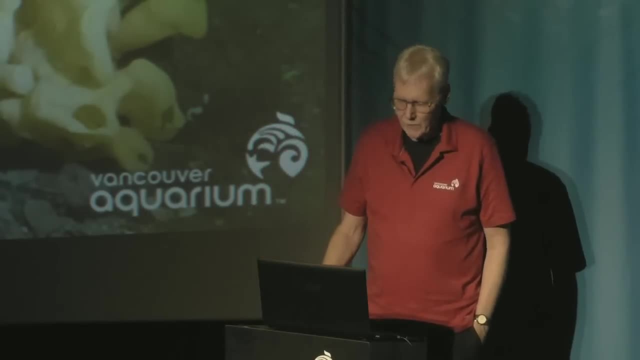 get swept away, and it dies quickly. The one exception, though, might be on these glass sponge reefs, where all these arms are coming out, and I've failed to mention this. is all one cell Like. it's so primitive. It doesn't have cell walls, so there's no tissue compatibility problem. 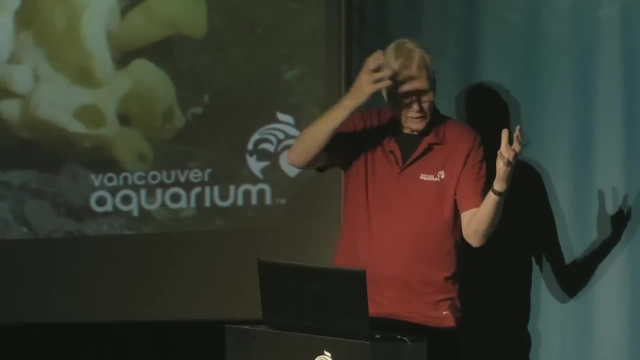 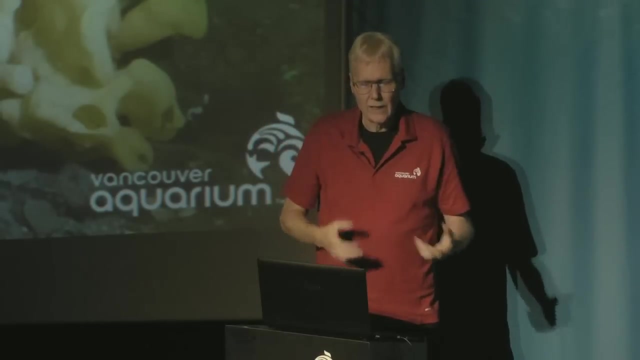 And if a living arm gets broken off on a glass sponge reef and it comes to rest on other arms of living cloud sponge, it probably can fuse and continue to grow, And so we've seen a lot of evidence of breakage resulting in subsequent growth on the one. 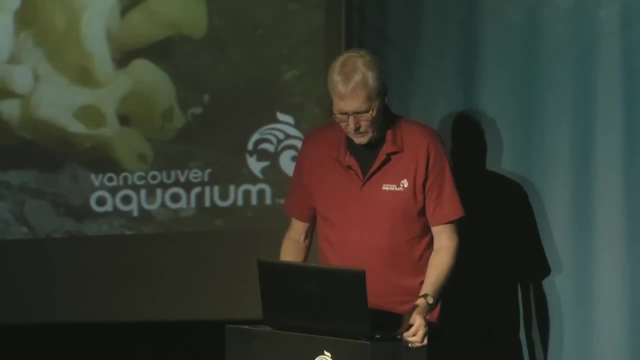 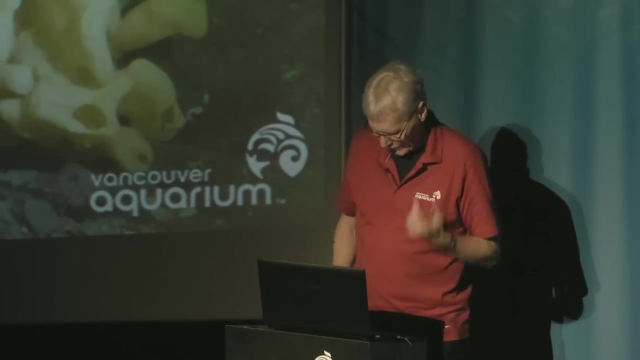 reef that we've been studying And it's very likely, from what we see on a drop camera, that where there's damage by fishing gear, If there's damage, these sponges struggle to fight back and earn a living, even in the presence of humanity. 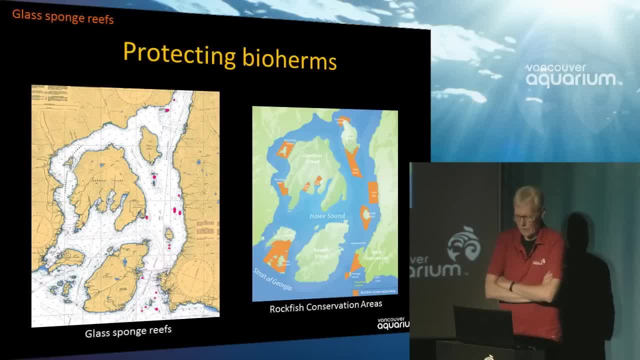 So I want to talk about protecting these sponge reefs or bioherms. Now I have actually made a presentation with those taxonomic data and such and argued up in Alaska that since hook and line fishing is not allowed in rockfish conservation areas, these areas in orange 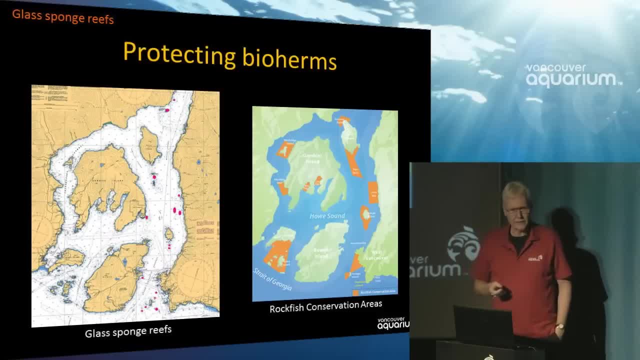 In order to protect rockfish, there should not be other deleterious impact on rockfishes in those rockfish conservation areas. And because it's not a hook and line gear, prawn trapping is allowed inside the rockfish conservation areas. So my argument was: either the prawn fishery should adopt a code of practice, so they will. 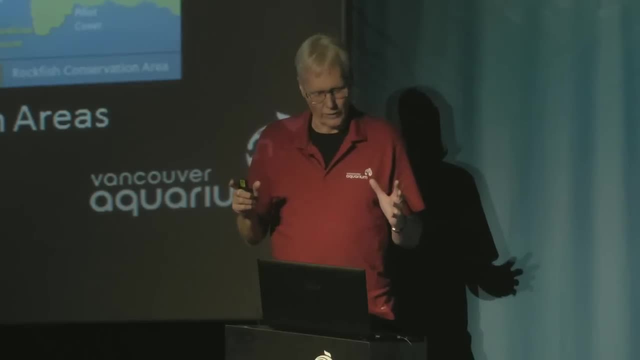 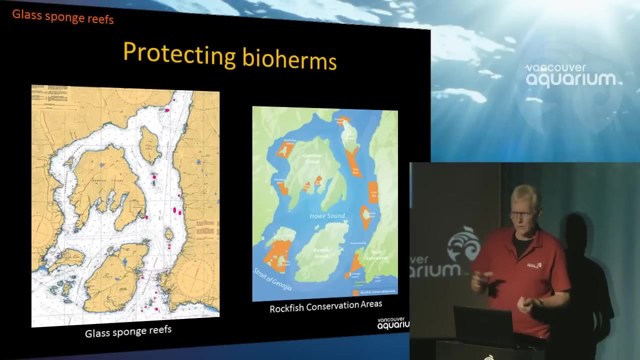 avoid sponge gardens and sponge reefs, or they should not be allowed inside rockfish conservation areas because they are damaging. Now This is a really strenuous case to make, because between 25 and 33 percent of British Columbia's known rock reef substrate is inside rockfish conservation areas, and that would be a serious 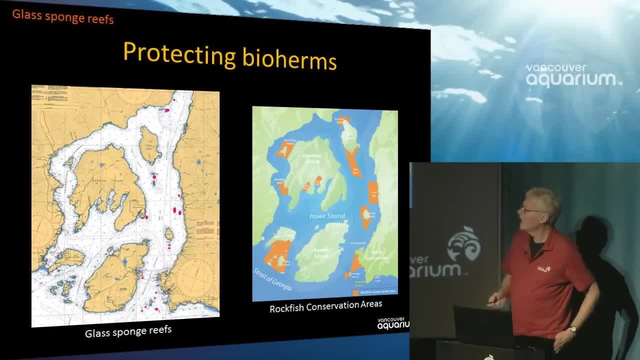 economic damage to the fishery. The reefs themselves are not nearly as great a spatial area and they could be avoided. Now. the pink dots represent known sponge reefs in the House Sound. They're being found fairly rapidly by Citizen Science, a fellow who operates a drift. 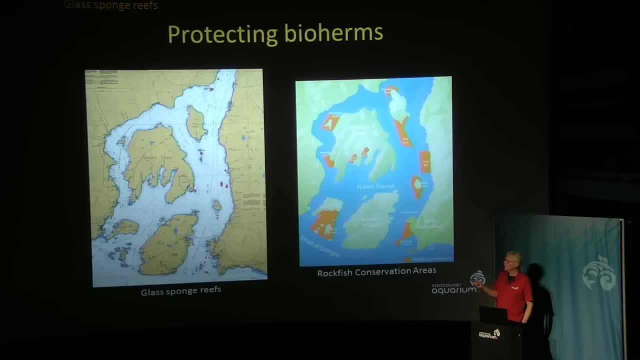 drop camera right here off this There's a feature coming out off the northeast corner of Anvil Island. Just a few weeks ago they discovered yet another sponge reef. None of these sponge reefs in this part of House Sound are encompassed in the measures. 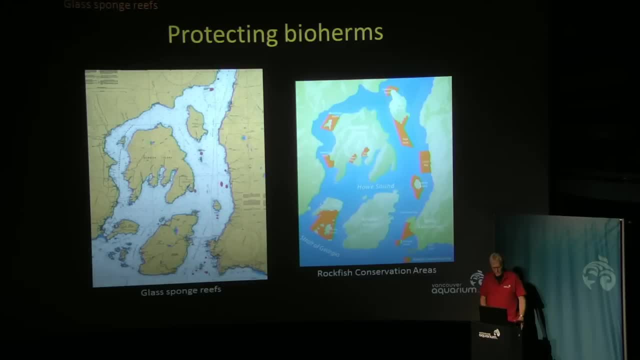 that are coming up to protect sponge reefs in the Strait of Georgia. in terms of federal government policy, These reefs down here are included, And the difference is that In the Strait of Georgia, which is a shallower slope to its seabed, multi-beam imaging could. 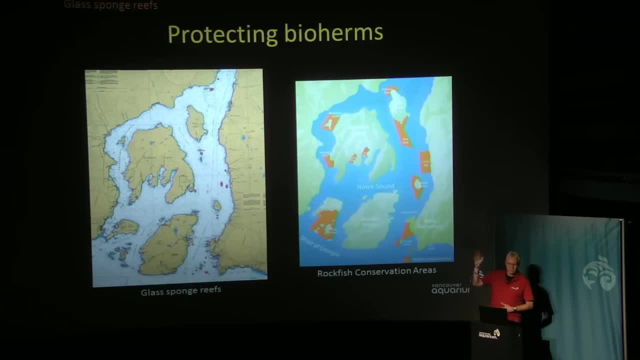 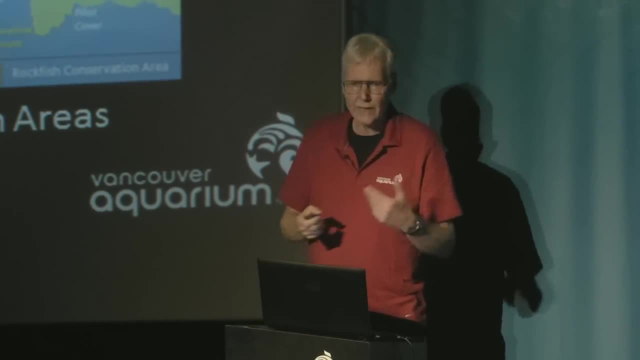 detect the presence of the sponge reefs, But on the steep pinnacle features in the walls. in House Sound the resolution wasn't high enough to reveal the presence of the sponge bioherms, So the indirect method used to indicate where they might be wasn't really adequate for House. 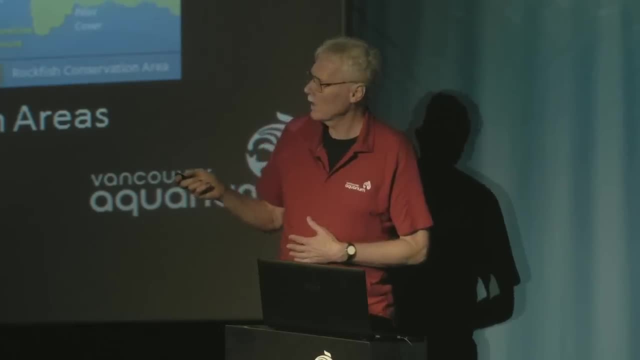 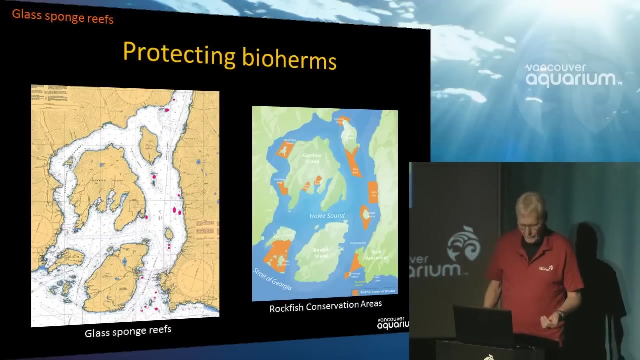 Sound. Now this has us concerned because we know these reefs are here. We know that, for example, off Lyons Bay there's a tremendous amount of prawn fishing, both commercial and sport, And so there's an active effort being made to convince people at the Lyons Bay Marina. 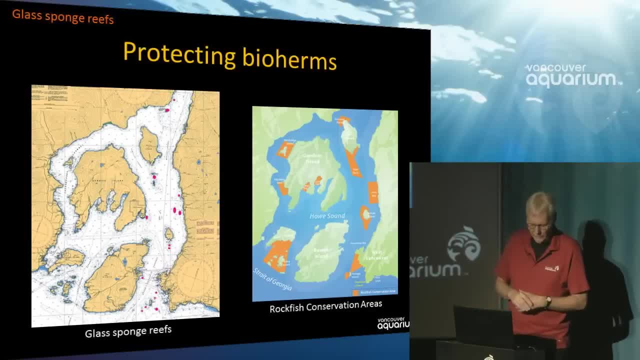 to do their fishing near the shoreline and not on the offshore pinnacles And that seems to be working with the sport people. There's a lot of negotiation going on with the government over these reefs down near Passage Island and White Cliff Park because the live fishery to Granville Island. that 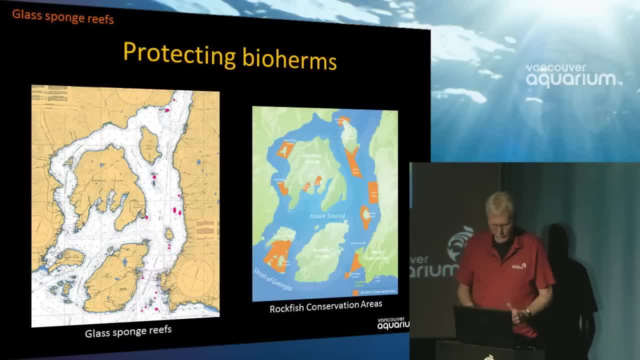 market depends critically on the prawn fleet being able to zoom out and get right back in quickly. So it's a really serious problem And one of the obvious solutions that we think has to do with these diveable reefs. there are only five areas. 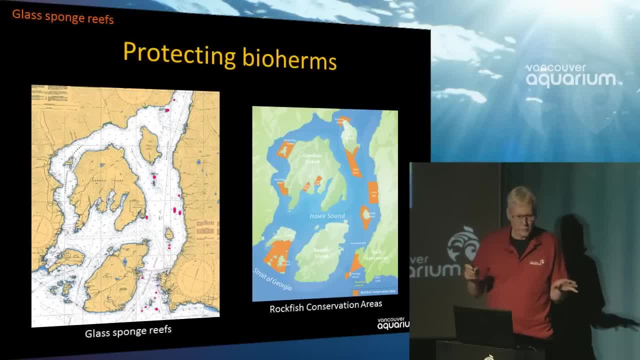 This is one reef off Passage Island. That's the dark, spooky video that Jessica and Donna got. And then this is a diveable reef south of where the ferry's going to Bowen Island, And it starts at 125 feet. Thank you. 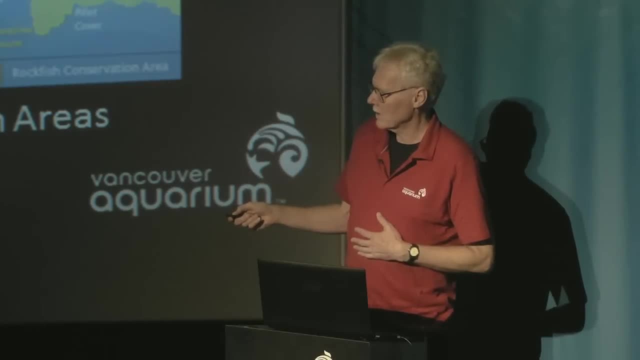 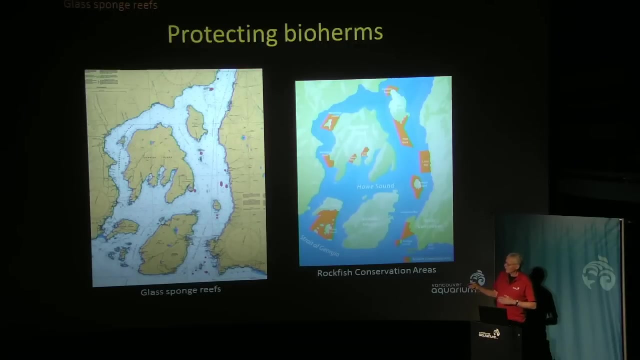 We're not going to go there. That's really deep. This reef starts at about 80 feet. There's a diveable reef that's really nice on a pinnacle off of Halkett Provincial Park. It's a little deeper, It's over 100 feet. 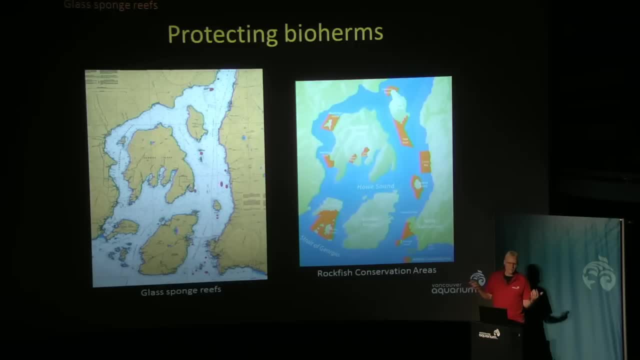 But this is a reef that starts at 125 feet, So we haven't been there. And then, finally, up at the Defense Islands, another set of reefs, two reefs that start at only 80 or 90 feet, And so they're very amenable to study. 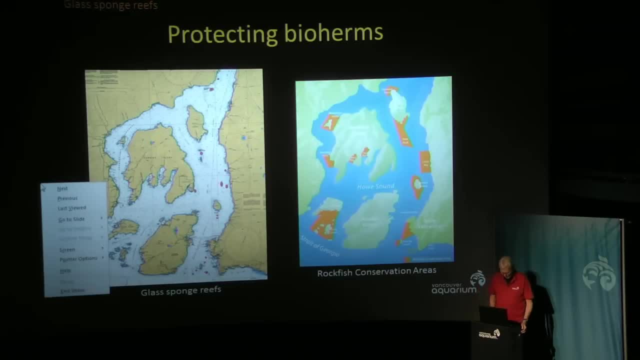 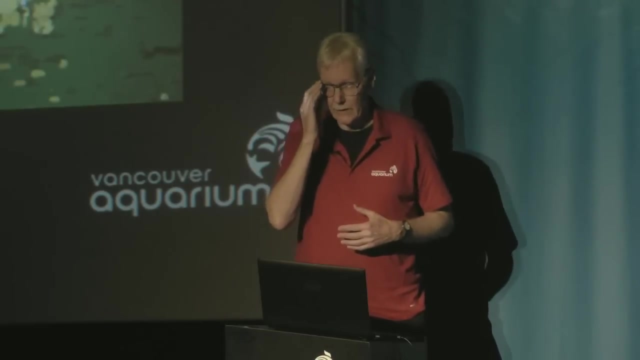 And that's where we've been doing some work And in fact we've decided to go public and to not keep a secret of where the bioherms are and to let the diving public know about them and actually encourage some citizen science. 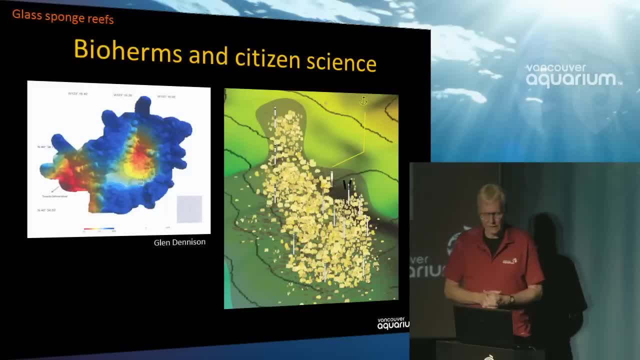 We would like to see how sound become a world destination for diving on these glass sponge reefs. It's the only place you can do it. What I realized looking at videos taken between 2007 and 2013 is that, just like with the, 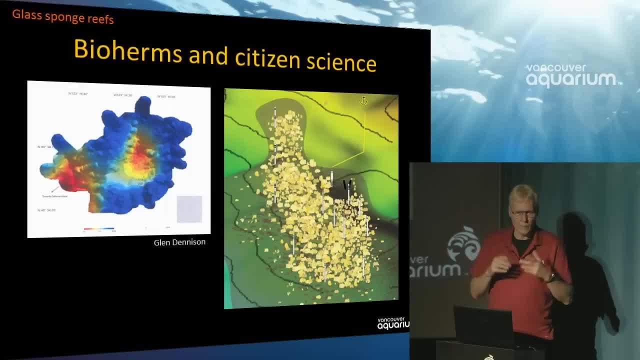 boot sponges. their growth is so amorphous that you really can't identify the sponges from one year to the next just by looking at them. You have to know exactly where you are. So what we've done is- this is a cartoon- of the sponge reef off the near Defense Island. 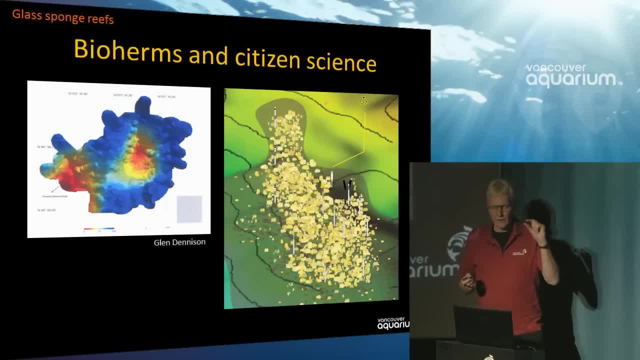 And we've put in stakes with a coating so that we know where each of these stakes is. There are one, two and three black stripes on this series of stakes and three, two and one green stripes, and then one, two and three blue stripes. 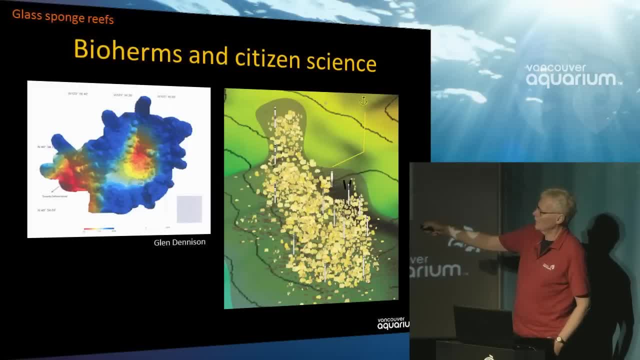 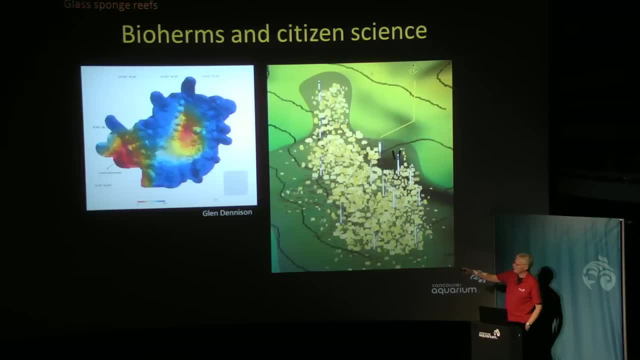 And we anchor the boat up on a rocky reef. This is with north, at the top of the. This is the Defense Island. We anchor on the rocky reef here and then this is the sponge reef. There's another sponge reef out offshore. 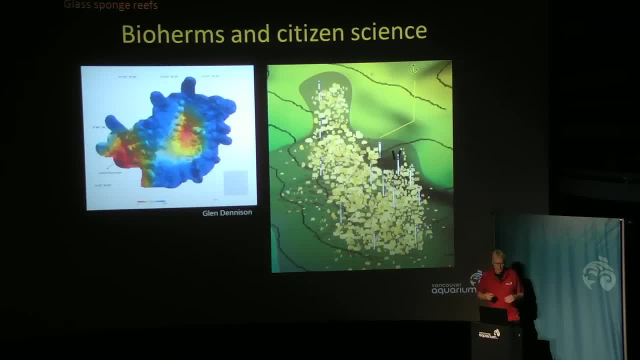 We have a polypropylene line that we follow over sort of no man's land where it's spooky, muddy bottom, usually very dark, And then when we get there we now have a temperature monitoring device there and the original two black stakes pounded in the mud where there had been no sponges but there 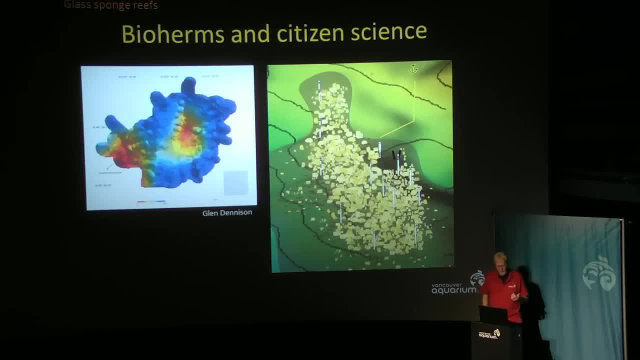 are now sponges growing right around it, probably because we think that during the El Nino that this whole reef kind of got decked like there was a lot of collapse, Some of it tumbled downhill around those black stakes and it seems to be regrowing now. 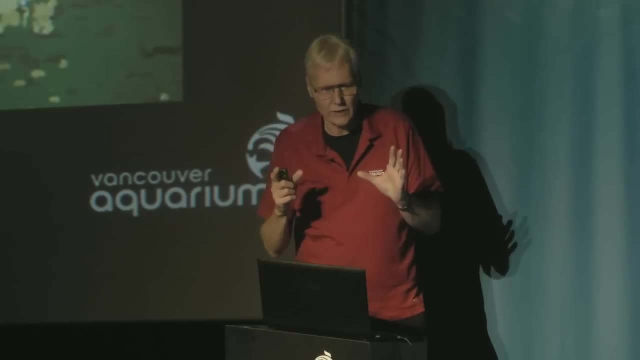 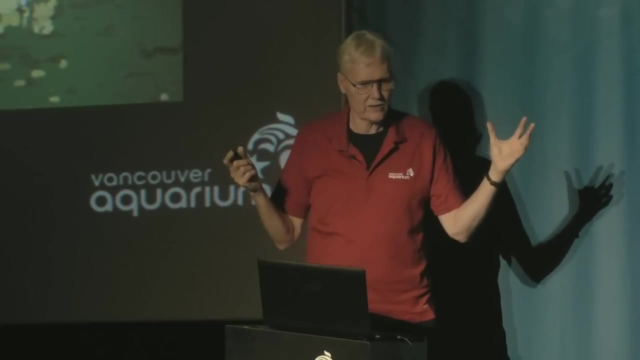 We don't know where we were. We don't know where we were when we shot earlier videotape, but we can look at videotape from 2012 and say, wow. well, those are obviously more than two meters tall and it's just not. 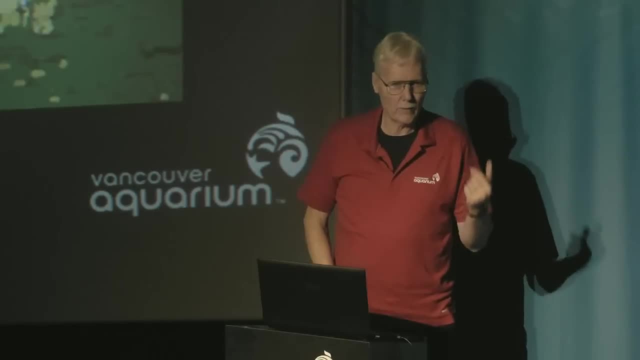 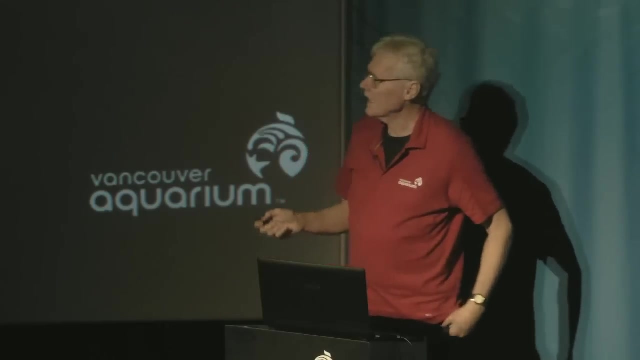 that way anymore, So we can't prove anything about what we were seeing then. Now we've got these stakes in and we're inviting other people to go, and the idea is to go around those perimeter stakes and always keep your fins and your body away from the glass. 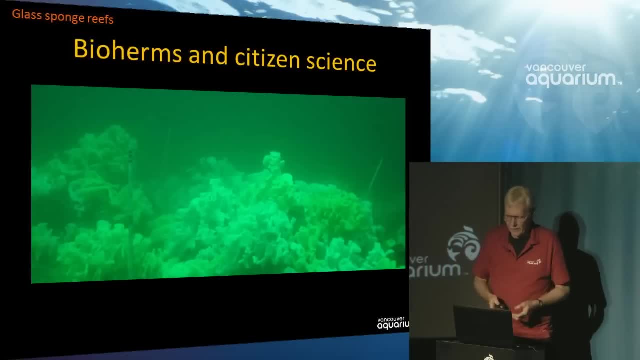 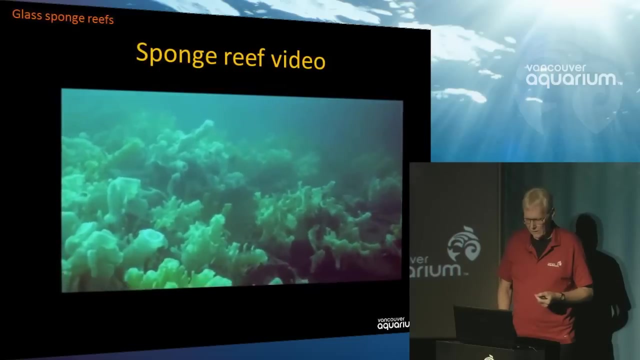 sponges Don't do any damage because, just like fishing gear, if you swim right into them They will shatter. And then always to have the color code of one of the stakes in the frame of your photograph or your video, and then we'll be able to analyze shots over seasons and years. 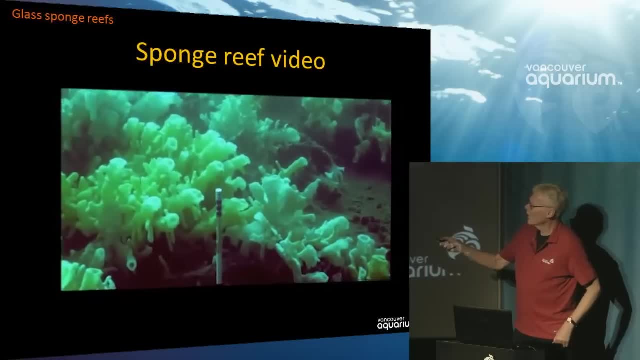 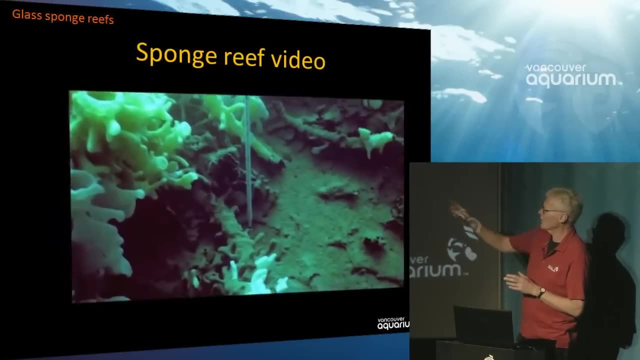 So this is videotape of the three green stripes at the deepest part of this smudge reef. The frame is bouncing around because we've stabilized the video. There's a stripe at the bottom so we can see how deep the mud is and eventually we expect. 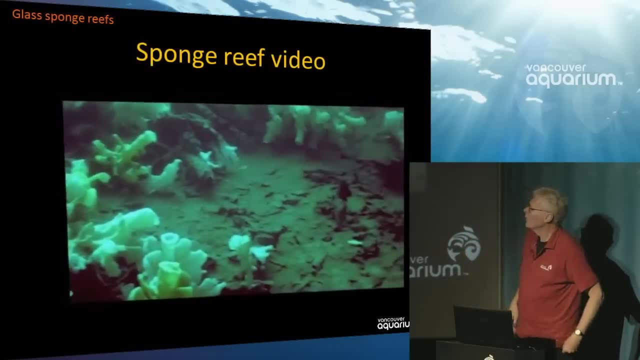 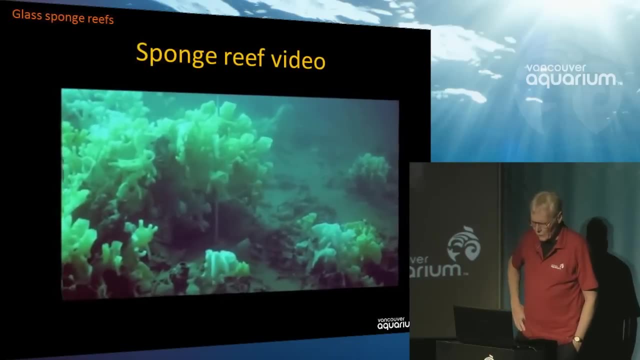 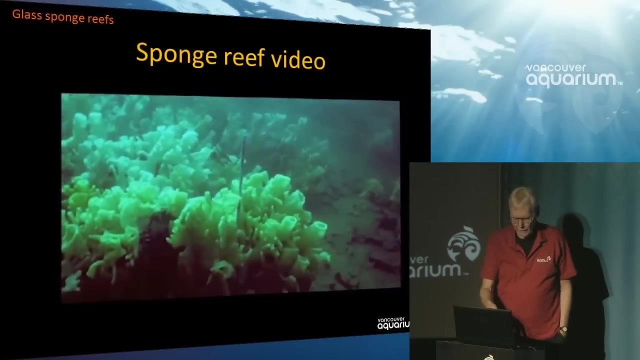 these stakes to bury themselves as the bioherm builds up, collapses, gets sedimented And then swimming over to the next stake with two stripes. we have a landmark in the frame and we're getting an idea of the relative height of the sponges compared to the stake. 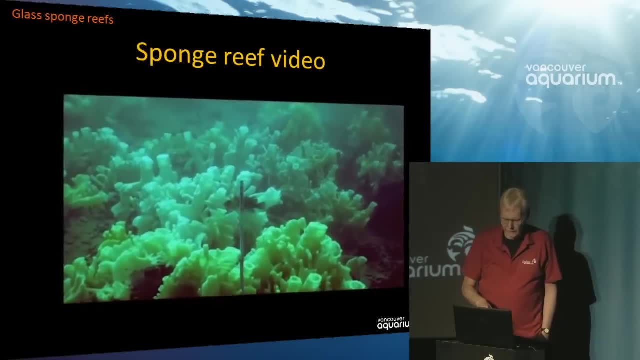 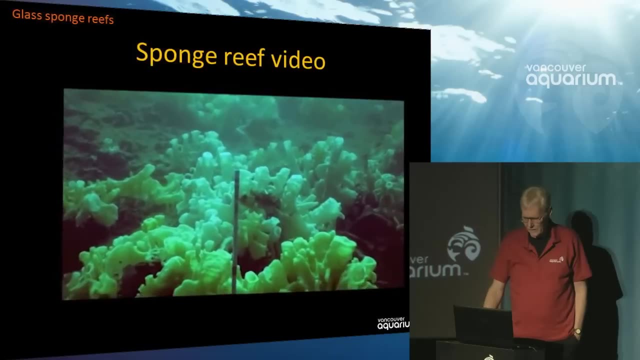 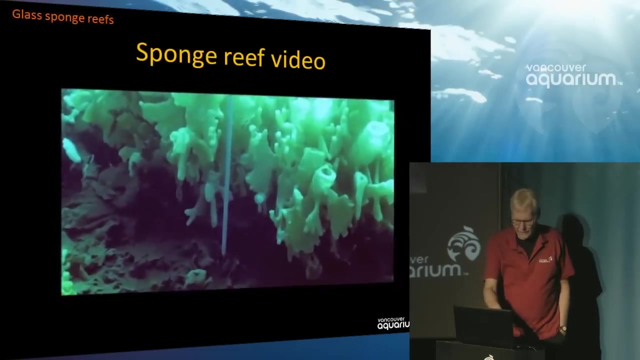 and you get a sense of perspective looking in the distance. This happened to be full sun and clear sea water, So no need for scuba. We actually had our sense of orientation in this particular rare bit of video footage. Usually it doesn't have such good conditions, but down here you can see small sponges near 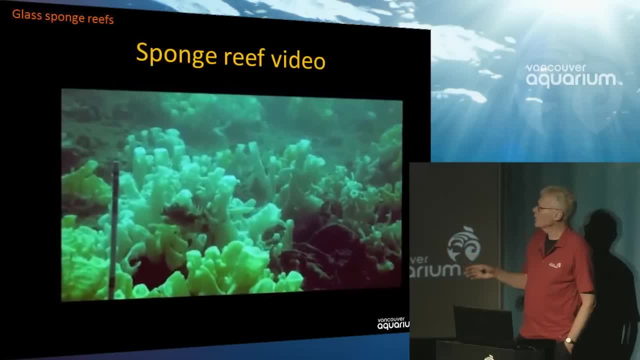 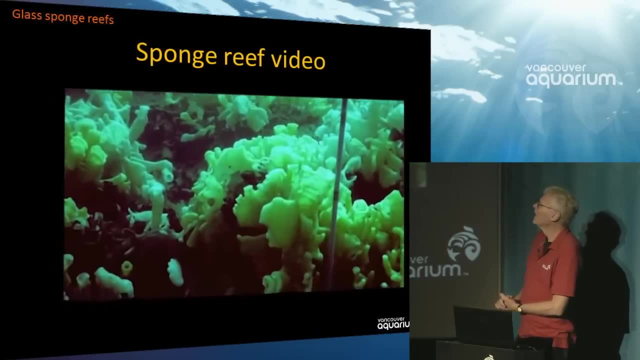 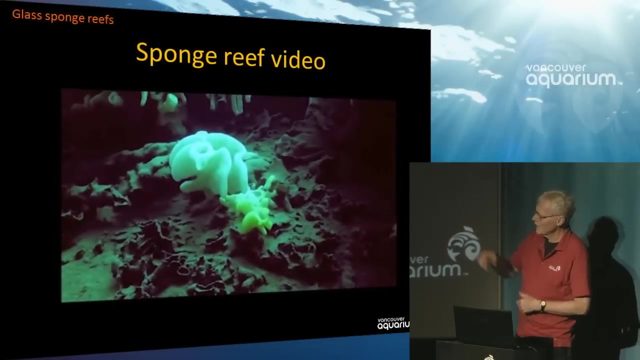 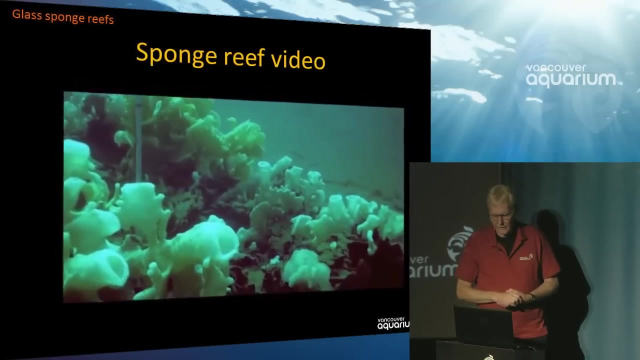 the stake so we'll be able to look at them in the future and gauge their rate of growth. And the camera panning down, keeping the stake in view, and then you see small sponges near the base of the stake And we'll be able to gauge the rate of growth. 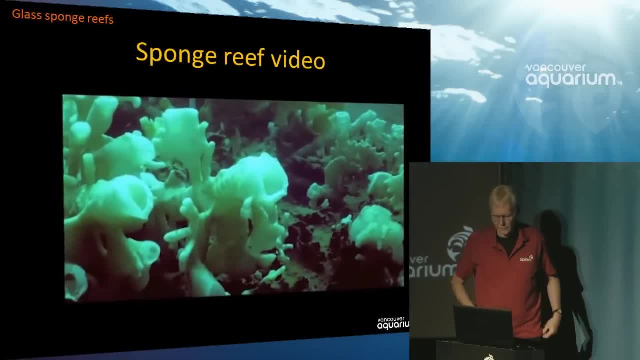 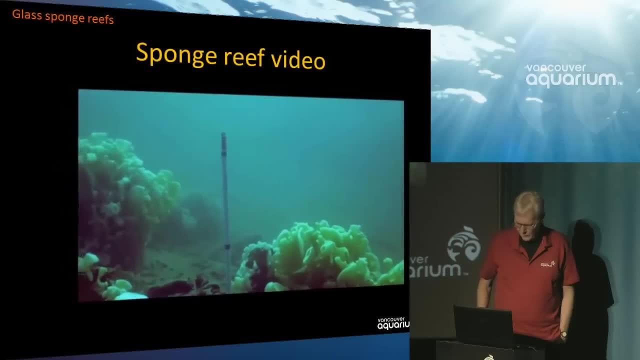 And then this is at the greatest depth, the greatest distance from the center of the reef, where there's one stripe on the stake with the full daylight. Without a video light you can't really see that the stripes are green, but when we're- 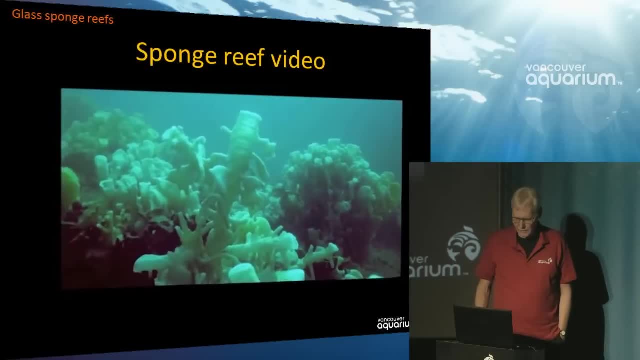 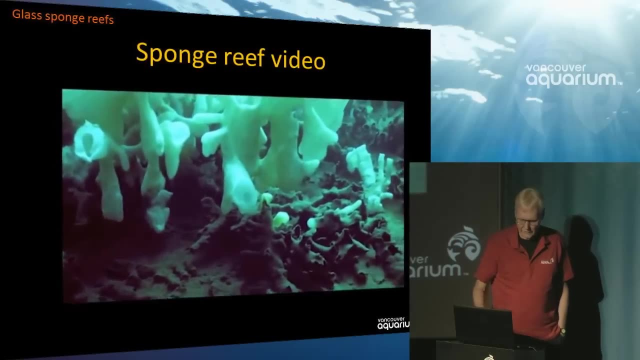